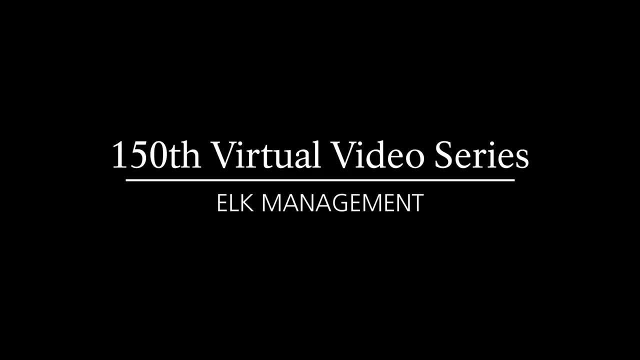 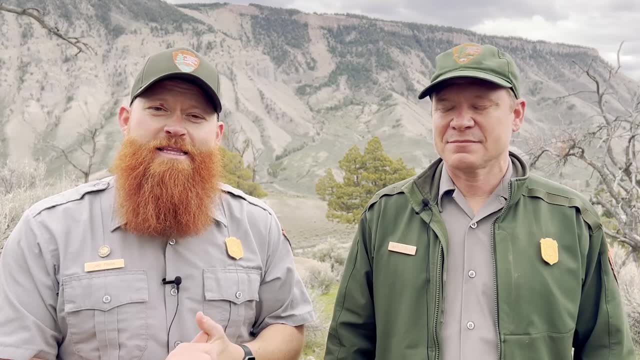 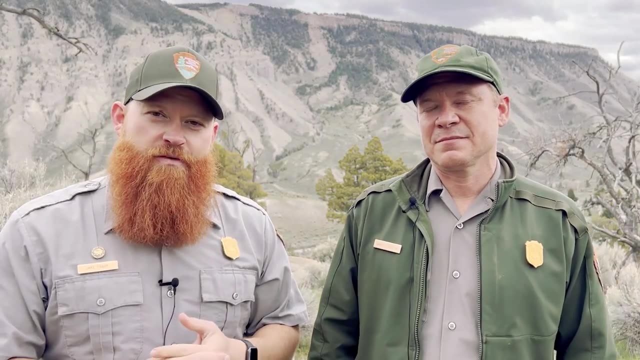 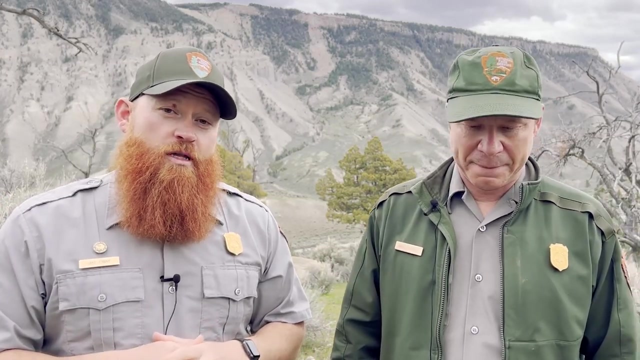 Good afternoon and welcome to Yellowstone. This is Ranger Jake. Today we're talking about the past, present and future of elk management in Yellowstone National Park as part of our 150th virtual video series. And to set the scene a little bit, we're here in the northern part of the park, which is where a lot of the wildlife watching occurs, especially a lot of elk and bison. 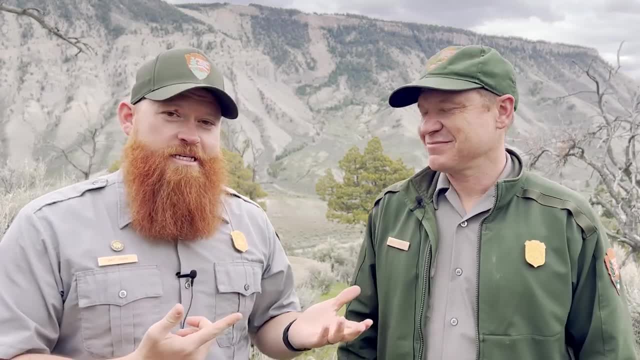 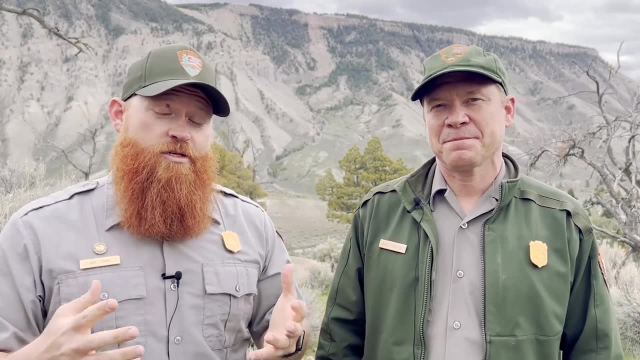 And today we're going to be joined. we are joined by Dan Stahler. He's a wildlife biologist here at the Yellowstone Center for Resources. I'm going to let him do a little bit more of an introduction about what he does, because he studies more than just elk. 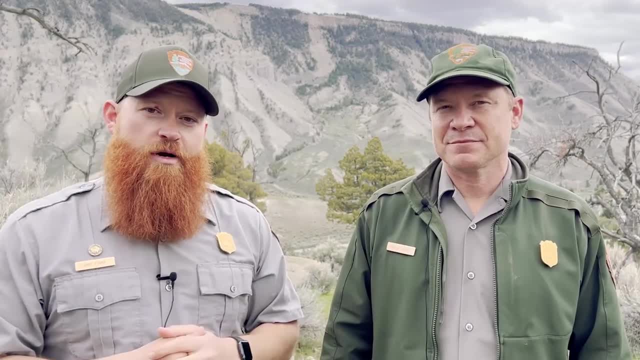 But it's been a very cool spring. You can see things are starting to green up. We have Mount Everett's over our shoulder. This morning there was a little bit of snow, but it's starting to melt off, So we're going to be doing a little bit of a walk around the park. 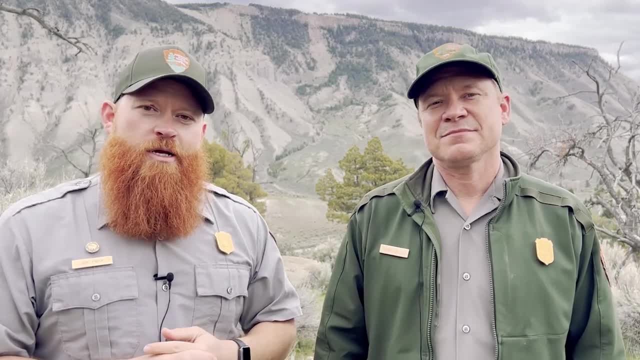 So we're going to be doing a little bit of a walk around the park, So hopefully, more warmer days that are coming along, But I want to thank you for joining us and I'm going to go ahead and jump behind the camera and let you take it away. 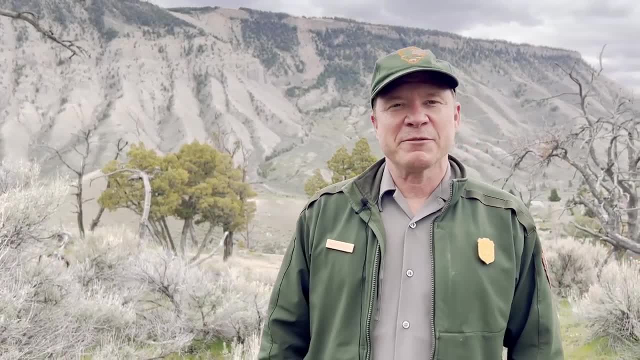 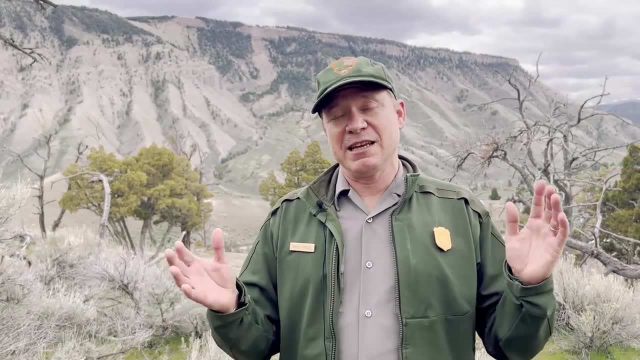 Thanks Dan, Thanks Jake, Welcome everyone. It's great to have you here. You can see, here we're just in a beautiful landscape And today I'm going to talk about the elk. It's really an icon of the West, an icon of Yellowstone National Park. 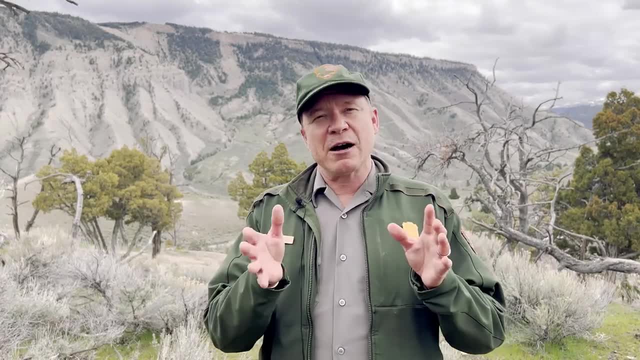 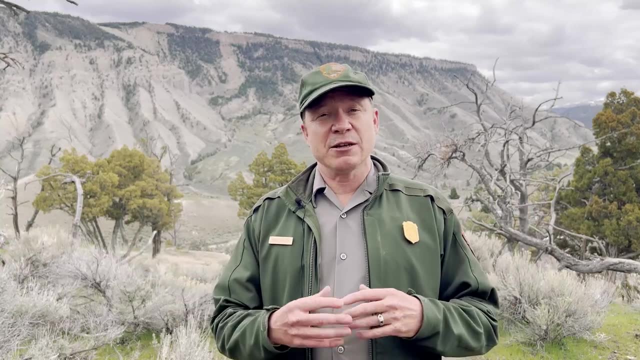 So I'm going to give you a little bit about their biology first, then talk about the history of elk in the Yellowstone National Park and surrounding areas. Well, first of all, just to remind everyone, Yellowstone National Park protects one of the most abundant and diverse wildlife communities. 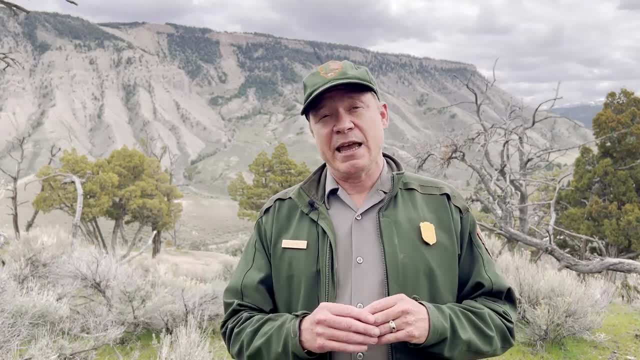 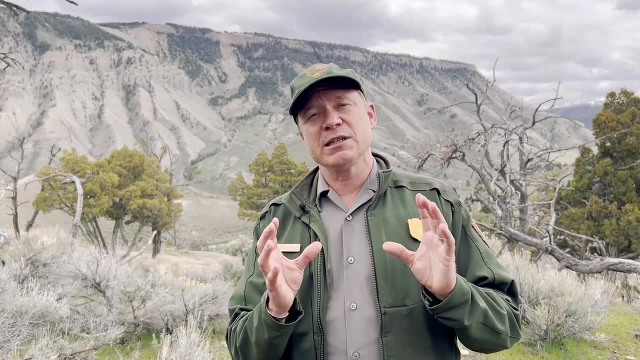 and one of the largest temperate ecosystems in the world, And much of the fate of wildlife, of course, has been controlled by humans through time. But if we just look at the story of the elk, it really is this wonderful tale of an animal that could have been lost. 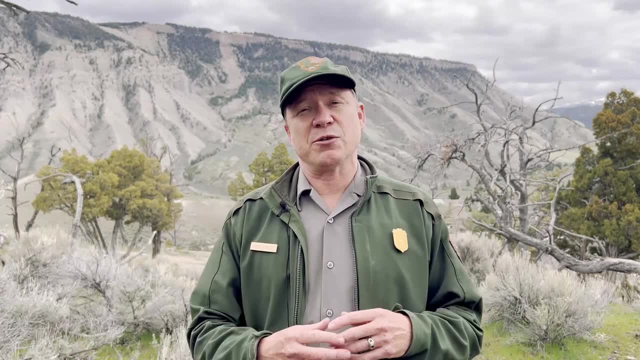 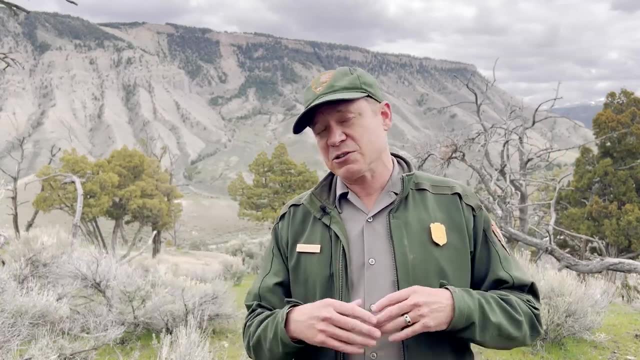 yet Yellowstone served to really protect it at the core of the greater Yellowstone ecosystem, And Yellowstone's elk really mean much more, not only for the park but beyond. They're on the borders of this national park and I'll talk a little bit about that in the history. 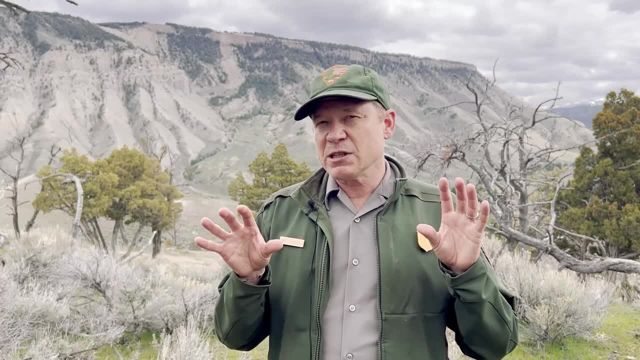 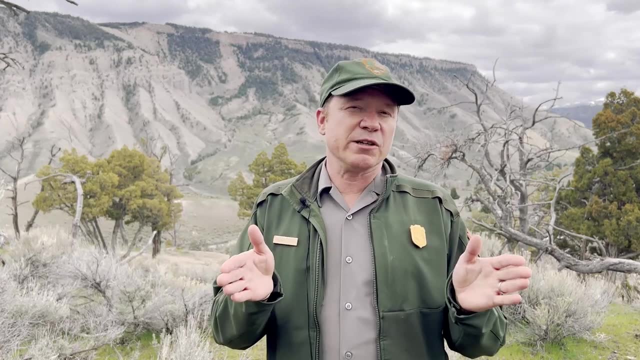 But let's start with a little bit of their biology first. This is a really poignant time of the year for elk. Right now we're getting towards the end of May, And this is the beginning of an elk's journey as an organism in Yellowstone National Park. 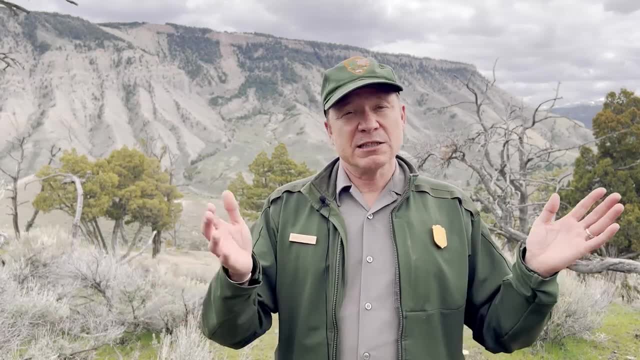 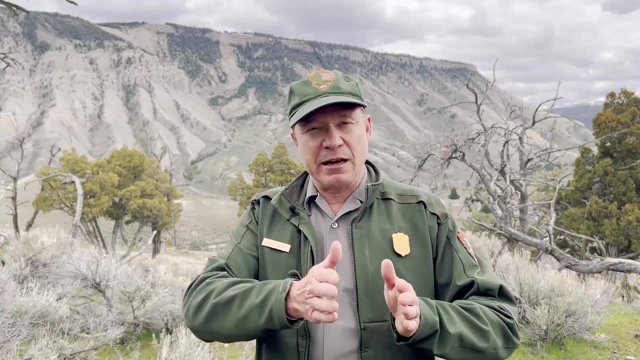 What we find with Yellowstone elk is calves are being born somewhere between mid-May and mid-June, with June, the first of June, kind of being a peak calving season, And so let's talk a little bit about the trajectory of an elk. 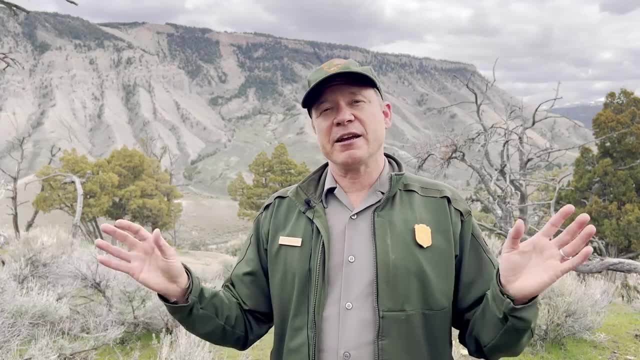 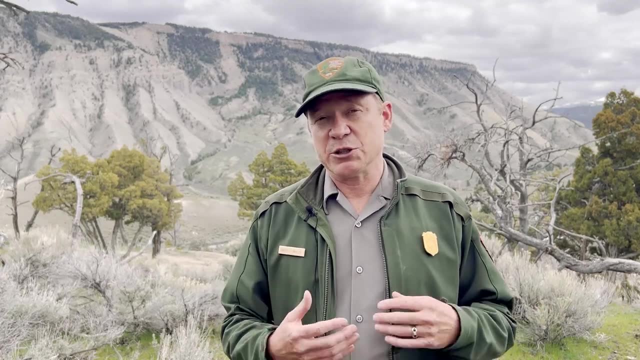 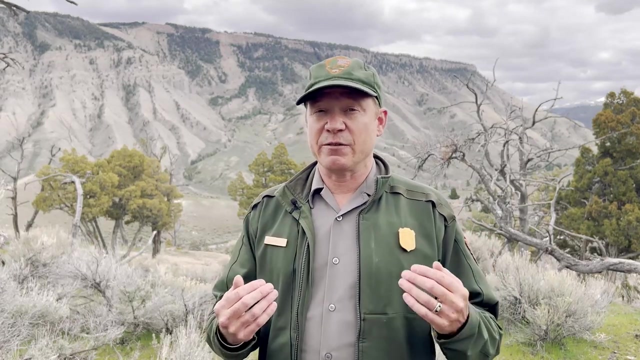 So right now, cow-elk are out there getting away from the herd of other cows and trying to select a very safe and secure spot to give birth to a newborn elk calf. And for the first several weeks of the elk calf's lives, very much its survival is dependent on getting enough milk from its mother. 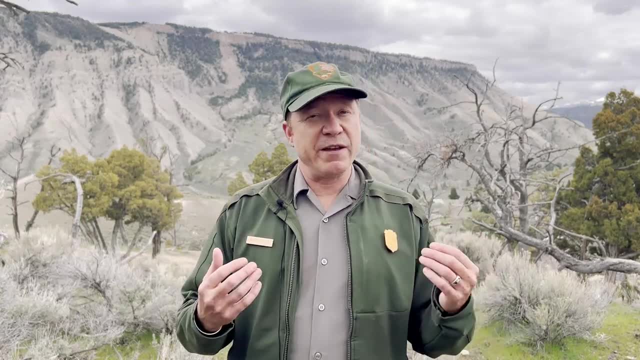 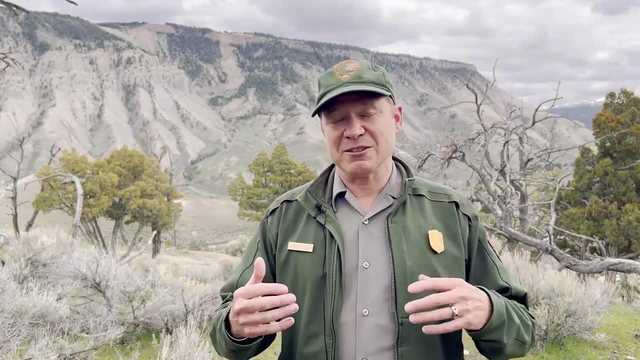 that really important nutrient supply, but also evading the risks of living in a landscape with predators, the effects of weather, You know. even though it's May, we're still, as Jake said, a little bit of a winter kind of lingering on. 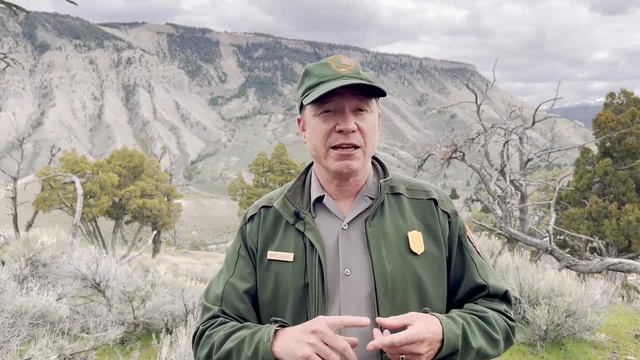 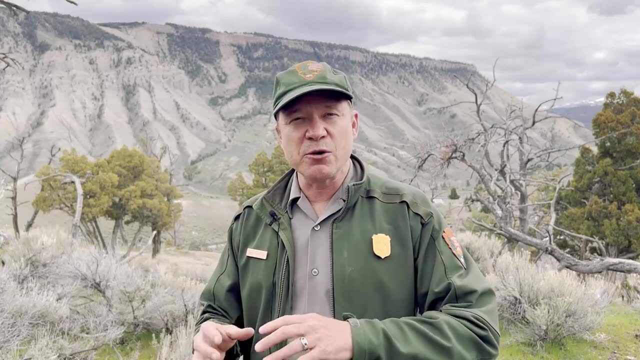 And so an elk calf's first couple of weeks really depend on security and food safety. And so they're hiding out and those mothers are coming and nursing them. Those calves are hiding on their own, They're spotted, they're relatively scent free. 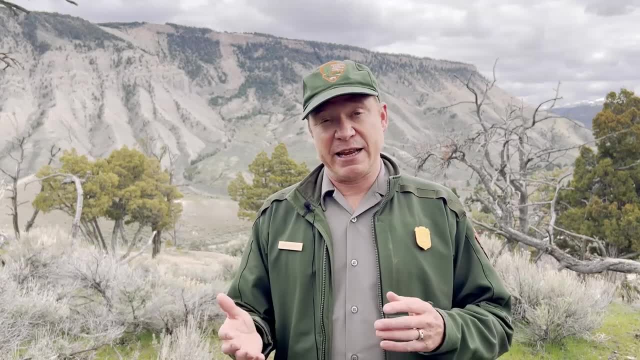 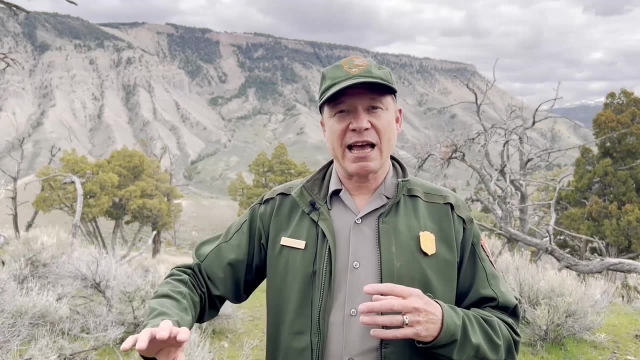 And these are all things to help protect them, evade predation and be safe. Those mothers will come call to them. They have a mother-calf bond and they nurse, And then those calves then go and hide again while mother goes off and grazes. 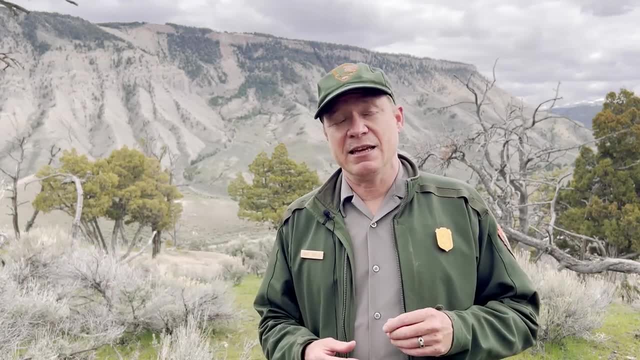 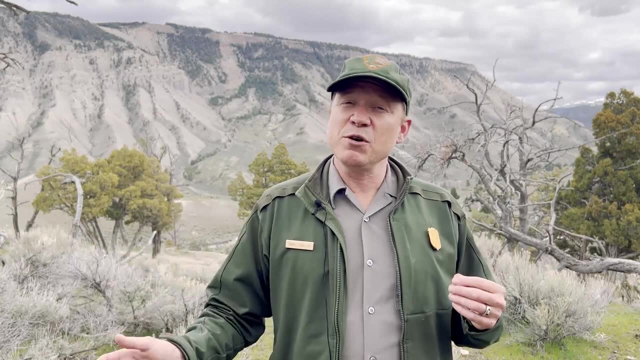 on these nutrient-rich green grasses that are coming up here in the May landscape. After several weeks those elk calves are up on their feet and can run and move quite adeptly with their mother, And eventually those mothers will gather up groups of calves. 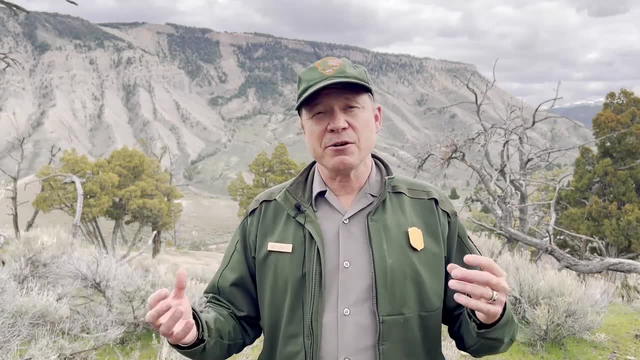 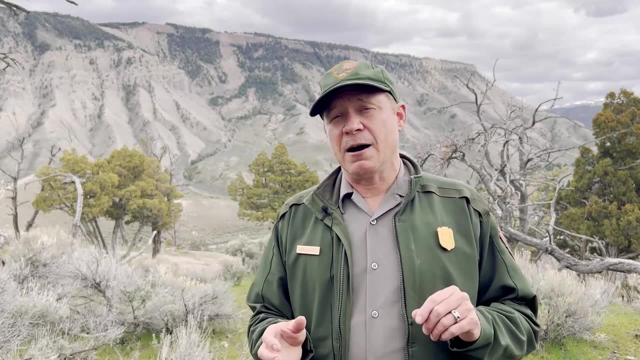 We call these nursery groups And that provides a little bit of safety. in number You get more adult cow elk to be vigilant, to look for predators. I'll talk a little bit about what predators are particularly important. And then, as the summer goes on, those calves are growing. 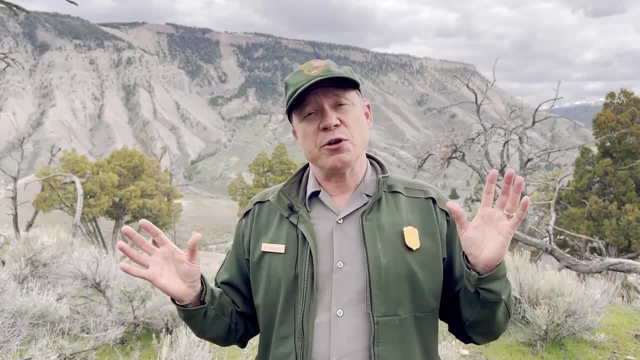 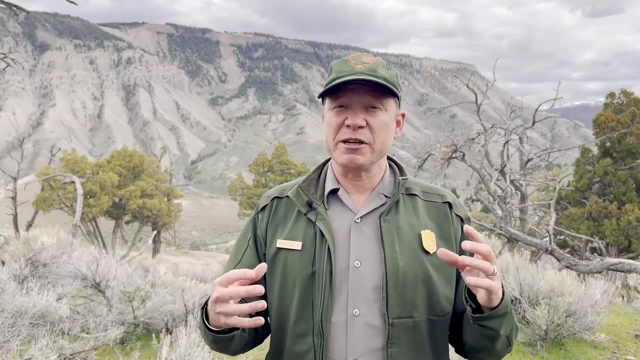 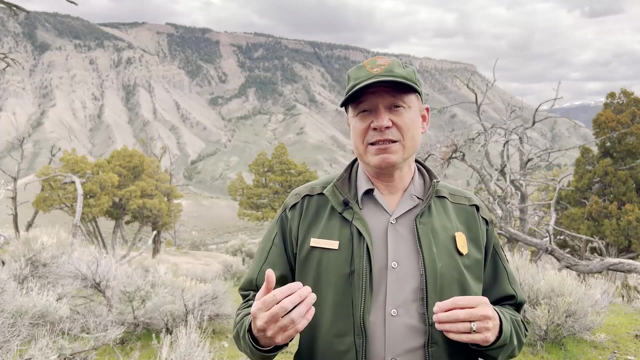 quite rapidly and by the fall those herds congregate up, Of course. then we get into the breeding season for elk, where the bull elk then come down and try to secure breeding opportunities by gathering up a harem of cow elk. Those males fight with one another to compete to be the one to be the most successful at breeding. 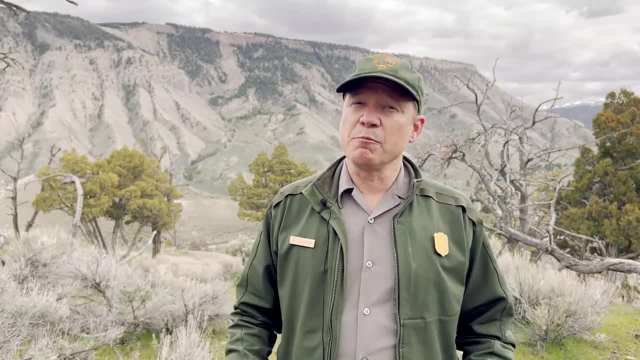 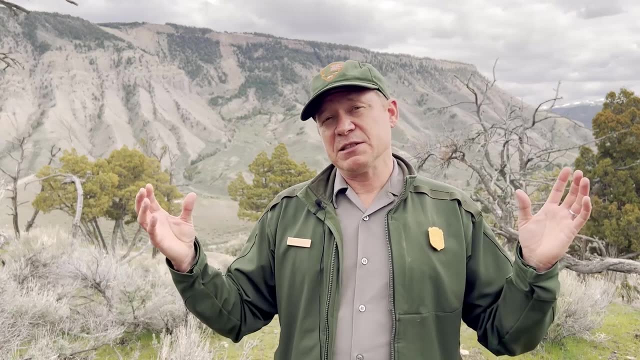 And those mature bull elk are the ones that are dominating the breeding. The young bull elk are sort of lingering off to the sidelines. The young of the year are still hanging out with their mothers And then, as the fall of the fall, event happens of snow coming October, November snows, then those elk go into their migratory. 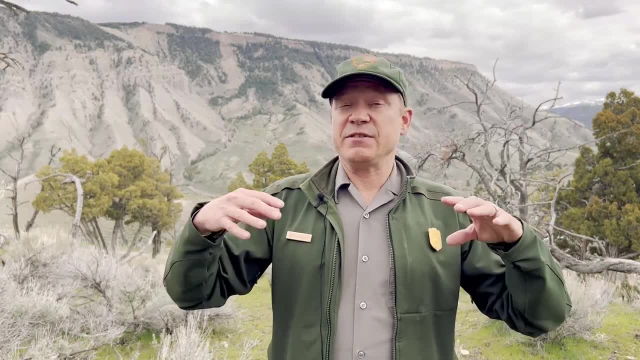 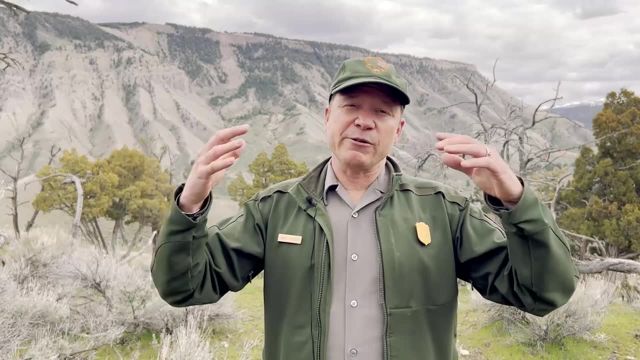 practices where they'll come out of the high elevation of Yellowstone and the surrounding areas where they've been feeding all fall and late summer on still nutrient green grasses, And then those elk migrate down for the winter time on what we call the winter range, the 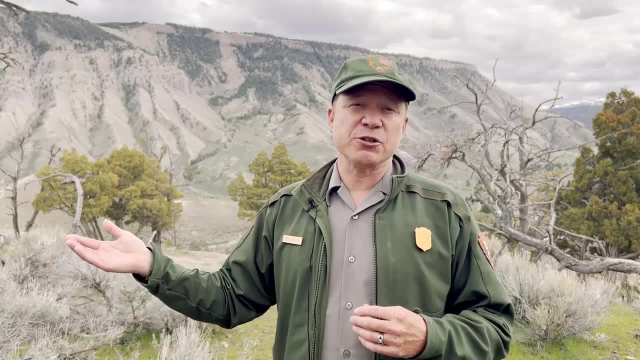 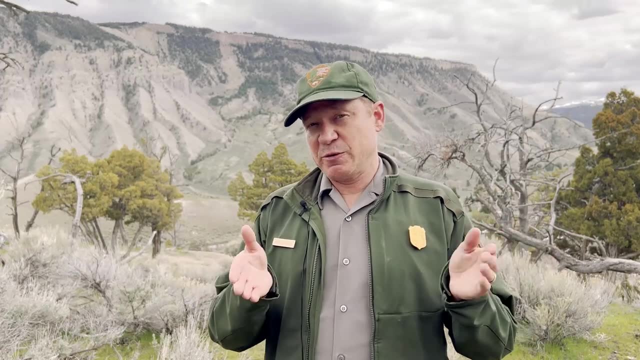 lower elevations. Here in northern Yellowstone, the northern range of the park that you're seeing behind us is key wintering range for elk and the other ungulates. And then ungulates, just to remind everyone, our hoofed animals. so bison, deer, pronghorn, elk, they all belong. 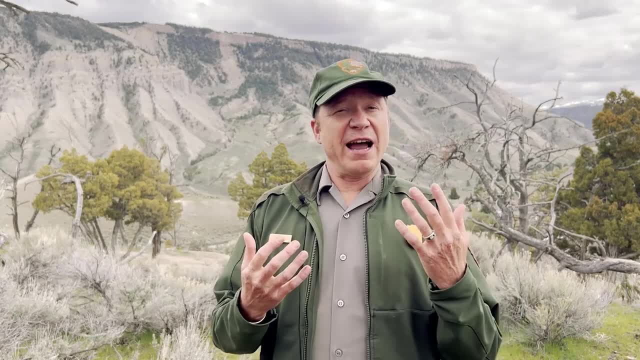 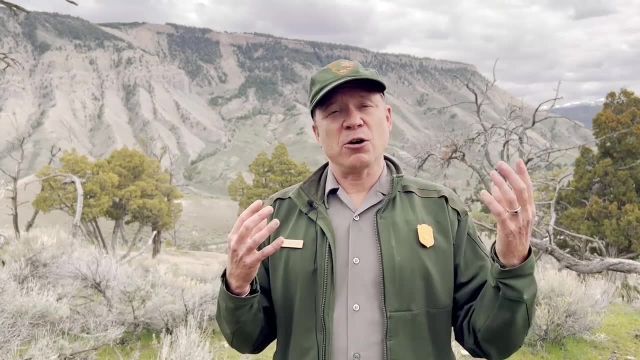 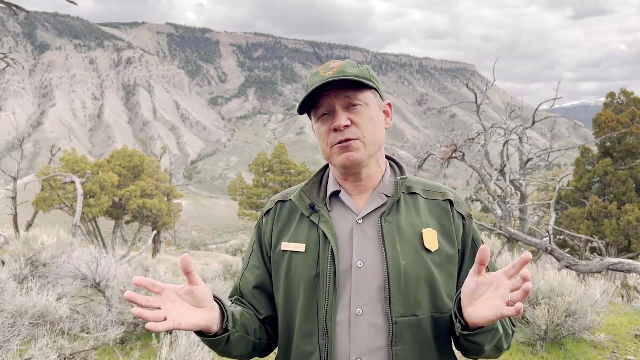 to the ungulate family. Of course, elk are one of five deer species here in Yellowstone National Park, and they're one of the largest ones, and they all share similar sort of nutrition and diet. They're feeding on grasses, sedges and forbs as part of their food throughout. 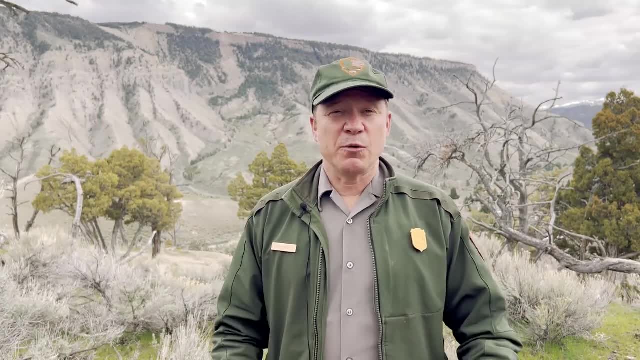 the year And they have a four-chambered stomach where they try to extract and chew their cud and extracts their food and they grow it. They have a very large stomach and they have And they have a four-chambered stomach where they try to extract and chew their cud and 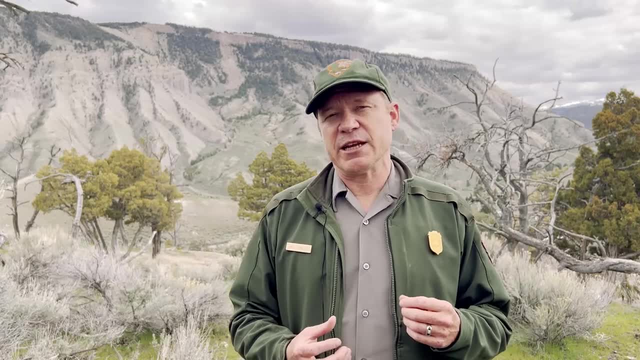 extracts their food and they grow it. They have a four-chambered stomach where they try to as much nutrient from those grasses and forbs and all the other vegetation that they feed on. in the late winter they'll sometimes feed on woody browse like aspen and cottonwood, and that's all. 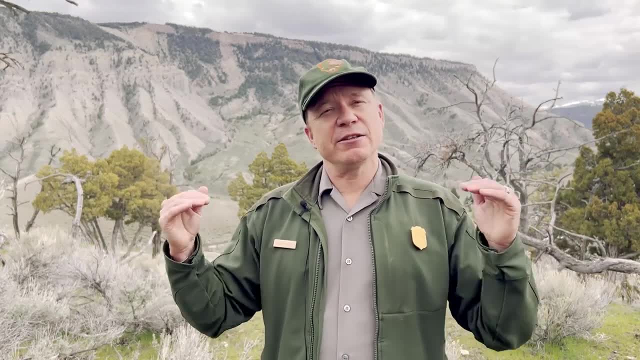 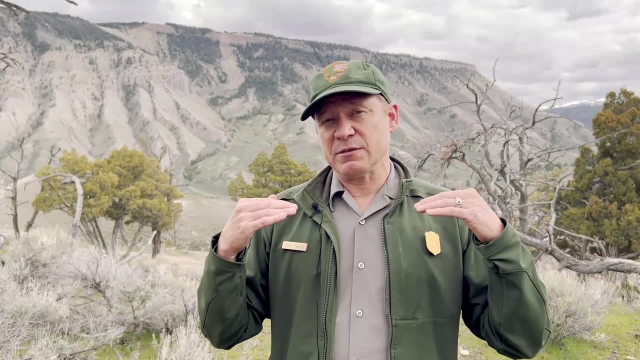 part of their diet. the elk are really adept and successful at tracking those feed food resources in space and time, and so once they're on the winter range, of course, they like to find places where there's relatively low snow. that helps them forage more efficiently and it helps protect them. 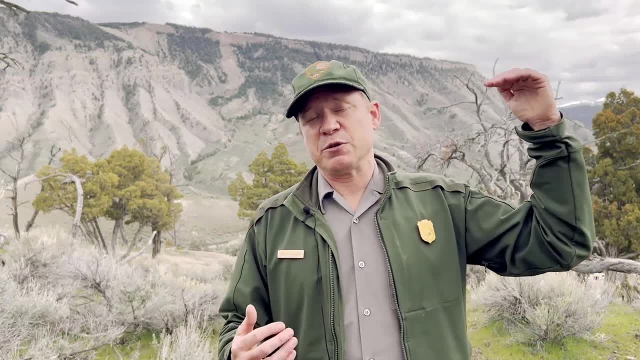 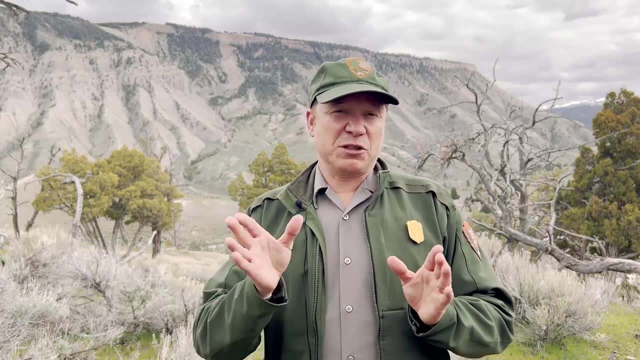 from the severities of winter that the interior high elevation of yellowstone presents to them. so that's why they migrate. and so if we think about a cow elk and and versus a bull elk, they have slightly different life histories. cow elk tend to live longer. usually a cow elk will start. reproducing by her second year and she'll be uh reproducing every year until she reaches her late, mid to late teens, and that's what we call reproductive senescence, where they no longer producing a calf every year. it's just the demands of of raising offspring can be difficult, as elk. 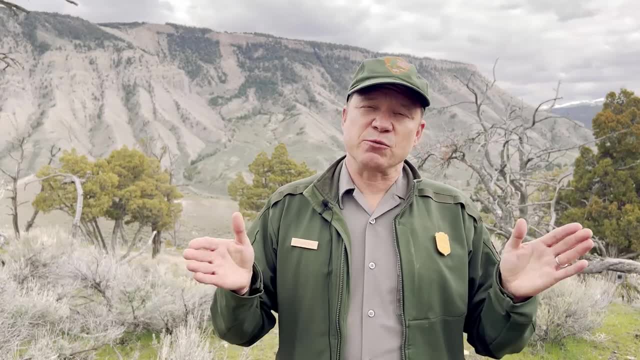 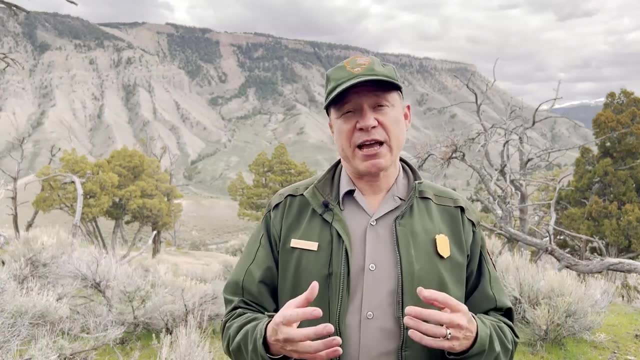 older in in their life, and so those prime age cows are really important to a herd's recruitment. they're producing calves every year. some of those calves will escape the gauntlet of predators and other challenges. others won't. but if enough calves make it through and survive to that reproductive 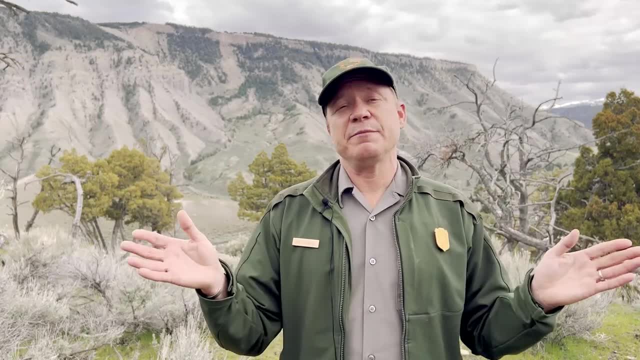 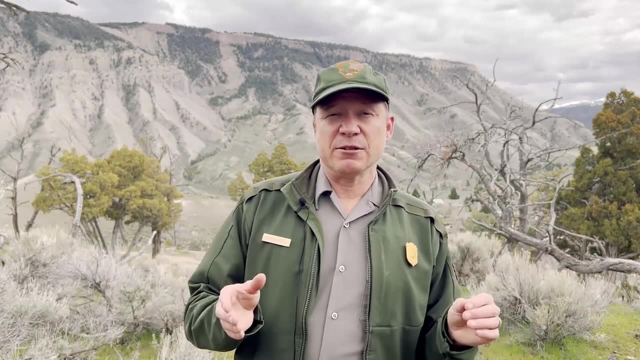 age they can experience a really successful life, for those prime years be ages between the ages of two and about 13 or 14.. they're relatively resilient to predation during those years, are very difficult to kill and so that we we find in yellowstone that you have high survival. 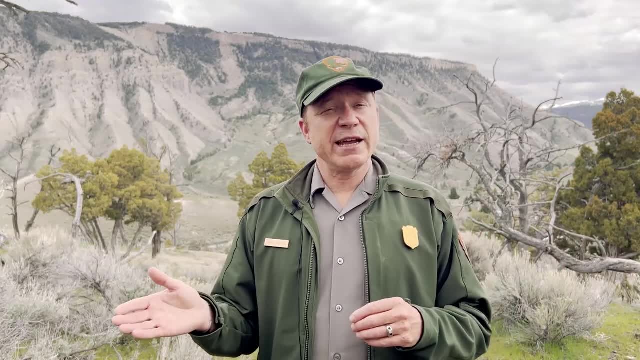 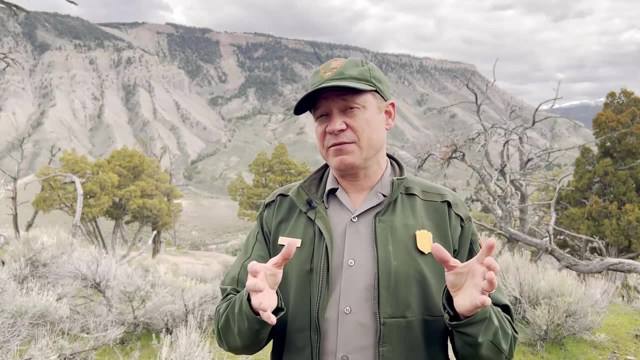 high pregnancy rates for those prime age cows, bull elk, on the other hand, tend to not live as long. it's a very difficult uh life that they face. they invest a lot of energy in the fall dedicated to the rut or the breeding season. they're bugling, they're fighting, they're chasing around cows. they're evading other bulls and they tend to go into the winter and poor shape because of that, so they can be more vulnerable to predation later in winter. and we find in general bull elk do not live quite as long as the results, averaging 10 to 12 years. 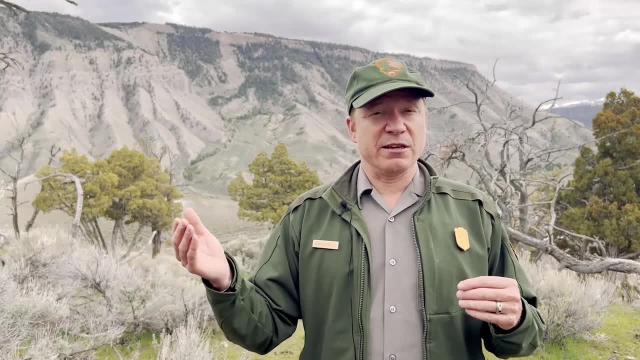 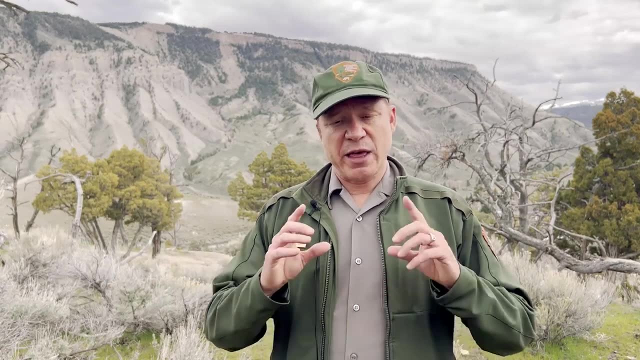 of age. we've had some cow elk here in yellowstone live to be over 25 years of age and we know that from some of our research on them and i'll talk about that here in a second. so that life history, that annual cycle of, of tracking resources from summer range to winter range, is really key to 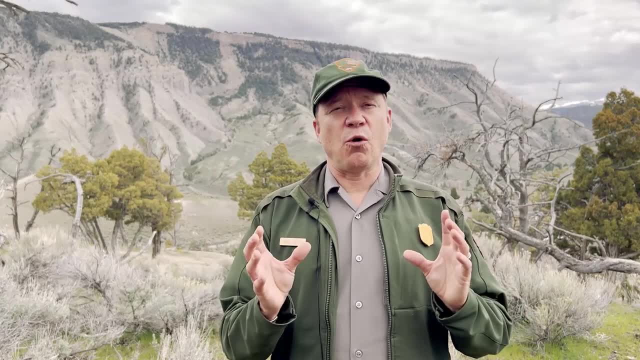 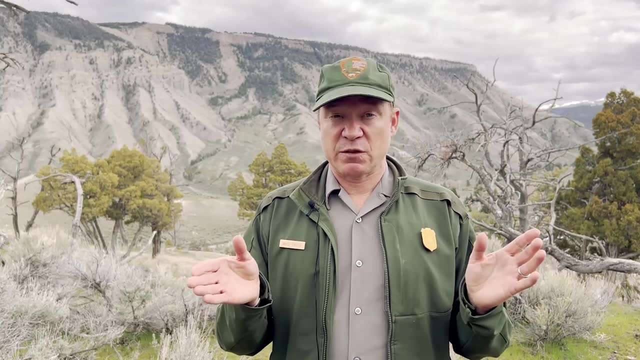 their success. when we look at yellowstone national park as a whole, we have about six or seven populations of elk, or herds that we call them- that use yellowstone. one of the most famous long-term studied elk herds in the world is the yellowstone national park. the yellowstone national park is a 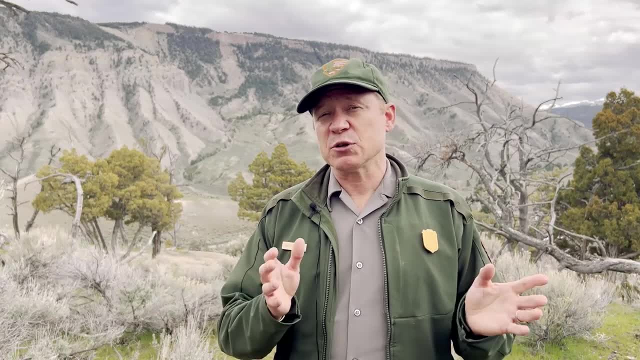 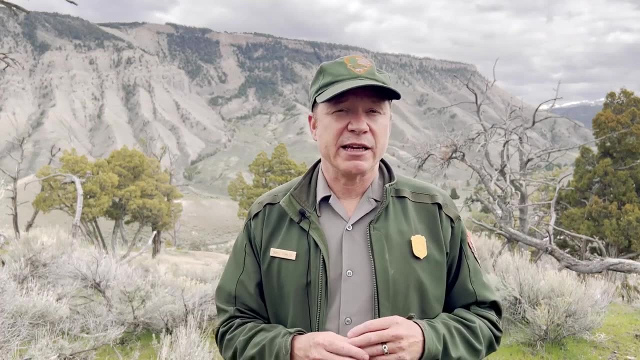 national park in the world is the northern range elk herd. today, that elk herd probably numbers somewhere around 8 000 animals, and it has been historically as high as over 25 000 animals, and those population trends have been dictated by human policies such as hunting, population control. 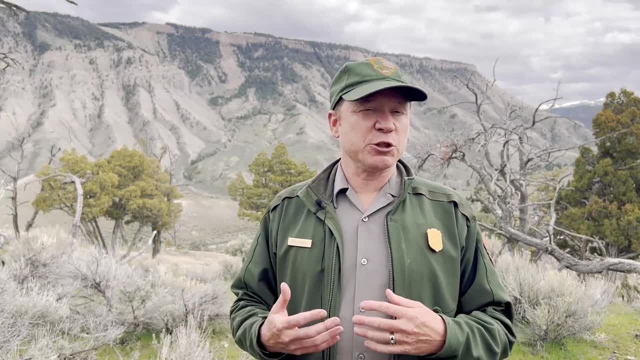 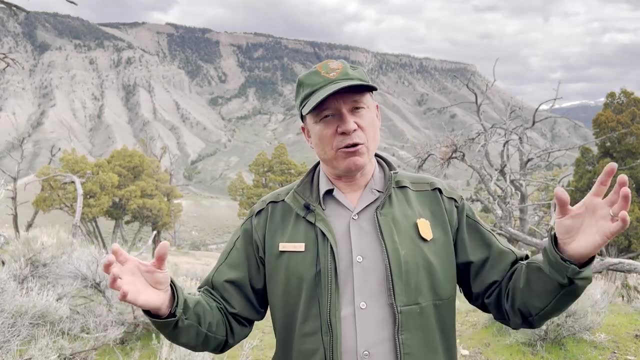 in the early years and, of course, in the last several decades. predators play a much more important story in that population regulation of elk. there are other herds that also use yellowstone and what happens is elk are migrating into the park this time of the year, right now. 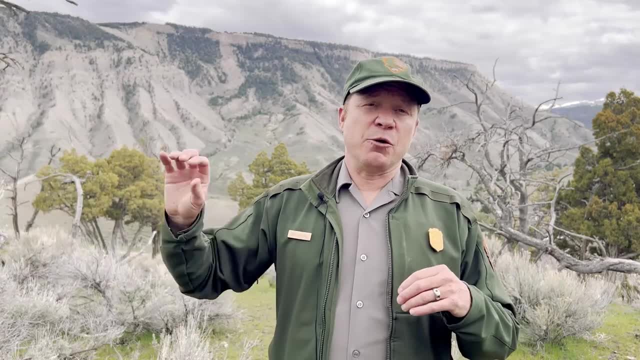 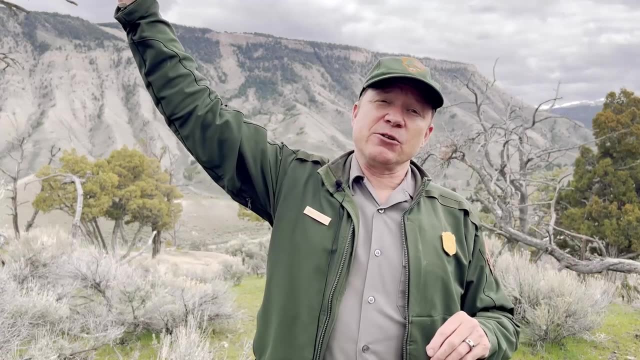 elk from herds: uh out by cody wyoming. uh, the wiggins fork herd, the jackson herd. you've got elk from the madison valley to the west of the park, the paradise valley herd to the north of the park, all coming into yellowstone because it offers such really wonderful summer range habitat for. 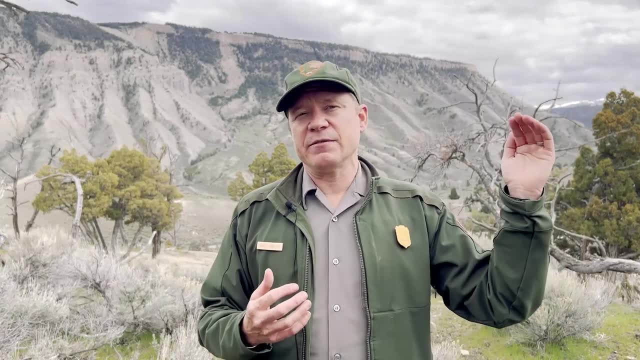 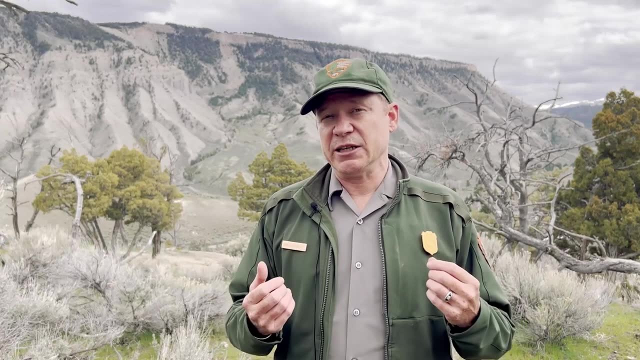 them nutrient rich grasslands all the way up into the high elevations of the mountains, and that really is a key to their success. so that kind of is a brief summary of elk biology. now, part of what we do as biologists to learn about this is we can really just take a look at how elk are doing in the 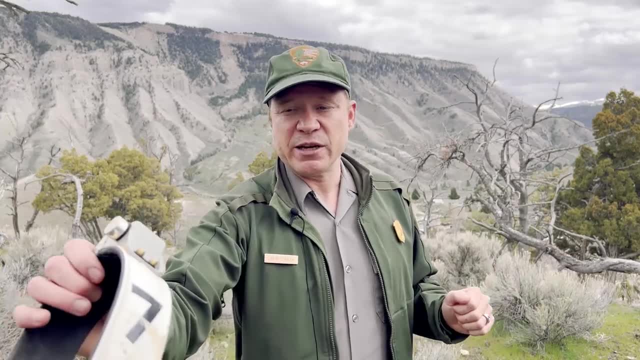 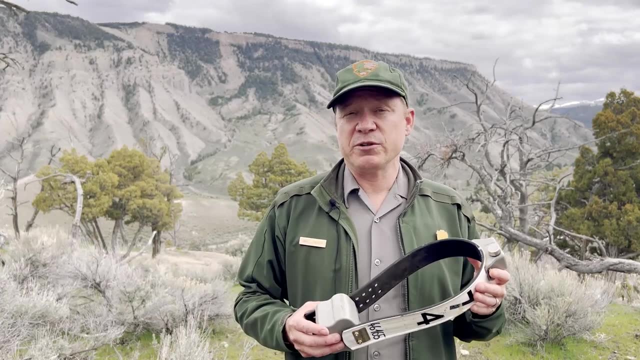 study them with the advancements in GPS collar technology. So here, for example, is a GPS collar that we would put on a cow elk. Each winter we capture elk here in northern Yellowstone and anywhere between a dozen and 20 elk each winter in recent years. we'll put on a GPS collar. 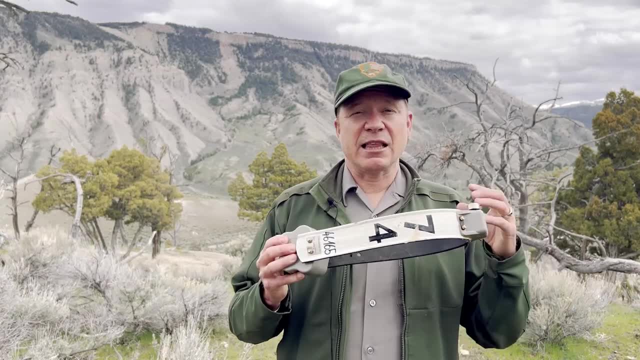 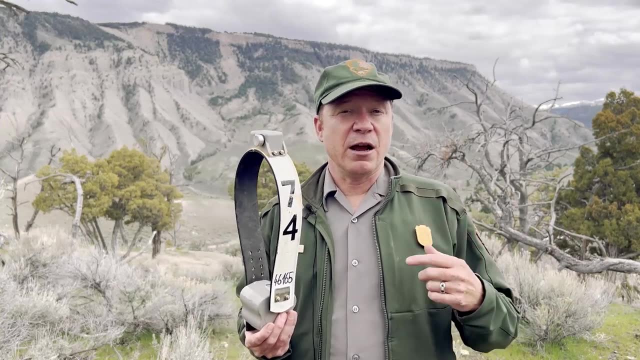 This collar gets a point once an hour around the clock, and these last for about four to five years, and this provides a really wonderful opportunity to study not only how elk survive when they die. what is the cause of death? Was it a wolf, Was it a cougar? Was it a human hunter? just? 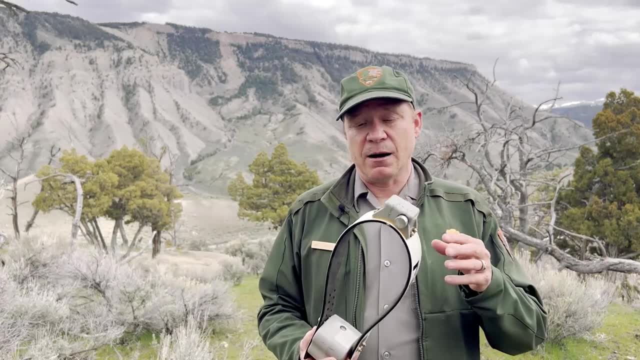 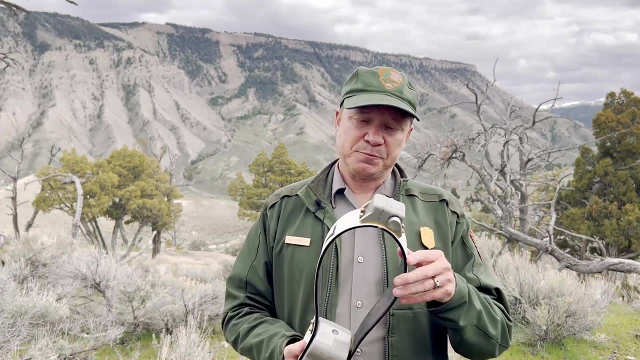 outside the park. Did it die because of winter severity? These are all the pieces of information that we, as biologists, can gather by putting these GPS collars out. What are the parts that are on that? Yeah, so this is the battery and this hangs below the elk's neck and this is a power source. 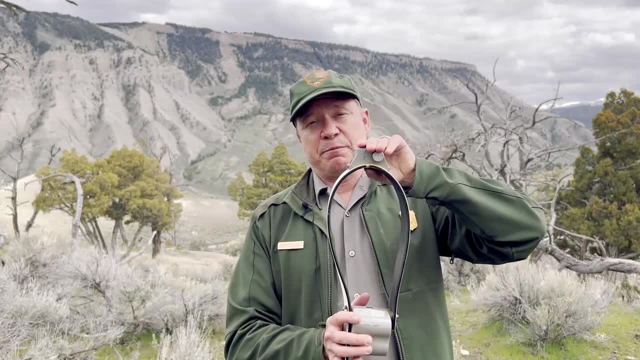 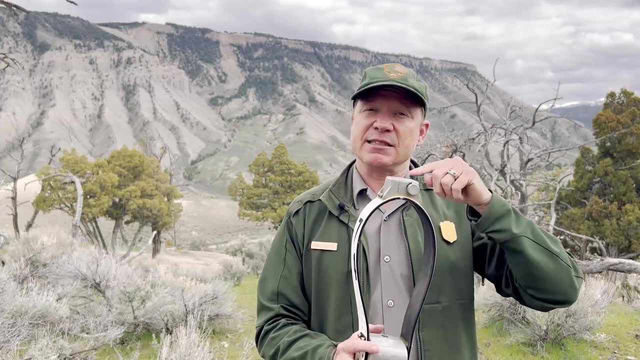 4d batteries that allows it to power the collar. This compartment of the collar at the top is the GPS transmitter, which communicates with the satellites to get a location fix and then that sends it to a different computer server that we can access the data from. 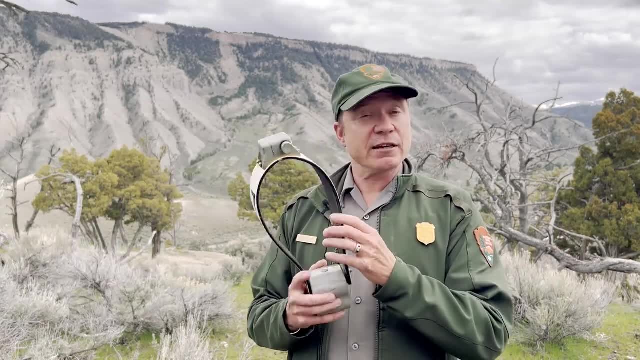 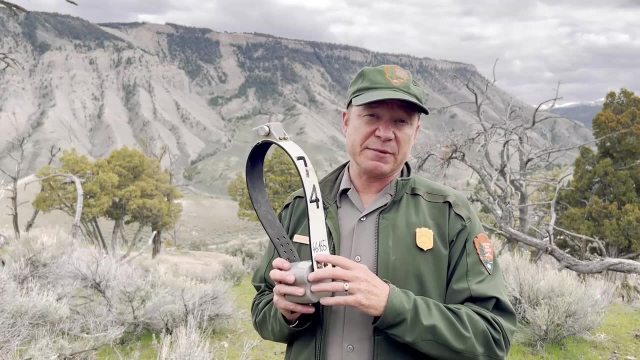 We put numbers on the sides of the collar in case we want to identify unique individuals from a distance. For example, up and coming, the next couple weeks we're going to be following around some of our cow elk to determine if they've had a calf or not, and we can use these. 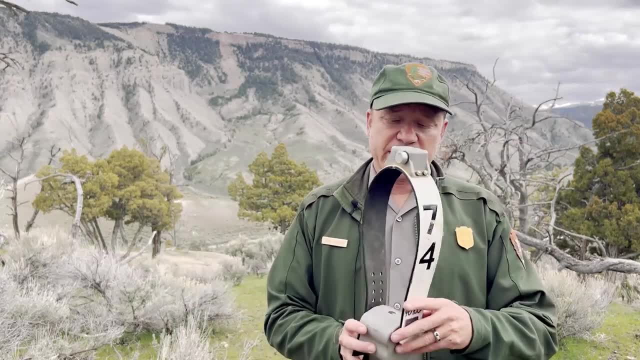 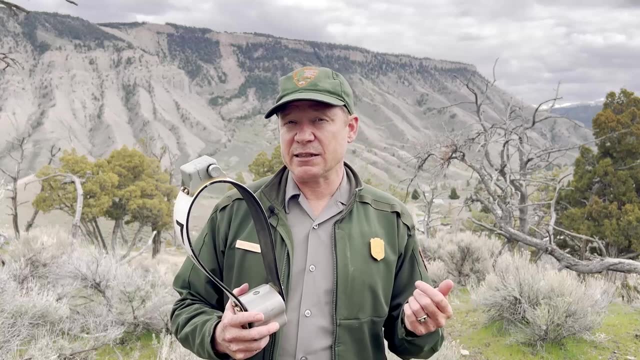 IDs to recognize an individual off in the distance, and so that's what the numbers are for. When we capture elk, we collect blood from them for genetics and disease. We can measure pregnancy at the time of capture. All of this fits together in our understanding of elk here. 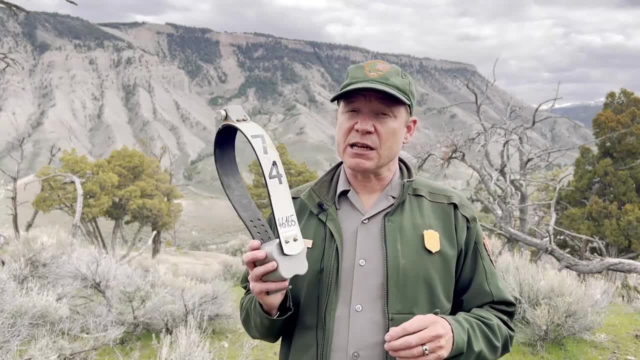 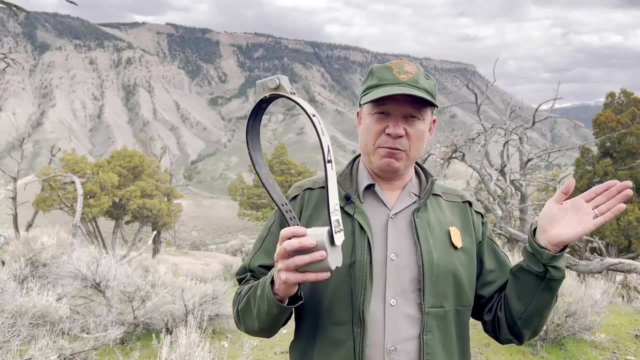 and our long-term studies on elk population. From this, for example, we've learned, as I mentioned earlier, that prime age cows have very high survival. About 90 percent of cows are living from one year to the next between the ages of two and about 13.. After that, survival goes down. For example, the average age of a wolf-killed cow elk is about 14.. Prime age cows are again not selected by wolves. They're too difficult to kill for them in most situations. but of course, a cow elk's calf this time of the year, the newborn elk calf. 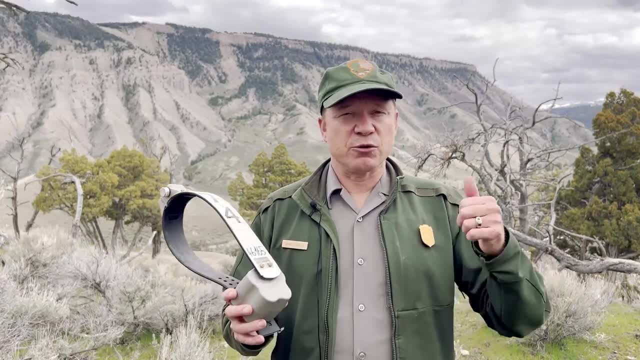 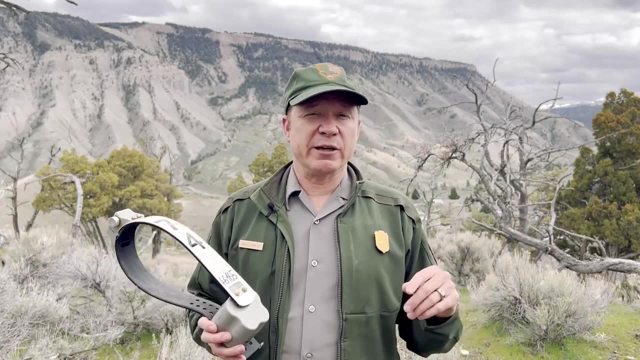 is very much the focus of predators. So right now there's grizzly bears, black bears, wolves, coyotes, cougars, even golden eagles, which will take advantage of newborn elk calves out there, and that's part of the strategy of a calf hiding out, being spotted, blending in with its 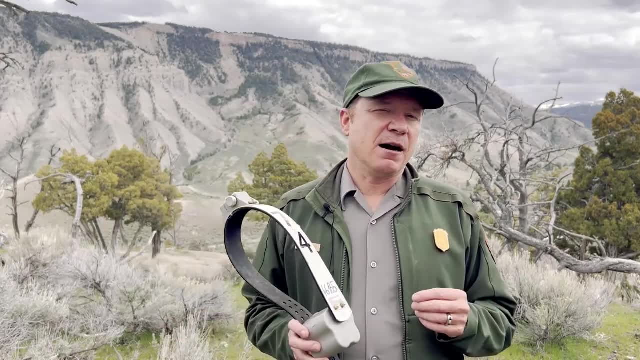 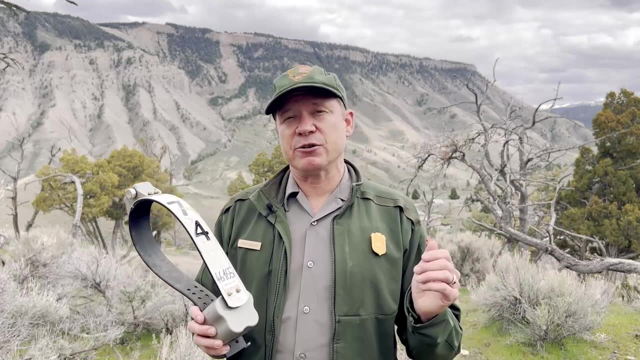 surroundings, hiding until mother calls to it to nurse it. So those first couple weeks are really key. Really the first month of an elk calf's life is full of challenges And if they can make it through that predator gauntlet they have a higher chance of surviving. 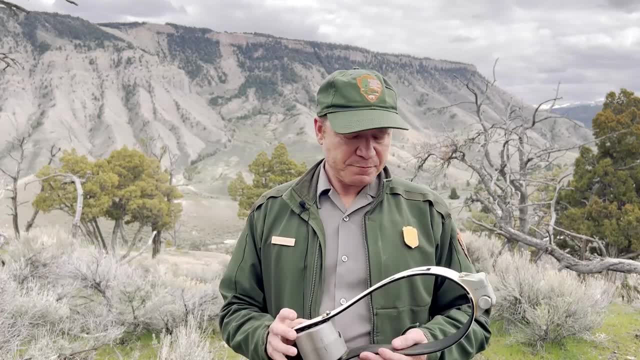 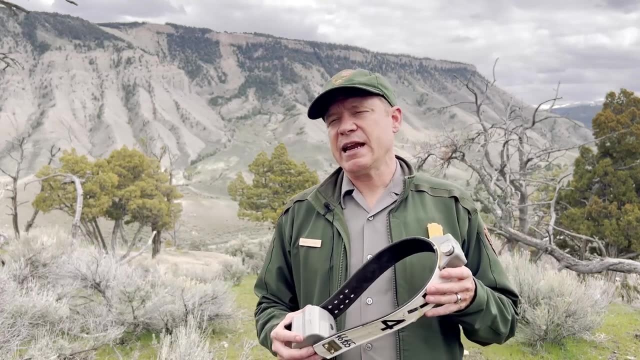 until adult age. Yes, Jake, What's the amount of elk that you're trying to have collared? Is there like a specific target number that gives you the amount of information that you like? Great question. Right now we have probably roughly 50 to 55 GPS collared cow elk in the northern herd. 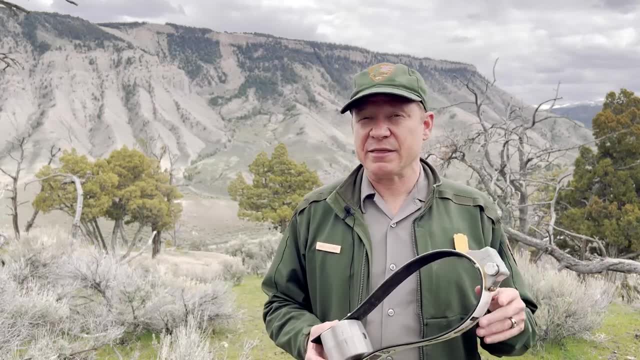 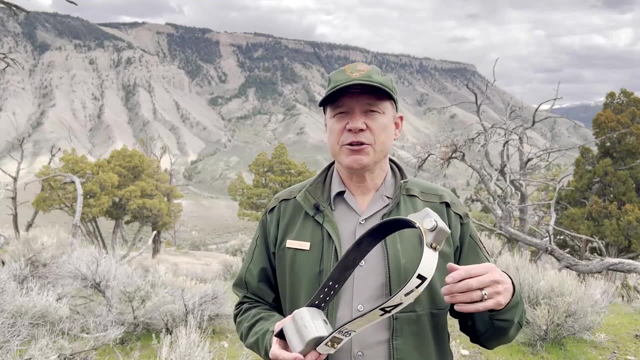 and that's out of about a herd of, about herd size of, you know, approximately 8,000 elk give or take. You know counting is imprecise but that's a kind of a ballpark And that gives us a really good if we can maintain, you know, 50 or more collars on our. 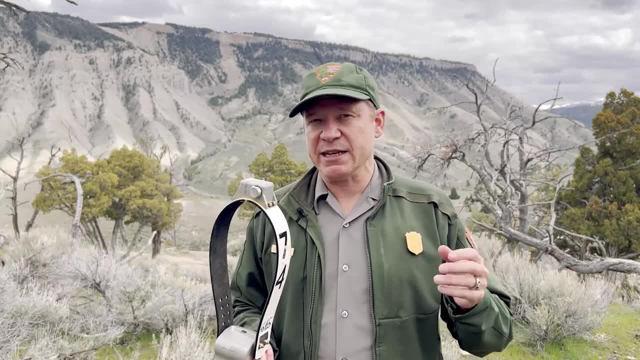 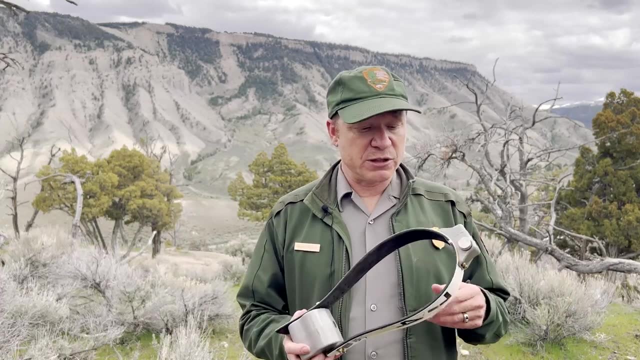 population. that gives us a good idea to track what we call vital rates, Survival, birth rates, recruitment into the herd, habitat selection. We also use these GPS collars in conjunction with the GPS collars we put on wolves and cougars, which is another of the other animals that I study here. 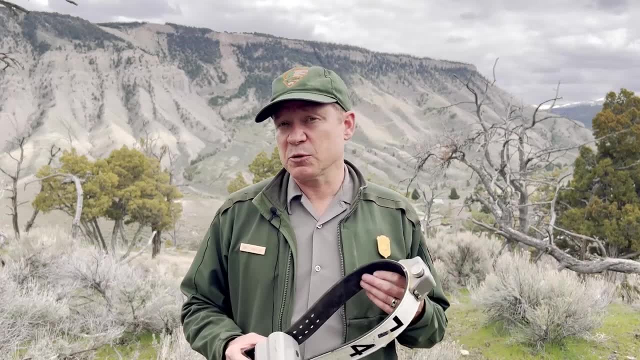 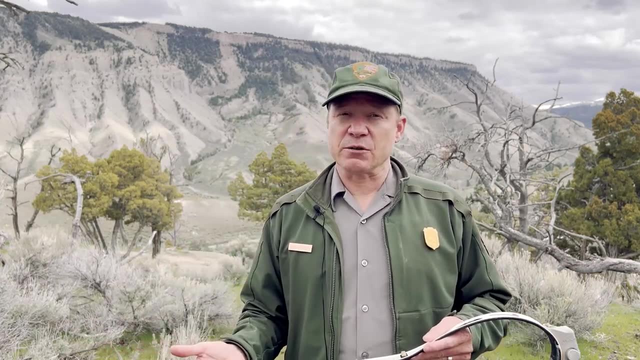 to understand how elk can avoid predation risk and what makes them vulnerable to predation. Bull elk can be, for example, more vulnerable in late winter, as I mentioned before, because they've exhausted their fat reserves. In the fall, they can be more resilient to predation. They've 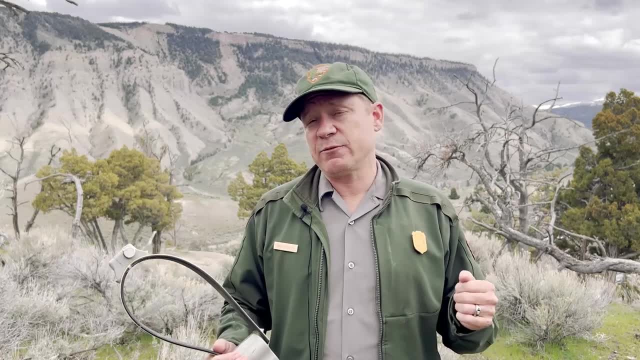 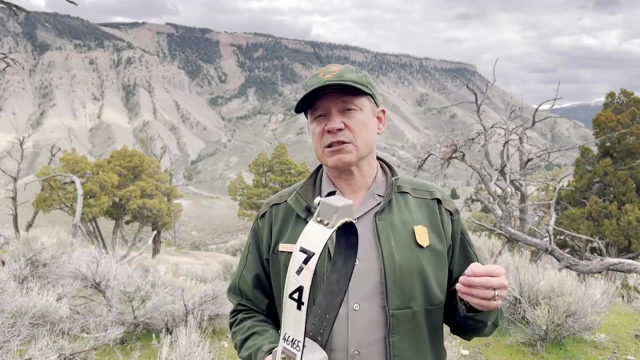 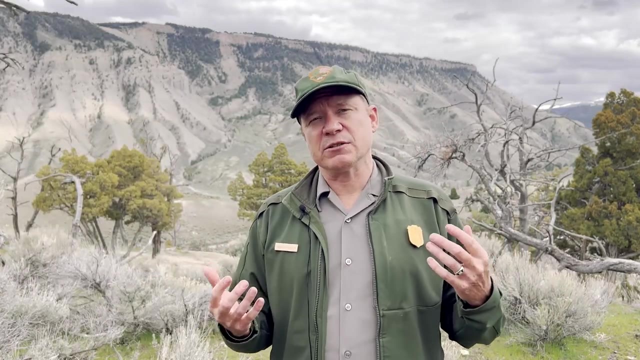 got antlers. If they stay in their ground and there's not deep snow, they can fight off wolves, particularly the prime age bull elk, And so all of that feeds into our understanding of what the risks are for elk on the landscape. So, as I mentioned, in terms of what the importance of elk to Yellowstone, we can think of them in. 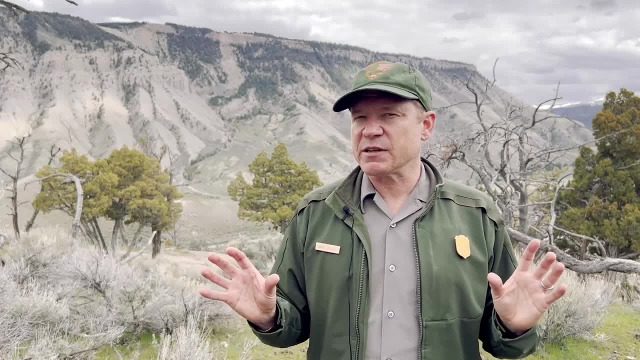 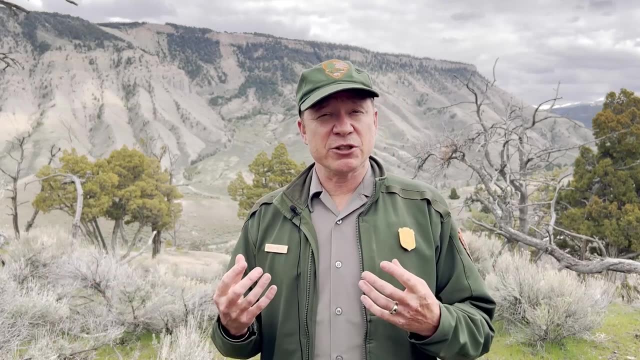 some ways as a keystone species. Now, some of the traditional definition of a keystone species would be an animal that's in relatively low abundance but has a disproportionately large effect on how an ecosystem functions. Elk aren't quite fit that proper definition or that original definition. 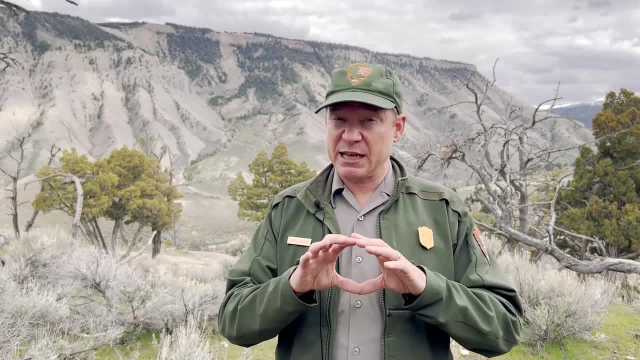 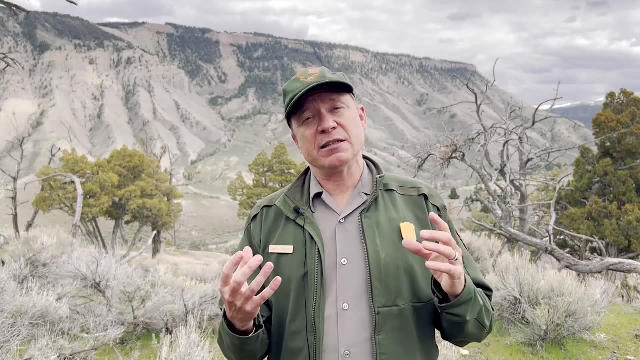 of a keystone species. but if you think of a keystone species as of an animal that plays a key role in how an ecosystem functions, regardless of its abundance, elk fit that title very well, And that is because they are incredibly important to how food web dynamics are structured in the 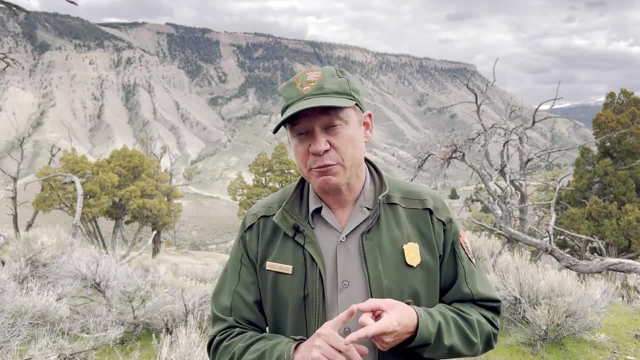 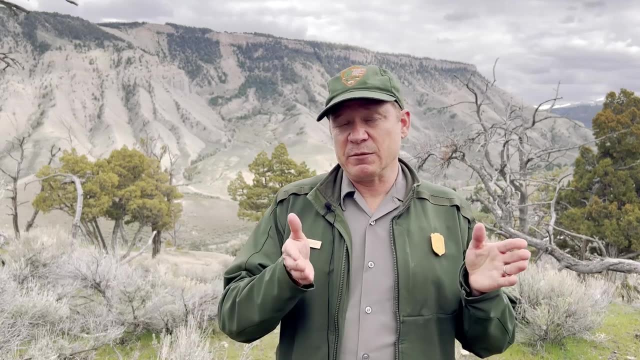 Yellowstone landscape. As I mentioned, they are the one of the primary primary prey species for Yellowstone's top predators, the wolves and the cougars, And, as part of the research that we conduct here on predation predator prey dynamics, we are really interested in what are the impacts? 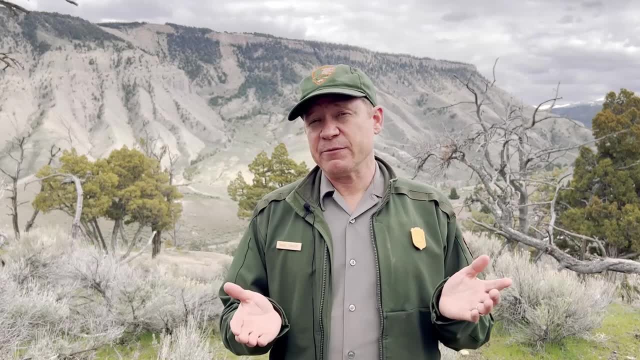 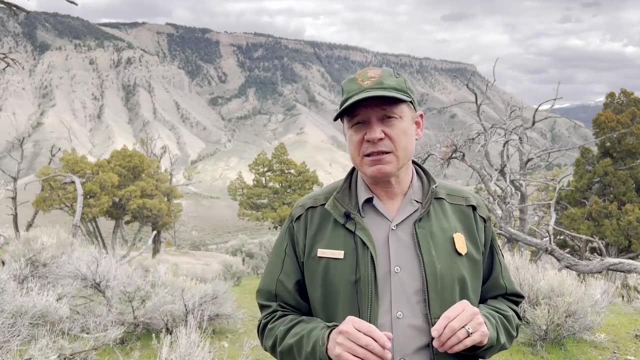 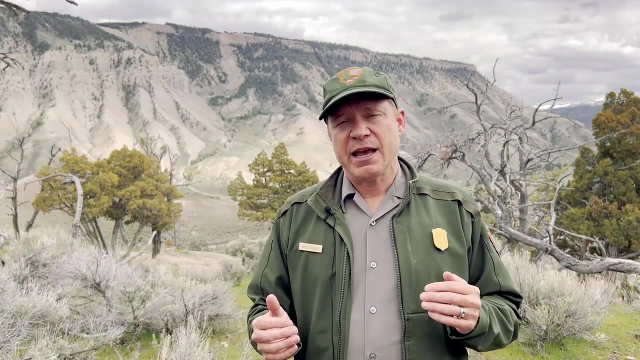 of wolves on their prey, such as elk, Elk, make up, for example, 90 percent of a wolf's diet through much of the year. For cougars it's more like 60 percent of their diet these days, sometimes 55. they're starting to use more deer in Yellowstone than they used to, you know, 20 years ago, And so. 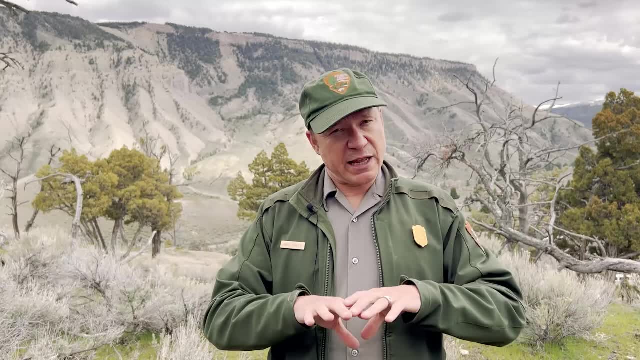 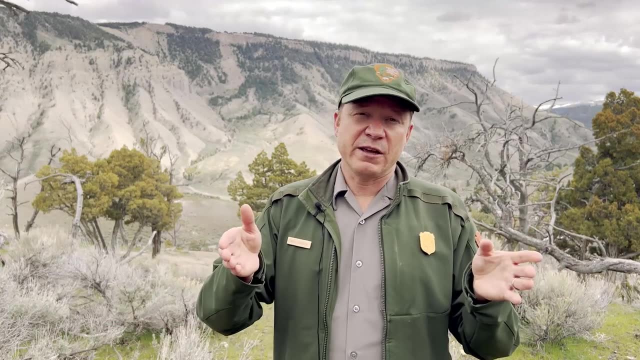 when you have a wolf pack, that's feeding predators and predation, which is a powerful ecological force that can shape ecosystem food webs, because of that top-down pressure essentially causes nutrients to ripple through the ecosystem. So when a wolf kills, a wolf pack kills an elk, or a cougar kills an elk. 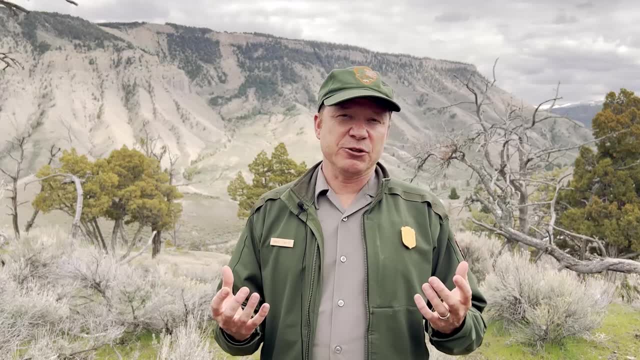 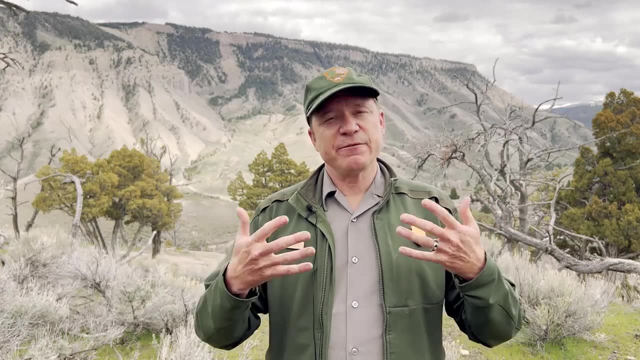 they feed on that themselves and then a lot of that meat, that biomass, can go to the scavenger communities, the ravens, the magpies, the golden eagles, the bald eagles, the bears, all which depend on that food resource. And when you have food webs that are more complex and more connections out, 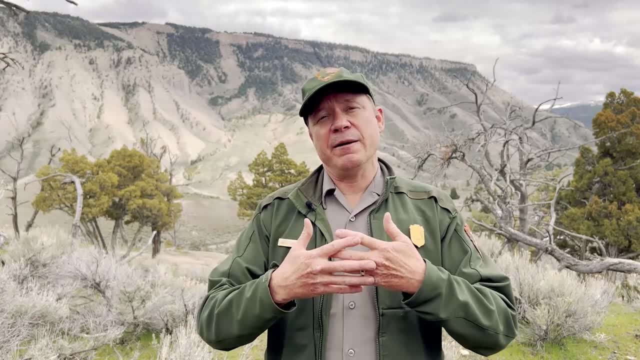 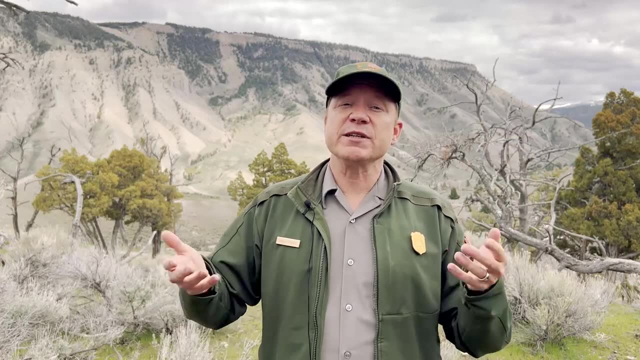 to environmental changes and so elk are very much at the core of that- Then if you look at the role that elk play as grazers- they graze grasses and forbs and sedges and that is really important for nutrient cycling in that component of the food web. So every time they're eating grasses and and 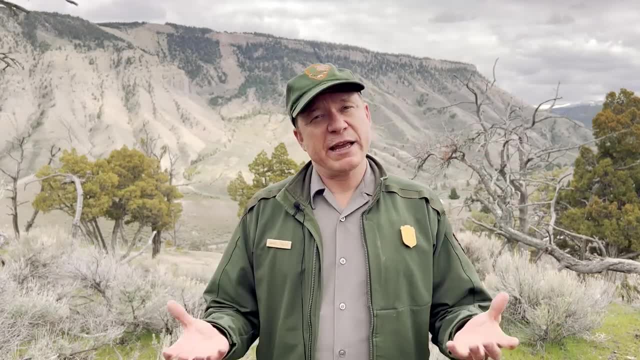 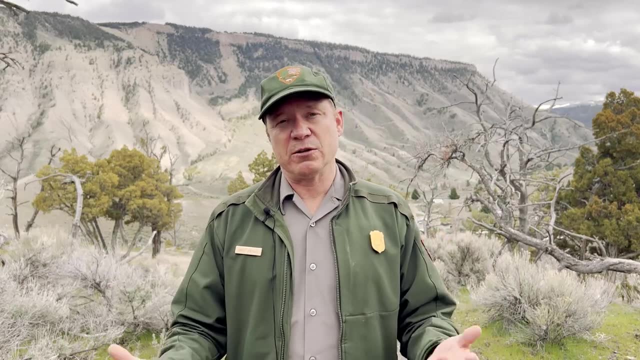 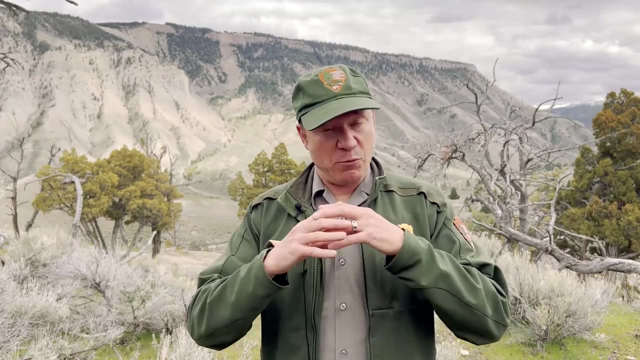 stirring up the dirt and the soil and grazing those. that creates more plant productivity. it helps with soil retention, moisture retention, it can help with that nutrient cycling through the lower parts of the soil communities that are important for regenerating plant growth. And and, of course, when elk defecate or urinate, they're spreading more of those nutrients back onto the landscape. 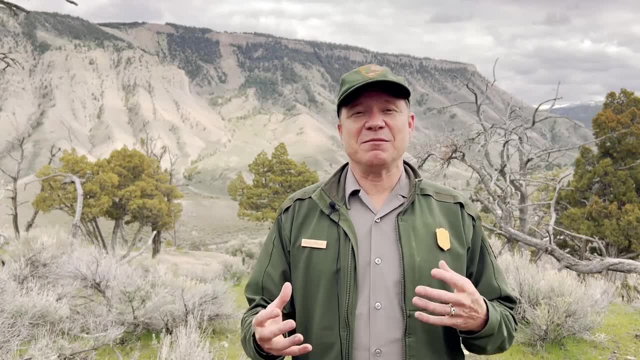 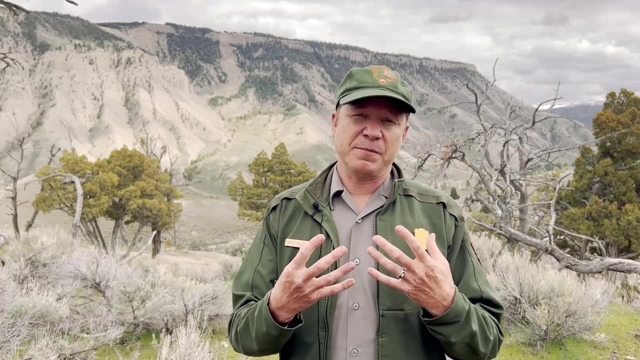 and then then that even feeds into a whole host of bacteria and microbes that live in the soil. So elk are very much at the core of that Yellowstone's really rich and complex food web system, And that that only isn't for the park, but elk rippling out through One of the things we've. 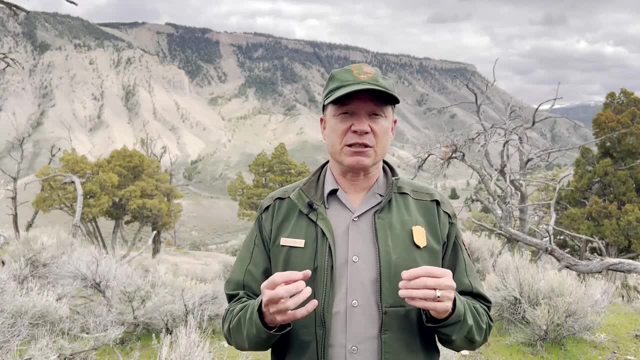 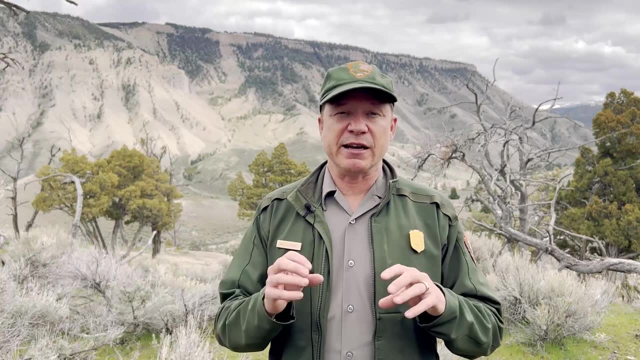 learned about elk movement from studying with GPS collars is not only is Yellowstone National Park at the core of really important uh ranges for multiple elk populations, but it's also important to remember that there are multiple elk herds that use this area, but so too are the lands. 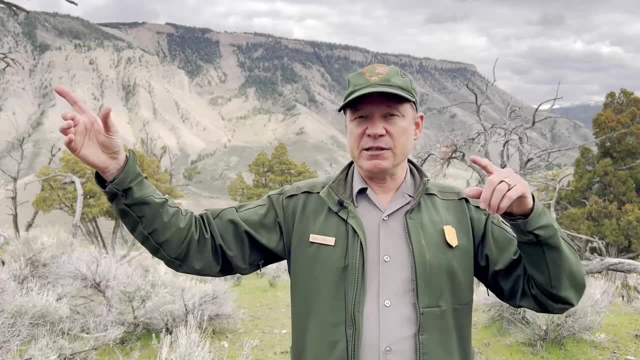 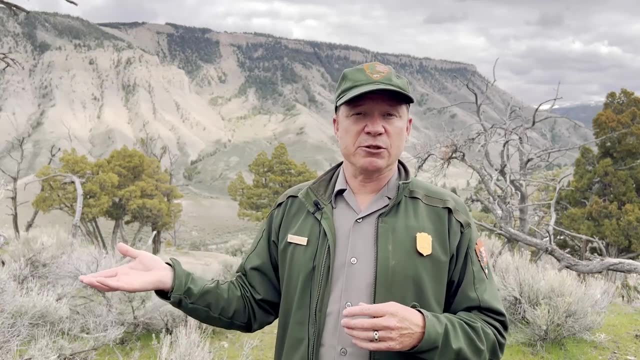 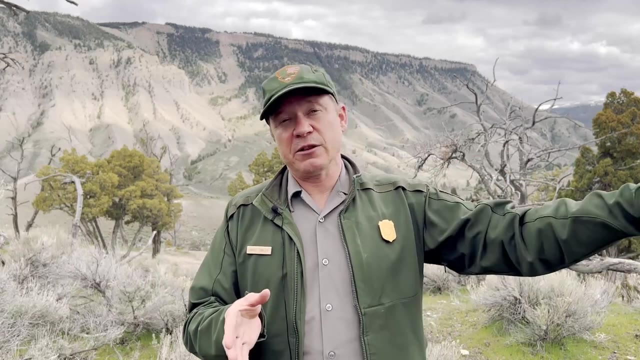 throughout the greater Yellowstone ecosystem because, remember, elk are migrating throughout the year to these different parts of the ecosystem. Some of that includes entirely within Yellowstone. We have, for example, cows that will spend the winter right here behind us in the northern range of Yellowstone, and right now some of those cow elk are starting to move down to. 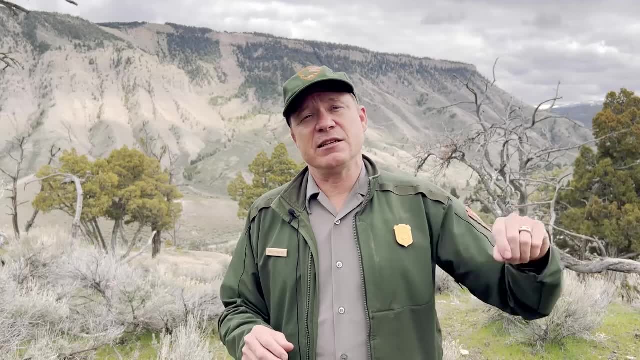 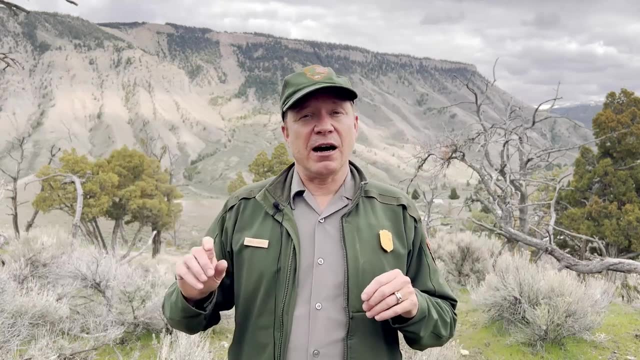 their summer range down near Yellowstone Lake. So they'll go all the way down, you know, 50 miles down into the interior of the park or further to their summer range, to track that food resource. Other cow elk are migrating north, uh, or up into the higher elevations here to the north or the. 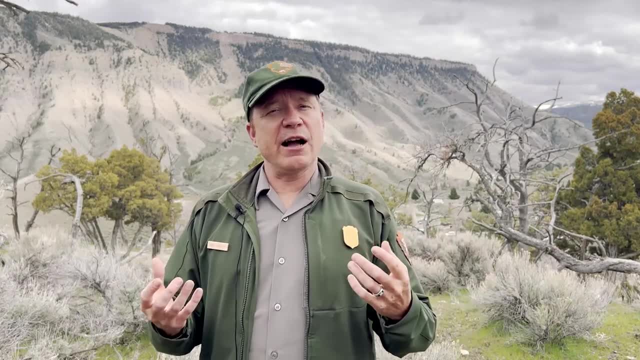 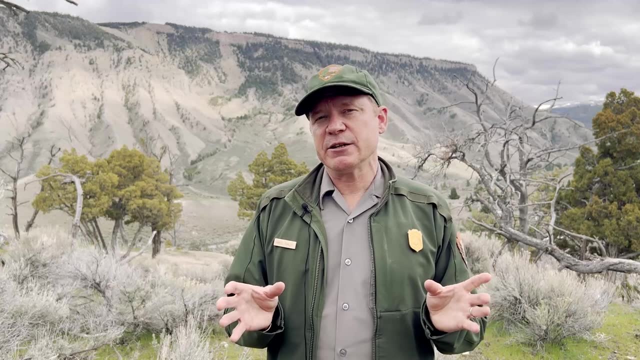 east and the west of the park. so it really depends on what those young elk have learned from their mothers and that they tend to follow those same migration patterns. Again, when we come back to the predation, what we've learned here is that the decline in elk 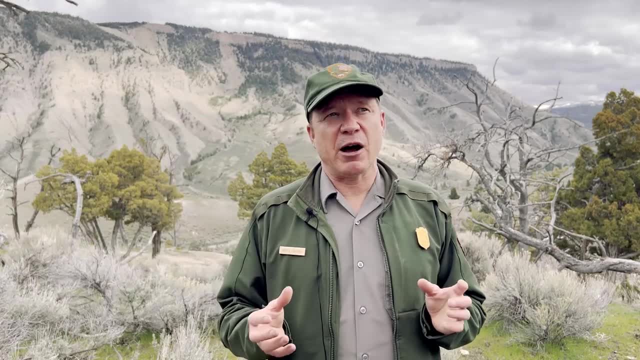 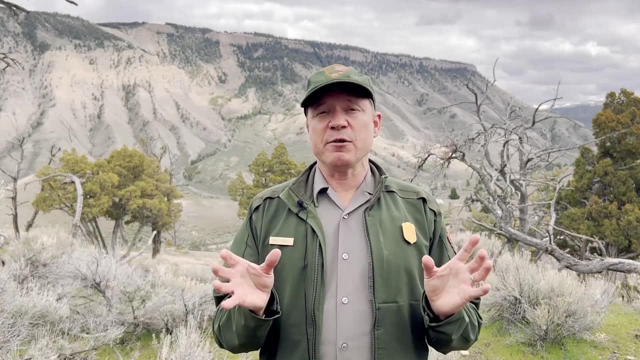 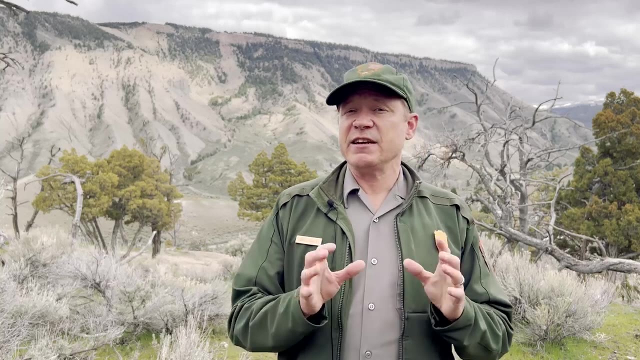 in the story of elk population growth and declines is really driven by a number of factors. So let's go back in time and think about the history of elk in this park. in the past, We have to remember, for many thousands of years, elk were an incredibly important part of of native peoples, The 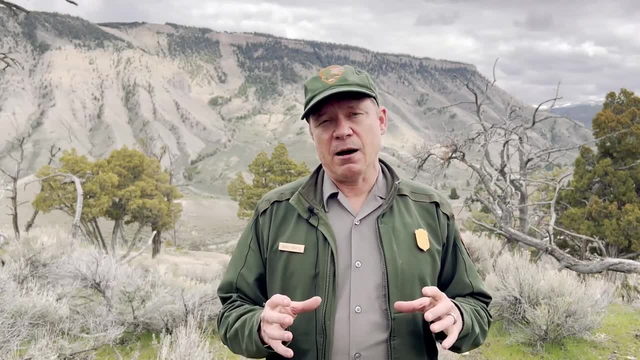 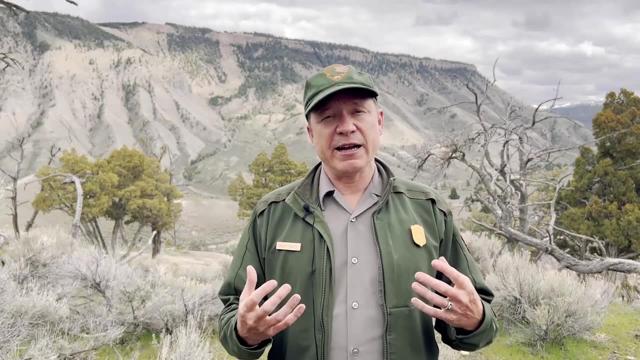 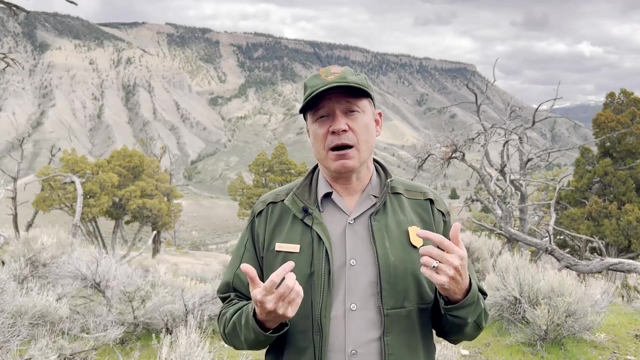 different tribal nations that have used Yellowstone historically were very much focused and relied on elk for source of food, through the meat for clothing, because the hides were really strong and easy to work with Elk ivories, which are the teeth, the canine, vestigial canine teeth of an elk, 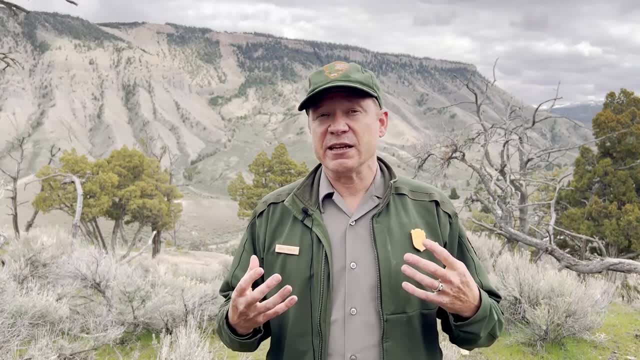 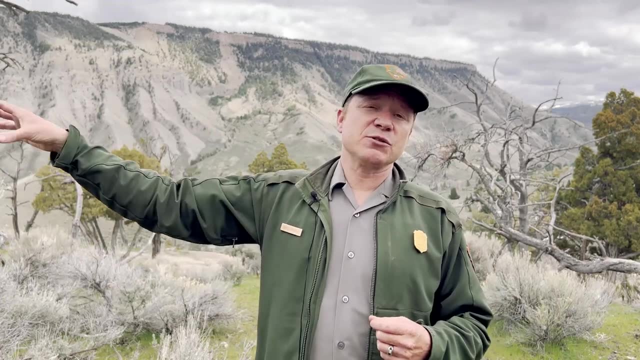 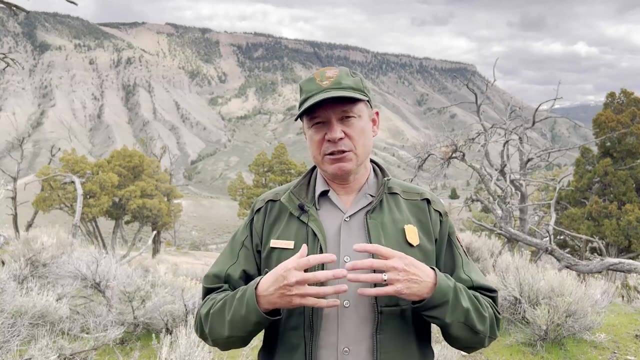 were really important for certain tribes: clothing and decorations for a part of their cultural and spiritual connection to these places. In fact, the Yellowstone River that flows out of Yellowstone National Park has been referred to by many of the local tribes as the Elk River. That, right there, tells you just how key this animal was to many people in this. 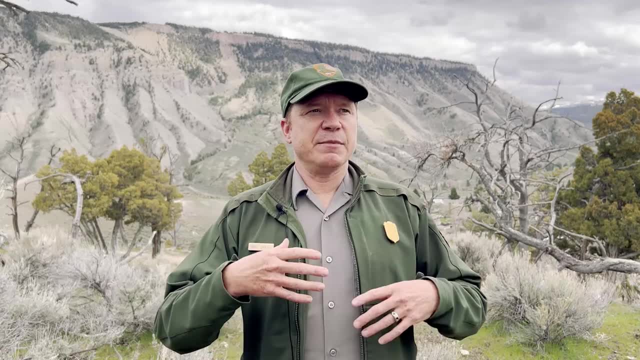 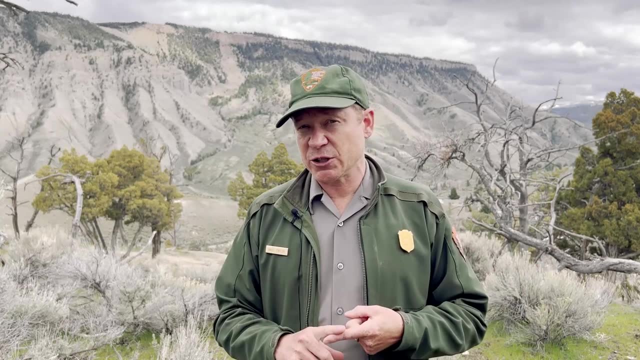 landscape for thousands of years. When the park became established 150 years ago, it was seen as a sort of a wide open era where there was large-scale destruction- uh, through market hunting and poaching of our wildlife populations, and elk were very much subject to that. 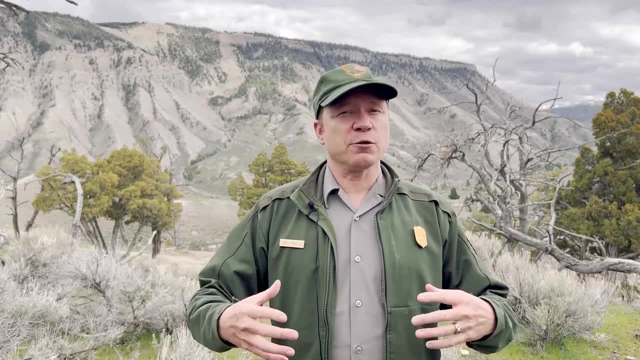 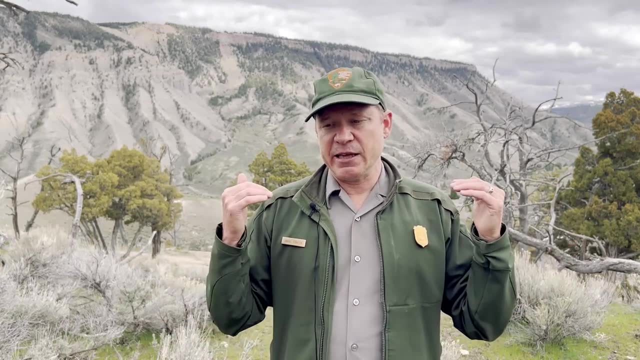 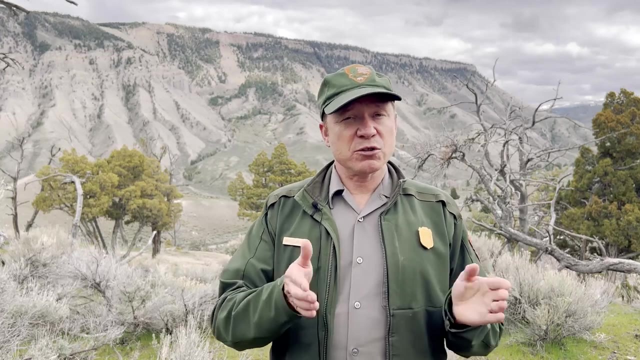 And so there was a big collapse in what was originally described as flourishing elk populations. when the early explorers came here, Lewis and Clark described this landscape of full of elk and and the early period of Yellowstone's history was one of destruction of many wildlife, and elk were part of that. When the park service uh got into a new era where the 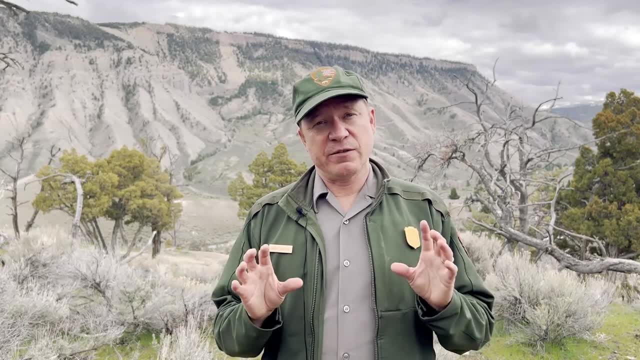 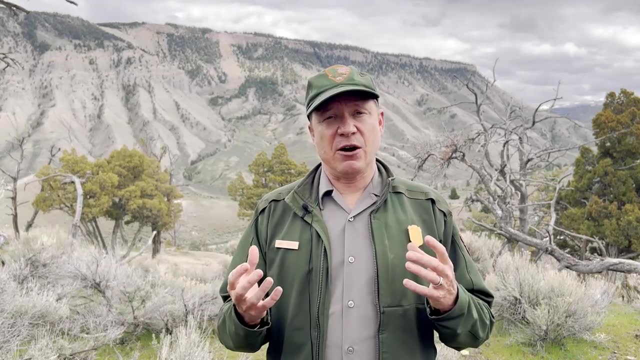 US Calvary took control. they protected a lot of uh animal species- not all, because they got continued to get rid of the predators which are important part of the story of elk here- protected the elk and to a point where they were feeding elk in the winter time and then we entered. 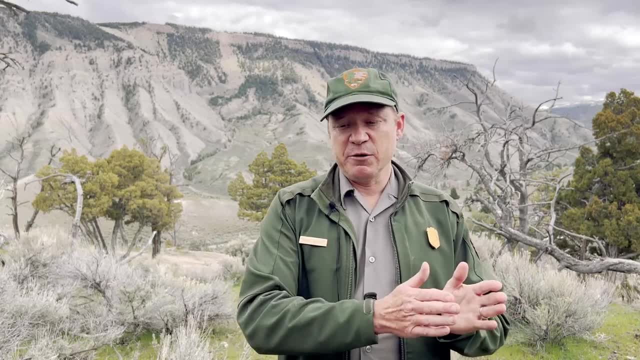 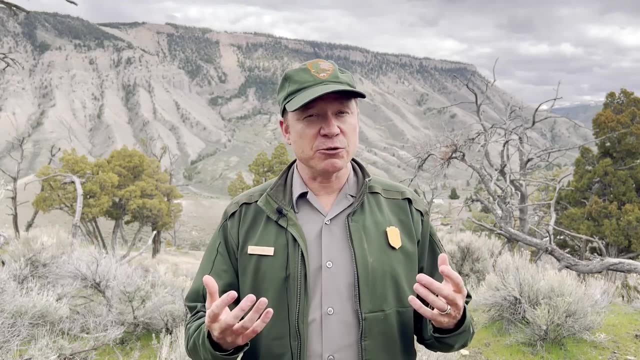 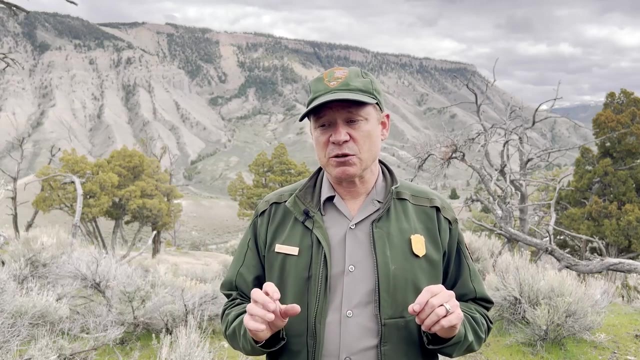 the era when the park service was created. uh, in that era, moving forward for about 50 years, much of the principles of managing animals like elk fell in line with the philosophies of agriculture, particularly when it came to controlling ungulate numbers such as elk and bison and pronghorn, and and it was sort of at a time when we really didn't understand the. 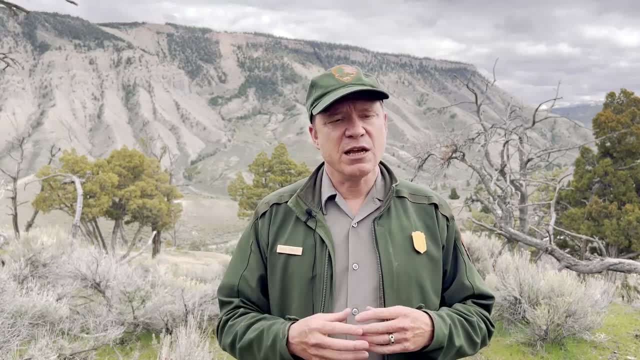 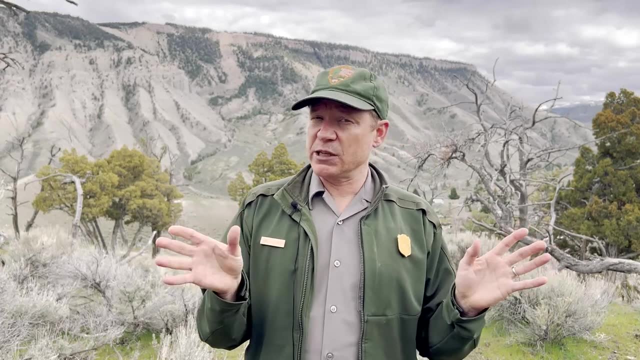 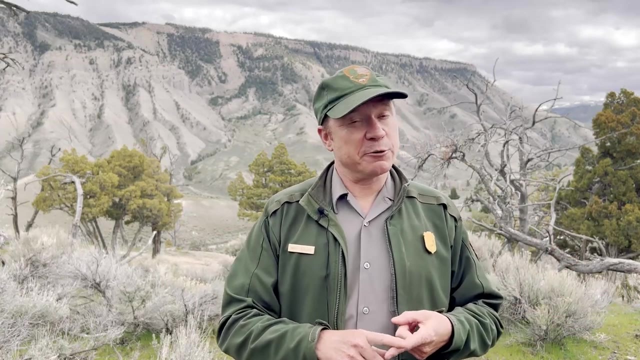 ecology of natural systems and the importance of things like predators and how weather and other uh ungulate dynamics like elk. and so the park managers at the time, working with what they thought was the best information available to them, managed elk uh very heavily. this involved periods of time when there were too few elk and then uh in good winters when there wasn't severe. 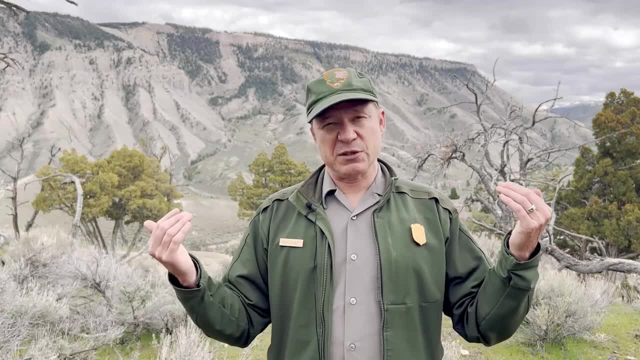 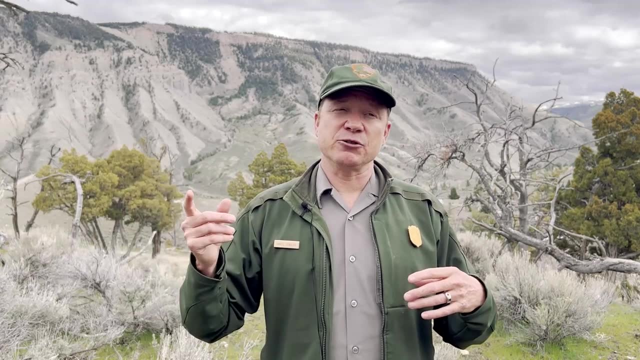 winters that population would grow. then it was felt there were too many elk so there was elk culling and that involved shooting and killing elk not only inside the park but a lot of elk just outside the park boundary. but it also involved a really important part of elk. 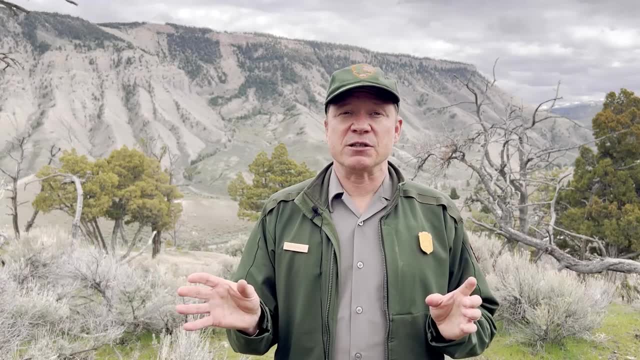 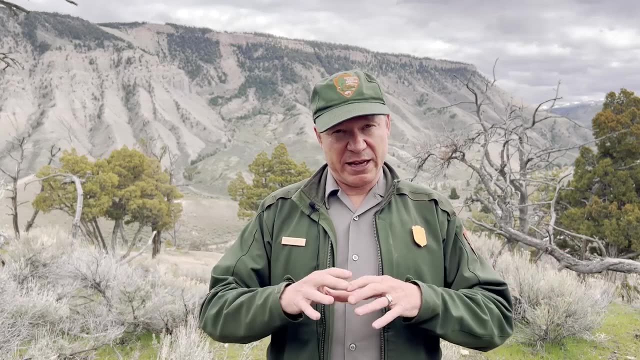 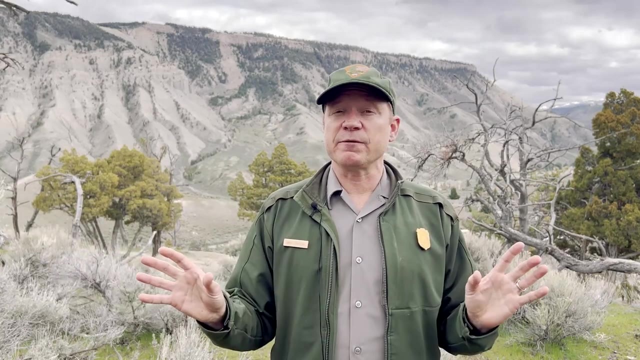 conservation throughout this country, and that is elk translocations. from the period of the 1930s until the mid-1960s, approximately 15 000 elk were translocated out of yellowstone national park to restock elk populations or recreate new elk populations throughout the lower 48. 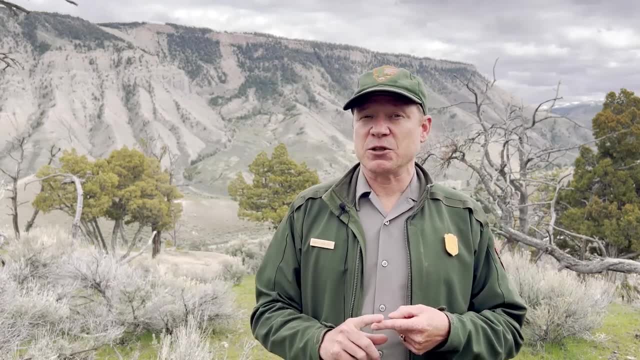 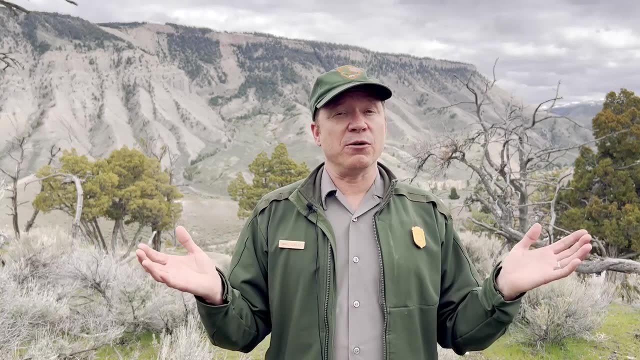 into canada. even argentina and mexico received elk from yellowstone. so it's a real important testament to the importance of yellowstone and the story of elk, not only in our local area here, but elk throughout north america. yellowstone elk are at the core of that story of elk conservation. yeah, i used to work down at rocky. 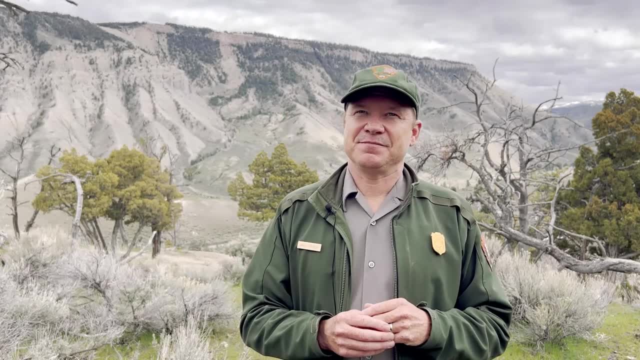 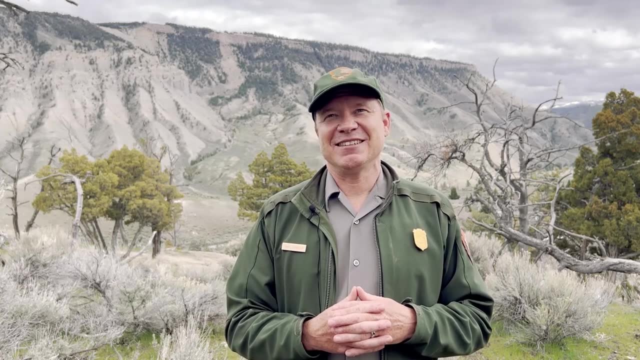 mountain national park and that was a big thing that we talked about. we had pictures of all the the trains that had the elk and they put them on a truck and load them out and just let them out into the park and now they're everywhere down there. yeah, i mean, it was very much the model for uh. 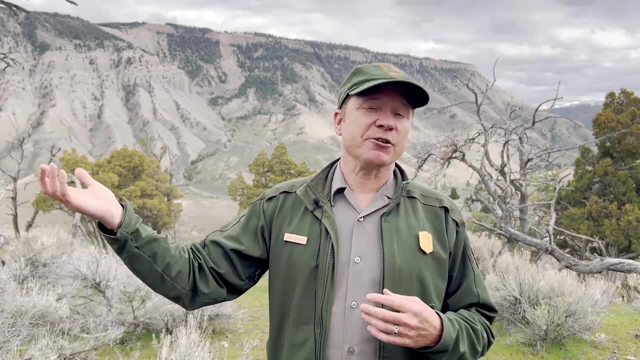 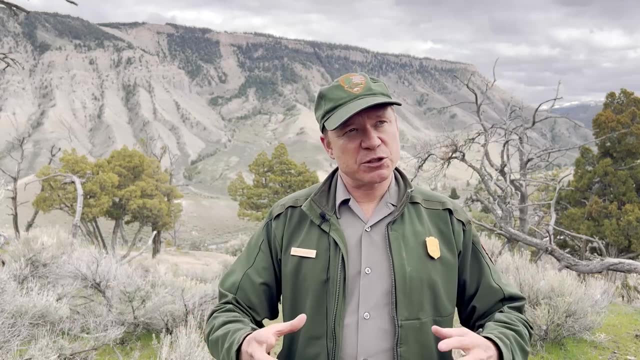 the restoration of a large-scale ungulate. we can look to the bison today as another great example of the importance of yellowstone in that conservation story. um, and then when the late 1960s uh came along, there was a sort of a new paradigm of how we thought about how natural systems worked, and that was really 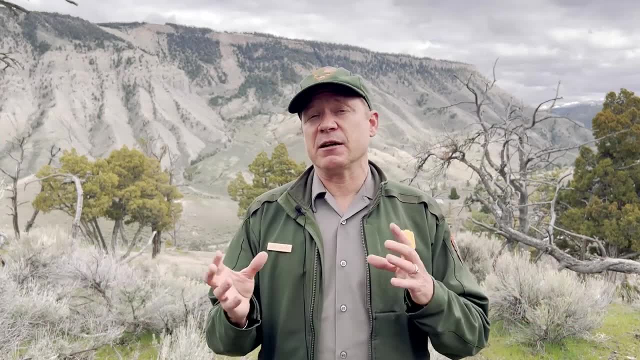 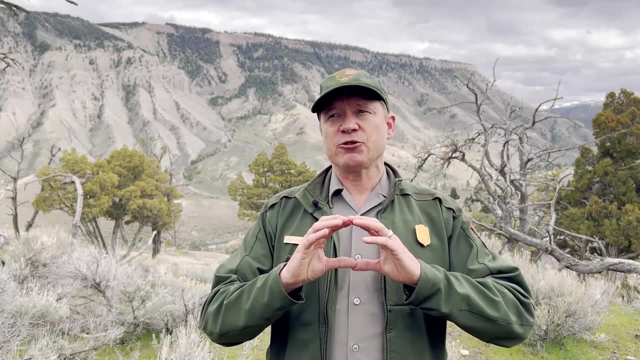 sparked by aldo leopold, he was uh contracted with the team of biologists to do what was called the leopold report and that really built off predecessors of his like george wright in the 1930s that really kind of tried to get managers in places like yellowstone to think about uh. 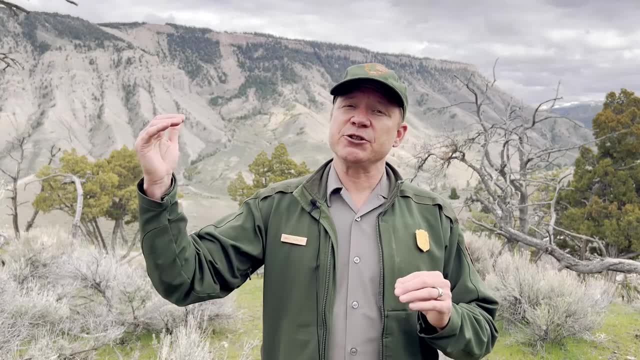 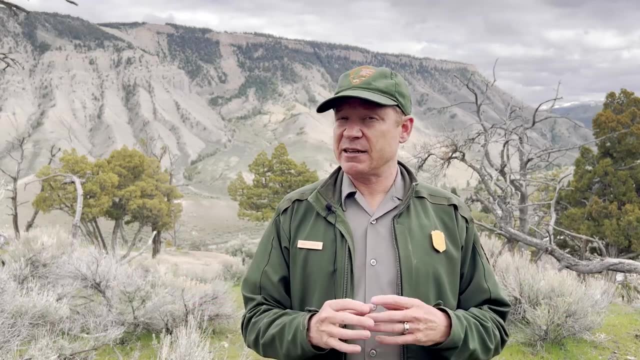 managing ecosystems, um uh, under the power of nature, not the power of humans. so, starting in the late 1960s, the park changed the philosophy on how elk were managed, and that was to let nature know that there was no more elk translocations, there was no more elk culling. i mean there had. 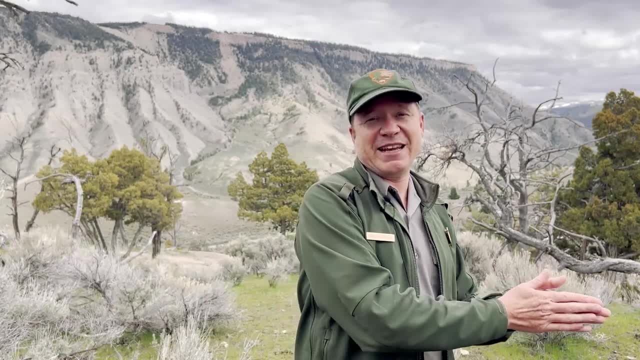 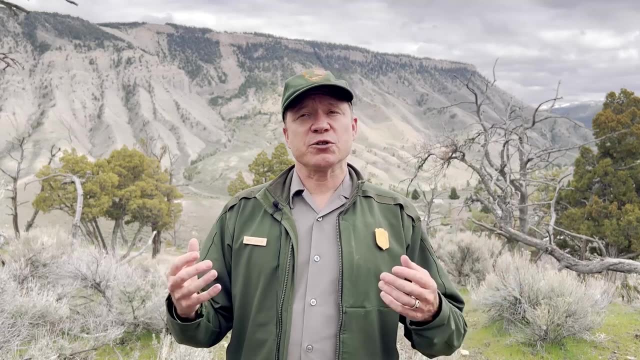 been over 50 000 elk killed in yellowstone from the early 1900s up to the late 1960s- a significant number. and then, all of a sudden, nature took back over. so elk were no longer subject to humans but to the, for the most part within the park. of course there was still hunting. 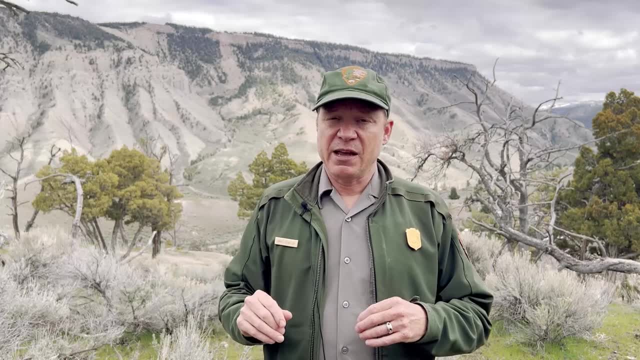 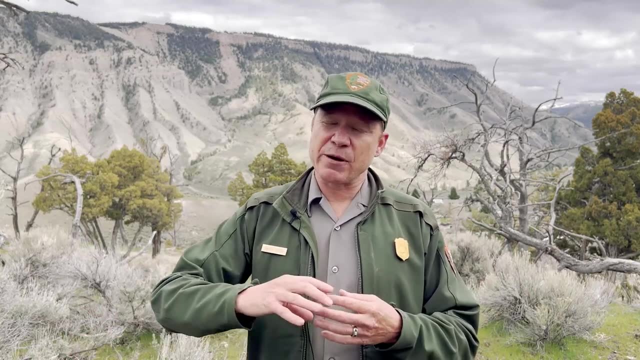 just outside the the park on some of the elk, like the northern range elk herd um. at this time, remember, though, predators have been eradicated from about the 1930s until we get to the end of the 1980s, and we get to the end of the 1980s and we get to the end of the 1990s. 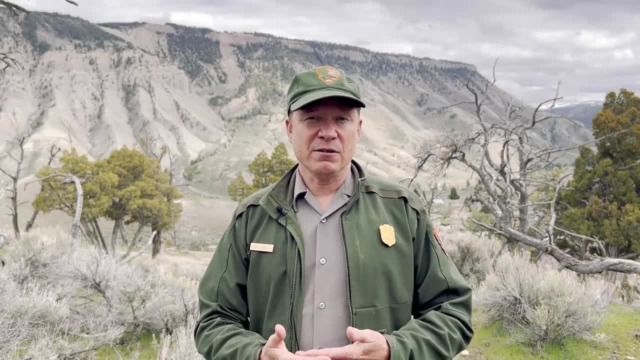 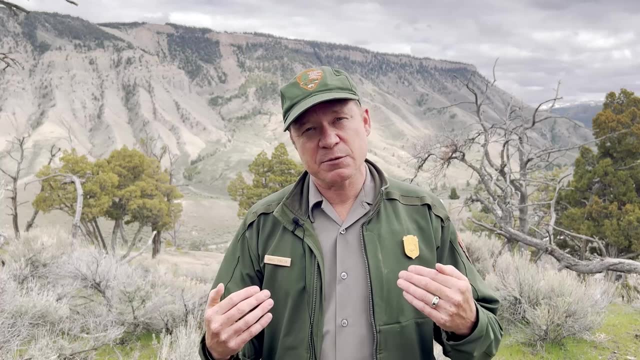 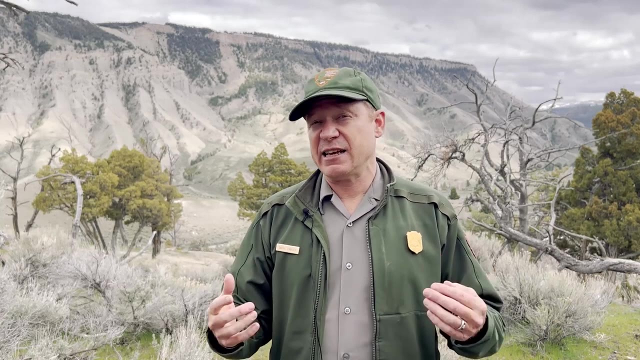 um elk were largely at the fate of weather events: severe winters, severe summer drought. these are all important regulatory mechanisms for elk. they can impact pregnancy rates, the ability of elk to put on enough fat to survive a winter. the 1988 fires altered a lot of habitats and that was. 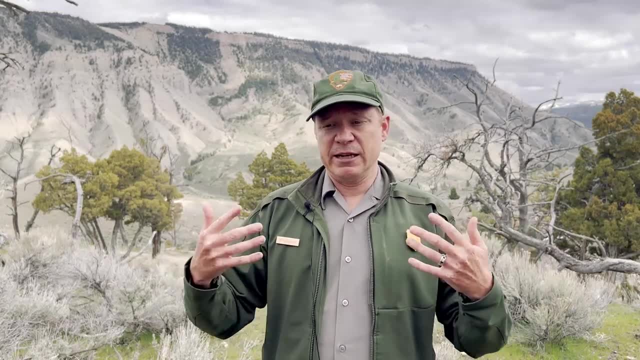 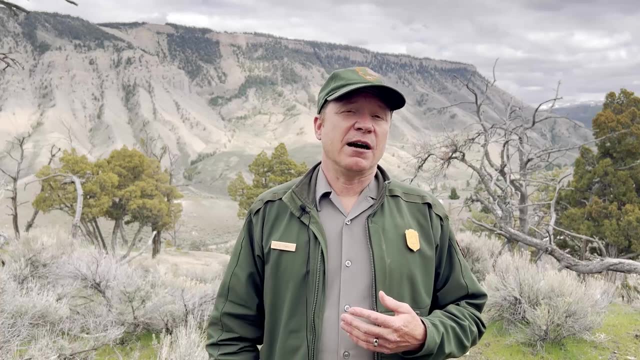 coupled and followed on the heels of some severe winters, and so it really was what we were seeing: the population that was knocked down by the powers of, of, of, um weather, uh, severity, um, because predators weren't there in place to kind of have that regulatory effect and, as a result, that 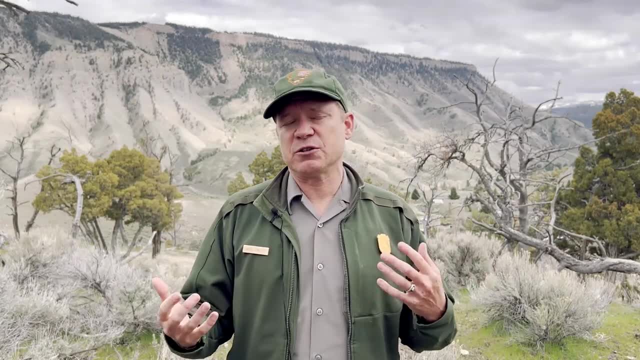 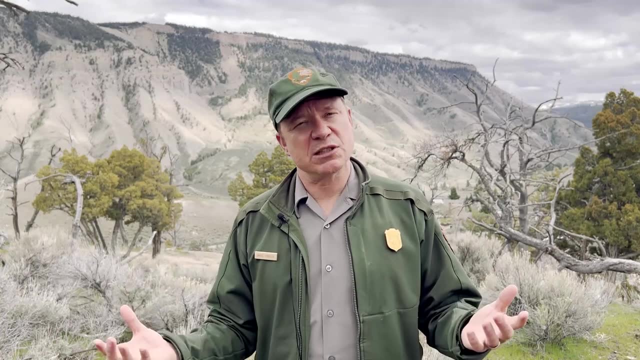 population skyrocketed, once again to what we think of as a sort of an artificially high number and and not particularly within what we would think of as or call the carrying capacity, what the resources can support. and so what we saw is pregnancy rates decline, survival decline under 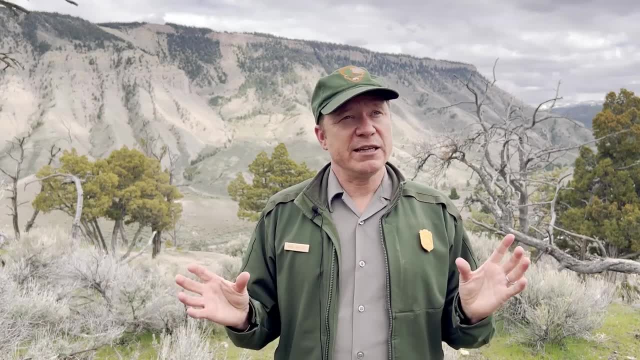 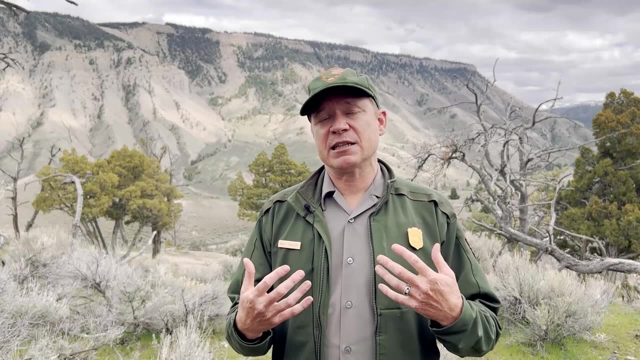 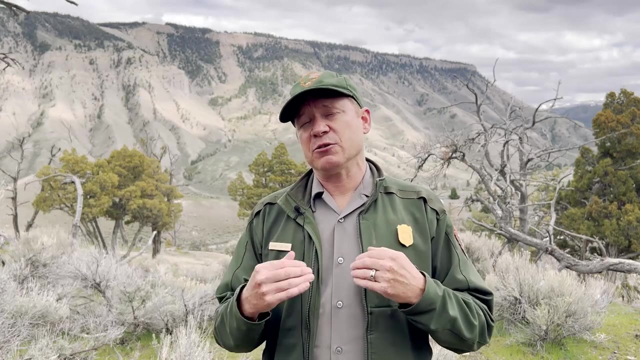 high densities of elk and that's why it was recommended that to really have an important effect on the natural processes of yellow stones wildlife species, which is part of our mandate as a national park to preserve natural processes, to restore native species- it was decided that predators were going to be a key part of the elk story, and so wolves. 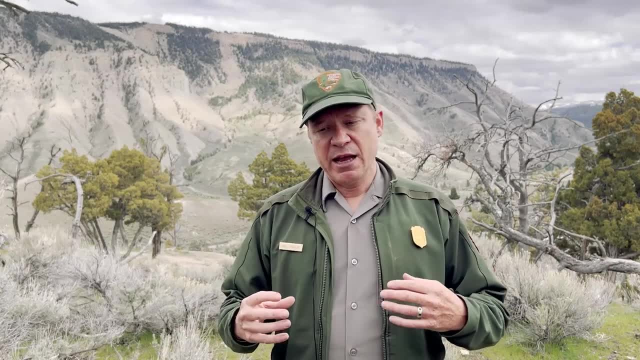 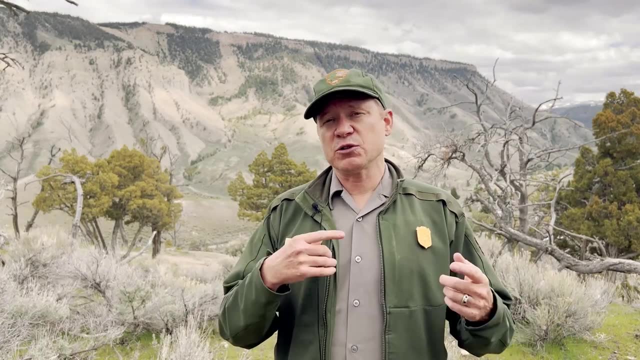 reintroduced in the mid-1990s. as i mentioned, cougars came back on their own and and grizzly bears and black bears are really important predators of of elk, particularly elk calves, this time of the year. so all of those carnivores back in place. um really played a role collectively. 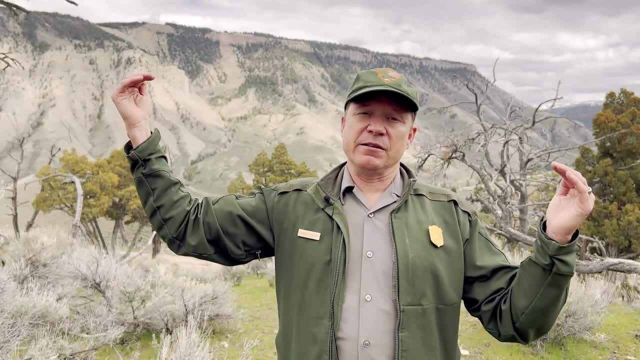 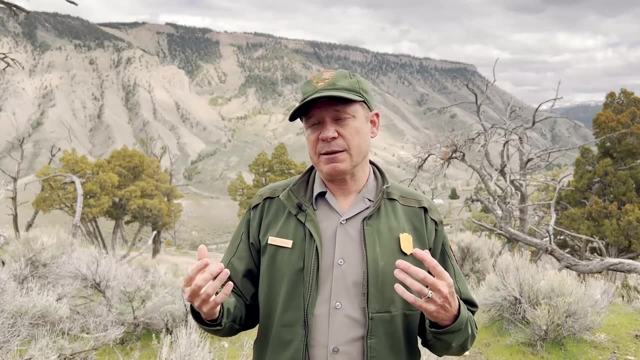 along with human hunting just outside the park here on on that decline of what was thought of as a really super abundant elk herd back to a population level that we think is much more in tune with this landscape. so if we look at elk today in yellowstone and we just look at the 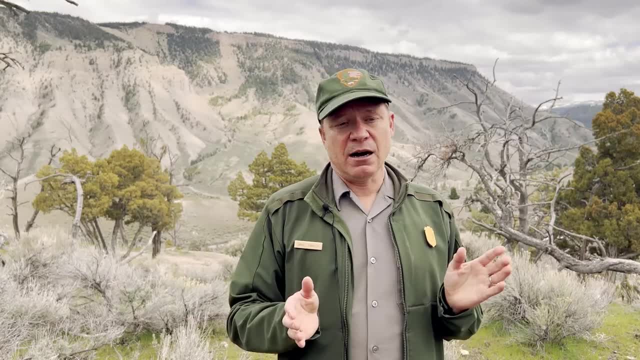 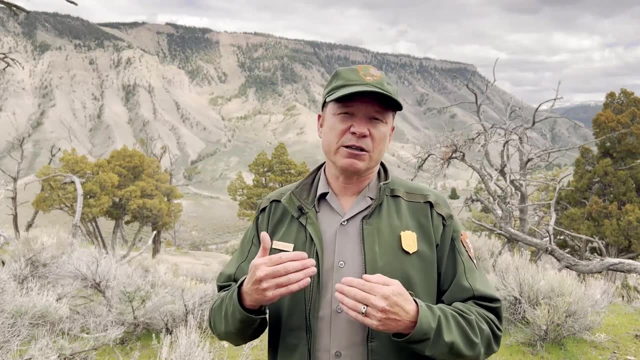 northern range elk, which is one of the best known and best studied. again we have what we think is a very stable, healthy population of elk when you look at where they are in terms of uh target objectives. we, the national park service, don't set uh population objectives for species like elk. again, 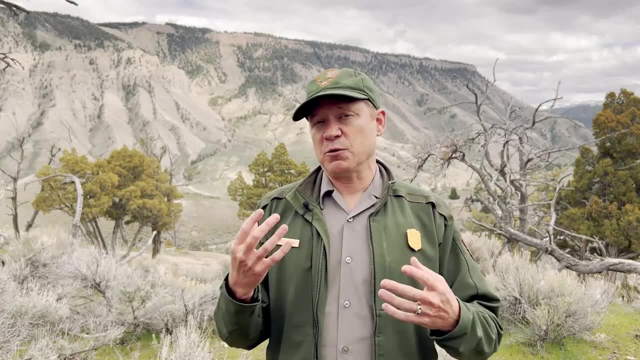 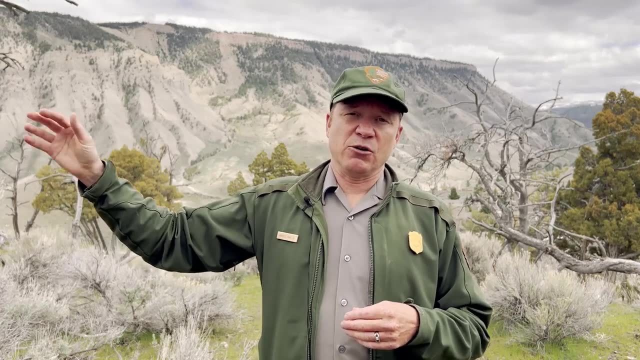 nature take its course. we let them be subject to the natural forces around them, such as predation and disease and weather. but this elk herd is incredibly important: cultural elk herd and economic elk herd. when they leave the park there's a. they play a key role in the state of. 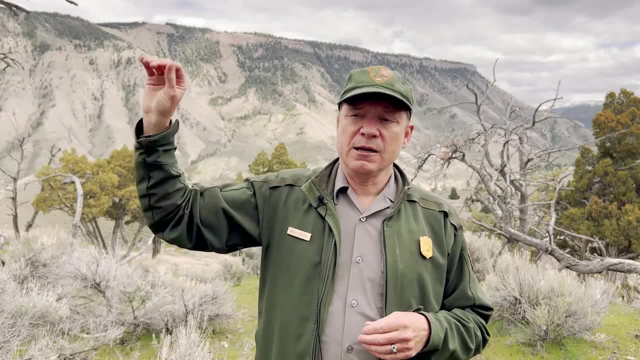 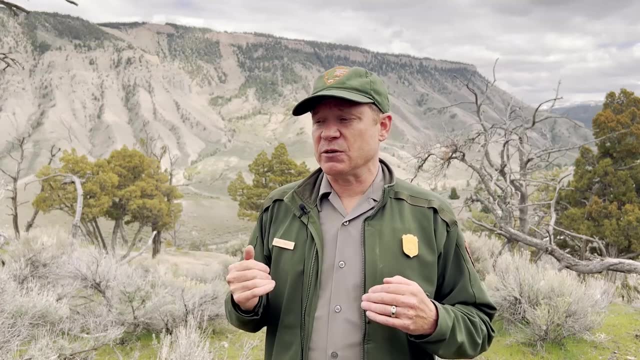 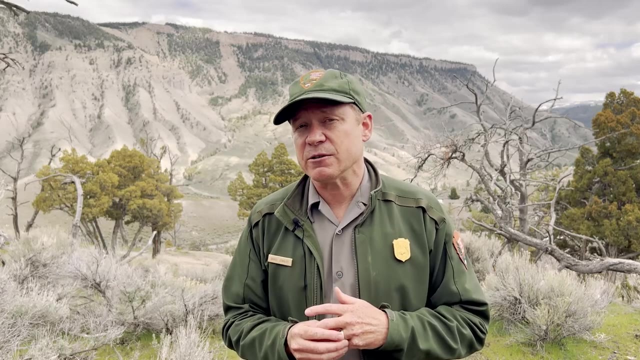 montana's hunting economics north of the park. they provide meat for a lot of people in addition to the natural carnivore species here, and so humans are very much a part of that story and moving forward will be continued be the uncertain of yellowstone, uncertainty of their future, is looms large. i mean there are emerging risks for elk such as 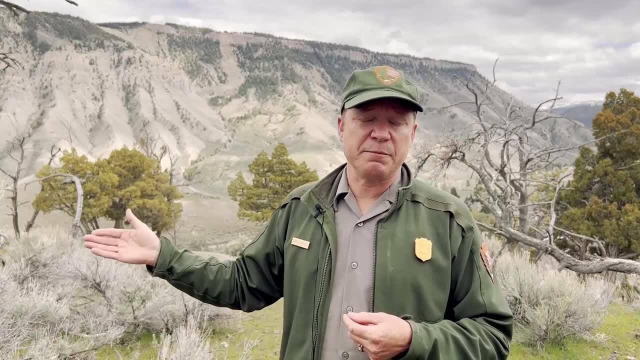 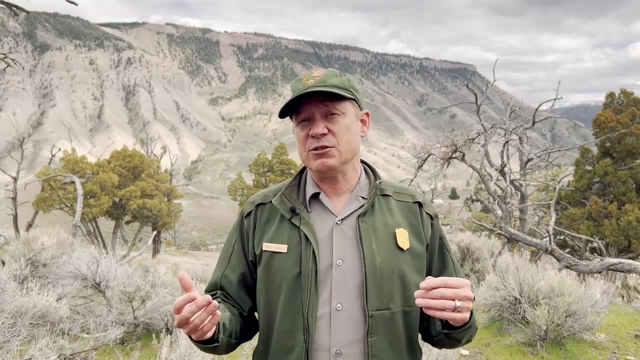 diseases like chronic wasting disease, which is at our doorstep, potentially here, although we haven't detected it in yellowstone yet- and that can be a fatal disease. or that is a fatal disease to deer and elk and other ungulates that get chronic wasting disease. so we're watching that. 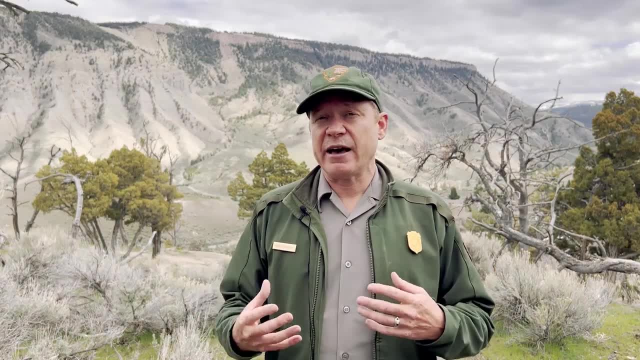 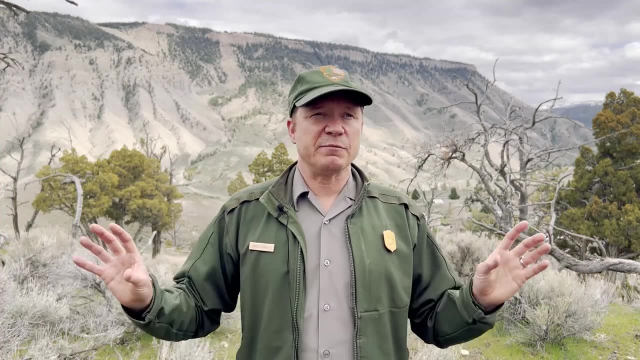 emerging threat. uh, brucellosis is another disease that i'll carry and of course that could be a potential transmission to livestock when elk leave the park. in fact, cases of brucellosis that have been transmitted to cattle in the rocky mount west around yellowstone have. 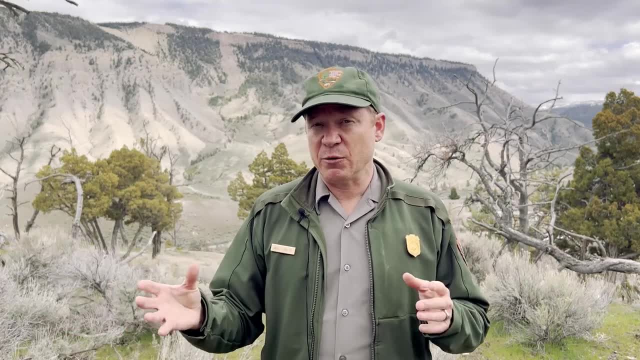 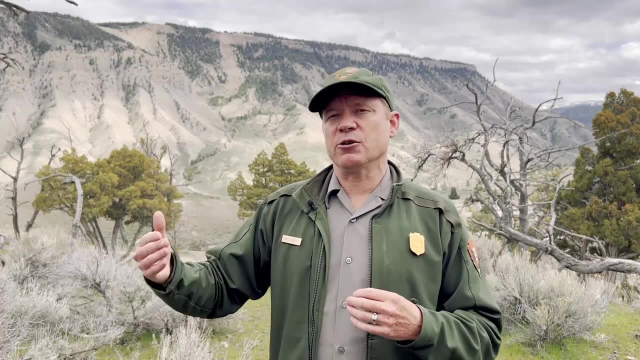 been actually transmitted from elk, not bison, even though we always hear about the story of bison, the threats of bison spreading brucellosis. so those are diseases that we as humans are interested in learning and understanding what those dynamics are. and so those the future there is uncertain. 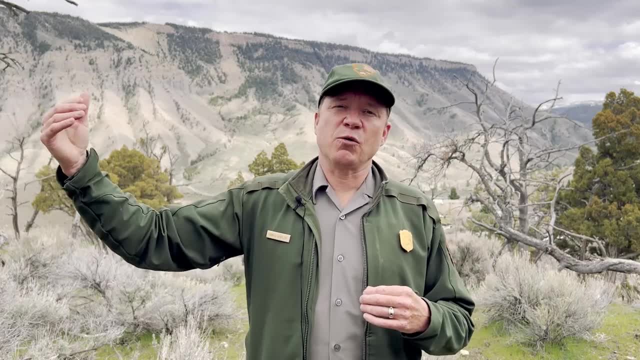 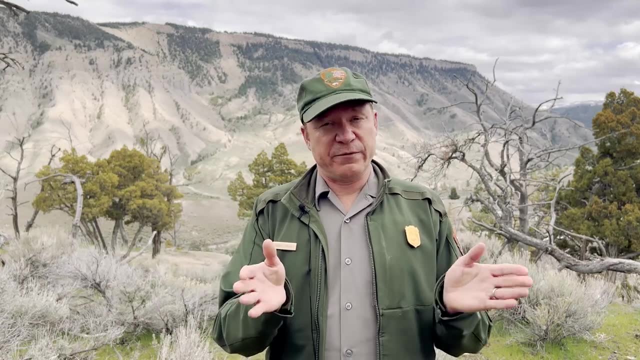 of what that will mean. uh, huntings will still play an important role. in fact, what we learned by studying the effects of human hunters on our northern range elk herd is that they actually play a significant role in the first decade of wolf recovery on the decline of northern 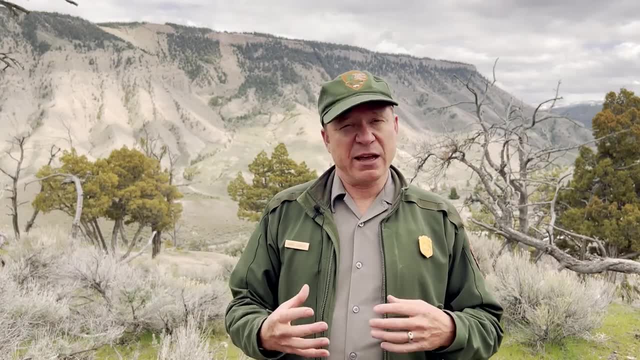 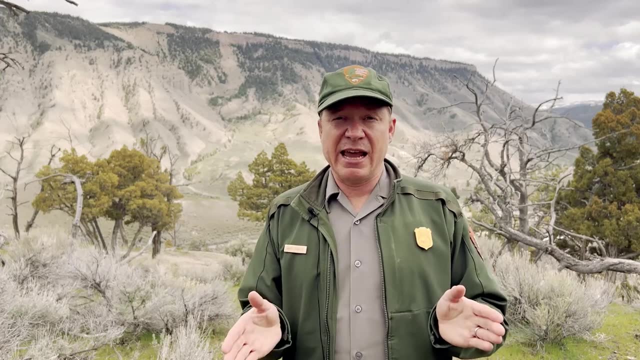 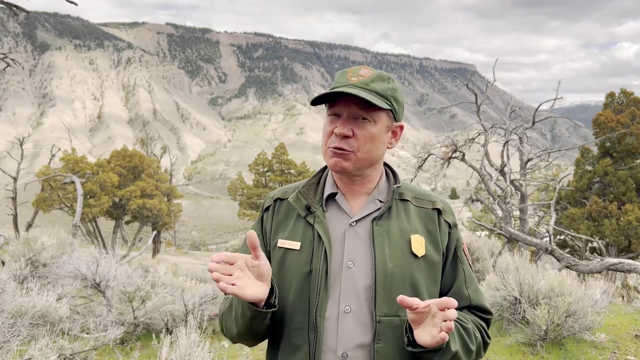 elk compared to wolves themselves, because we have really good understanding of wolves predatory role and predatory effect on reducing or regulating elk numbers. we think today, over the last decade, wolves are playing a more important role. so too are cougars and bears on elk population dynamics, particularly through their impact on elk calves, because they 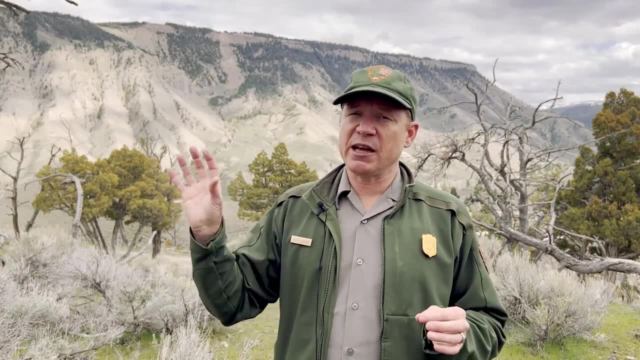 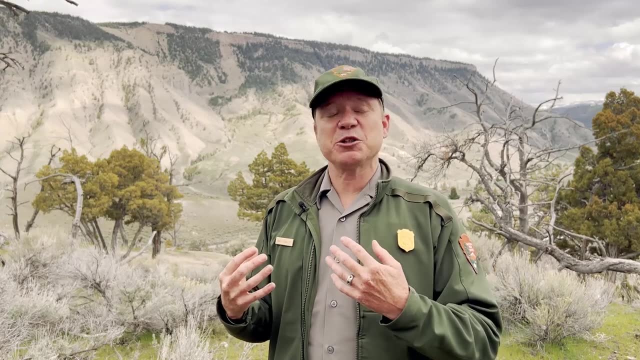 kill a lot of elk calves collectively this time of the year. human hunting still occurs north of the ocean, outside the park. there's no hunting inside yellowstone, of course, but so humans are still very much part of this dynamic. so, even though yellowstone has adopted management practice of 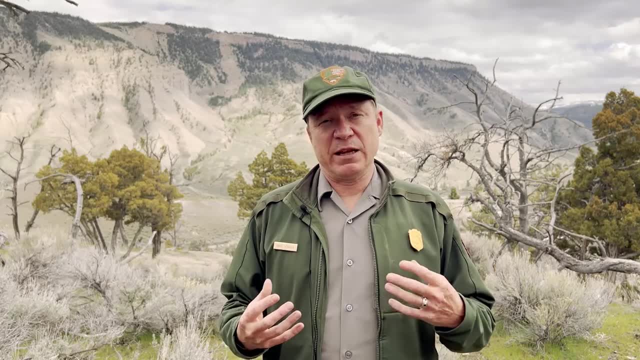 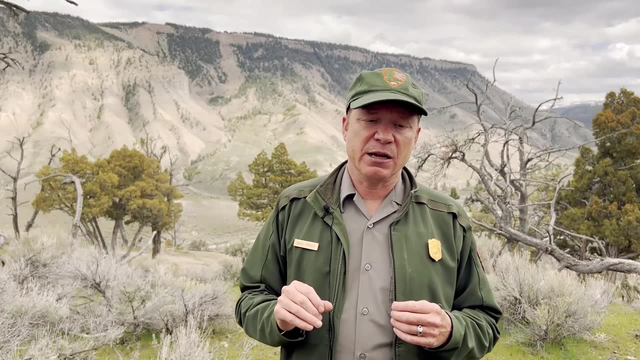 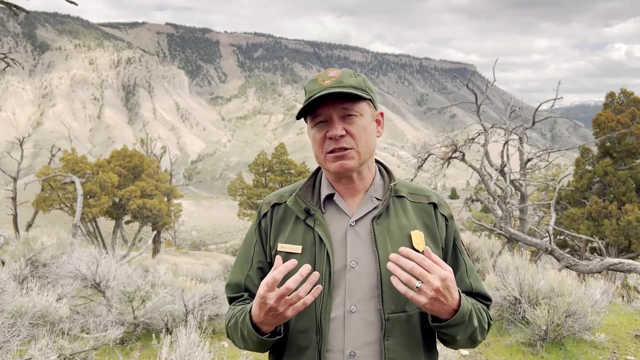 letting nature take its course, restoring large carnivores, and that in part is to help with natural regulation of ungulate numbers. humans are still very much part of that story just outside of the park but we have what we think is a very healthy and resilient elk herd. i think the elk to me is 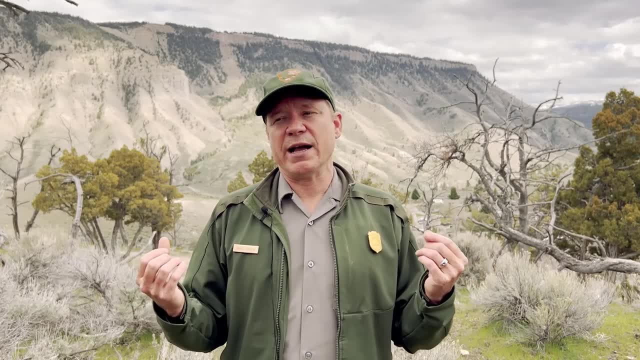 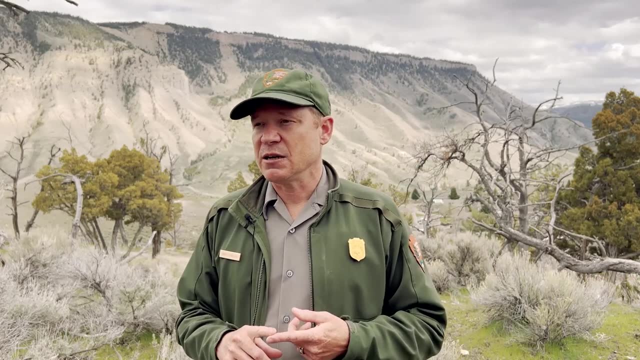 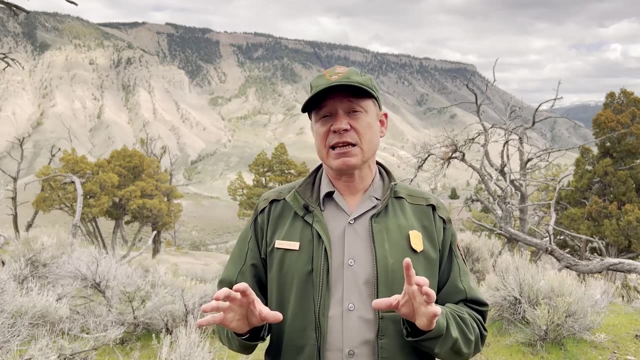 sort of the ultimate animal, the rocky mountain west. they are incredibly resilient to the challenges that they face in a place like yellowstone: the harsh winters, the unpredictability of food resources from one season to the next, the risk navigating a landscape of risk for predators- and they're really good at that. 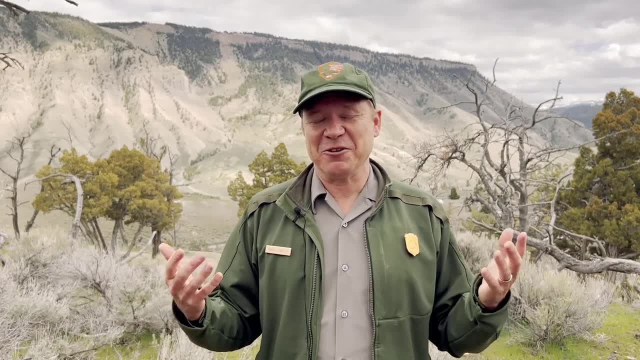 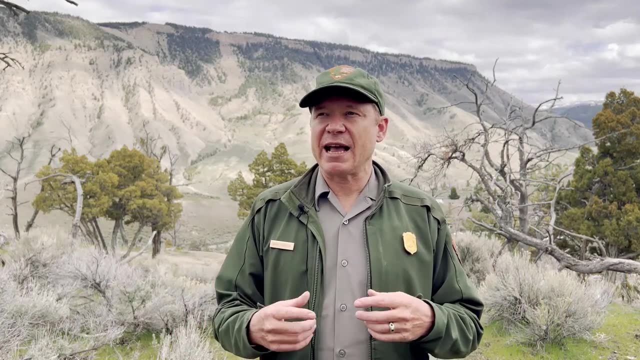 again, they're not particularly just sitting there as wolf bait or cougar bait. they actually have evolved many strategies to be successful living and co-existing with carnivores, and that has to do with things like grouping safety in numbers. so elk tend to group up in herds. that creates more eyes and senses for. detecting lurking predators and, like i said before, you know wolves need animals like wolves and particularly need vulnerable prey to be successful. so a prime age cow between the ages of 2 and 13 is really doesn't have a whole lot to worry about. they're not really a target of wolf predation. 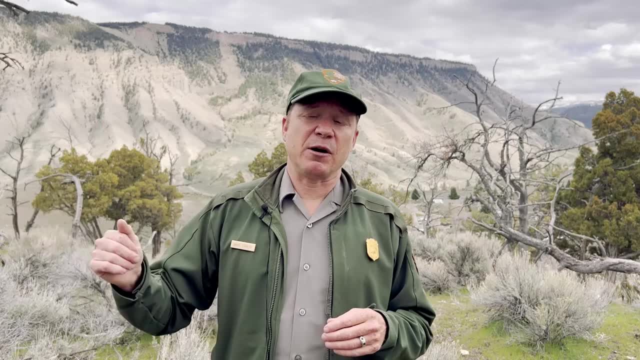 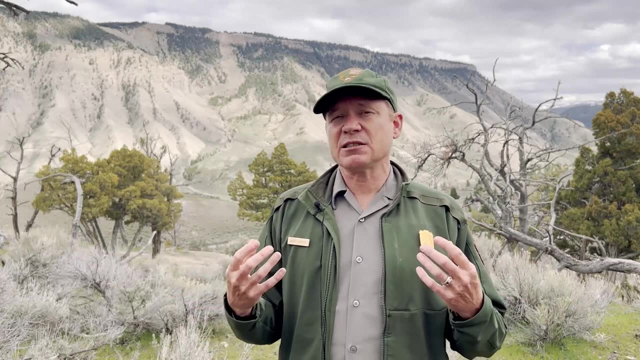 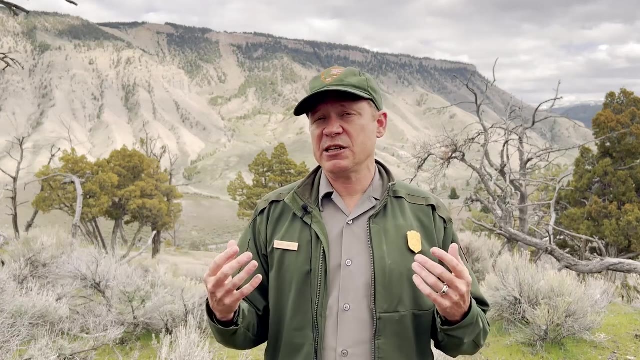 but their young calves are and so too are the older cow elk in that population, so they can. they can face predation risk and navigate that landscape quite successfully. the park is trying to study and understand competition between the, the different ungulates, the hoofed animals. so we have long-term work collectively, our team to study how elk are. 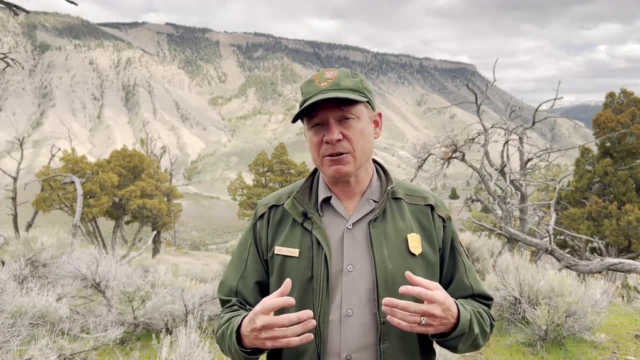 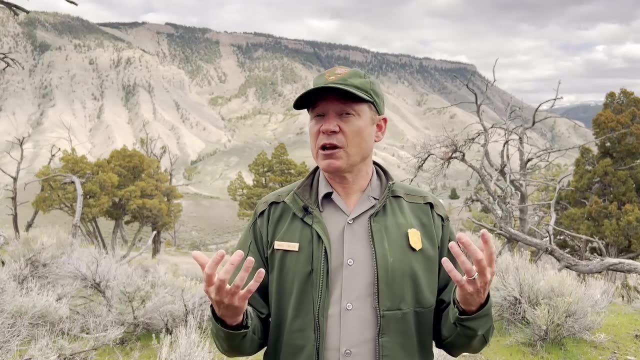 competing with bison, pronghorn, bighorn, sheep, deer and the other ungulates that they share this ecosystem with. who gets what resources? is there enough for everyone right now? our current understanding of this landscape is they all play a really important role in the grazing. 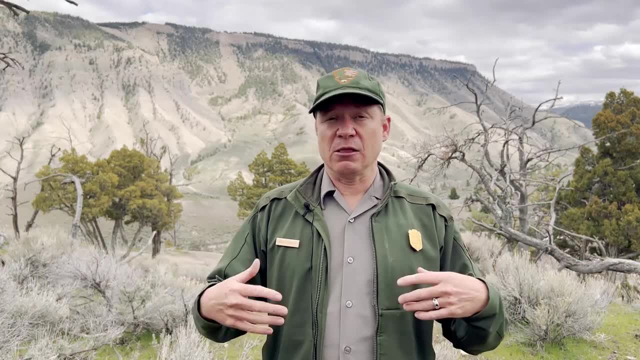 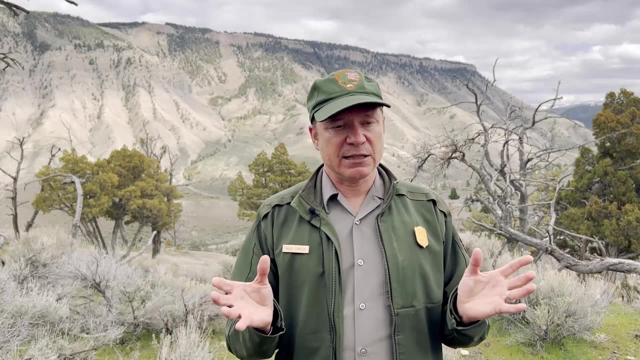 community and grazing health of our grasslands, and there's a lot of food for even a lot more animals, a lot more bison and elk- than we see today, and so what's really important, moving forward, is for us to engage with a diverse body of stakeholders, people that want to come here and 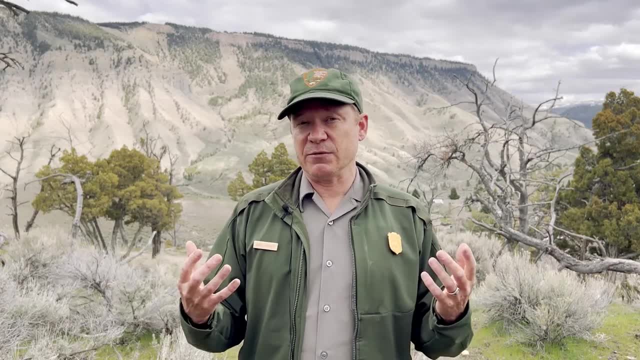 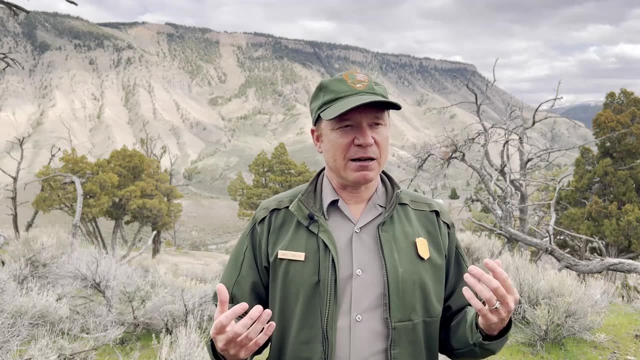 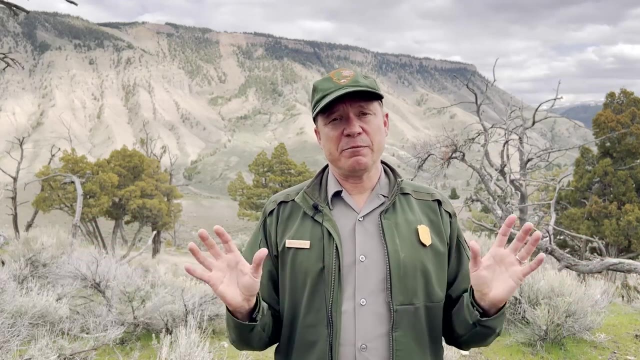 experience yellowstone for its abundant and diverse wildlife, to be able to see elk and wolves interacting with one another, whether it's to photograph them, for to nurture our souls and our spirit, just because it might be an important part of our culture. it supports a huge economic viability. 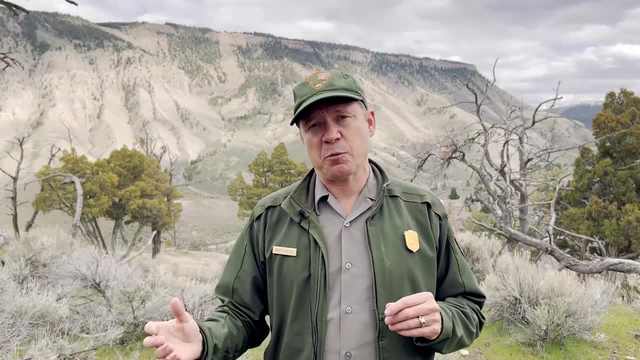 of our surrounding communities, not only the park, but also the environment, and so that's what we're going to focus on today. during this time of pandemic, we're going to do the best we can to help our communities protect themselves and our wildlife, and to make sure that we are not only protecting ourselves. 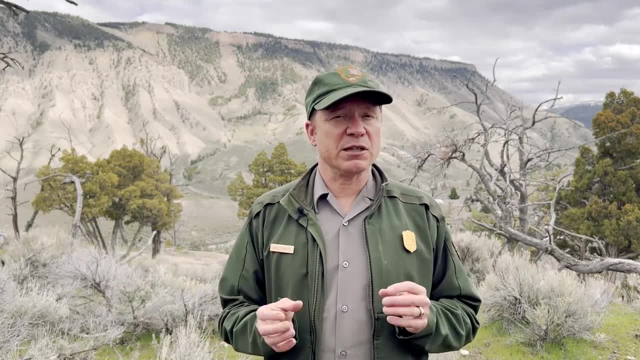 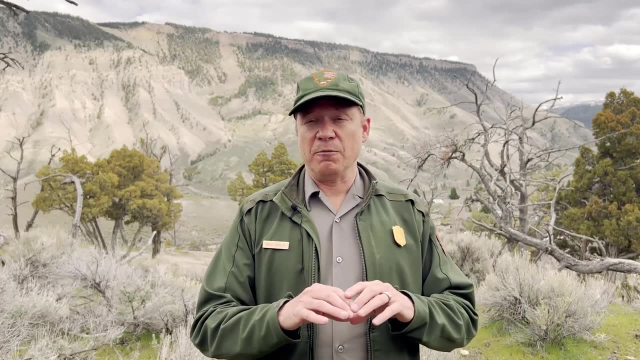 but our surrounding gateway communities for people that want to have healthy, robust populations of species like elk, and so they're really incredibly important to yellowstone's past. we've learned a lot about managing wildlife and, maybe more importantly, how to not intervene and manage them, and let 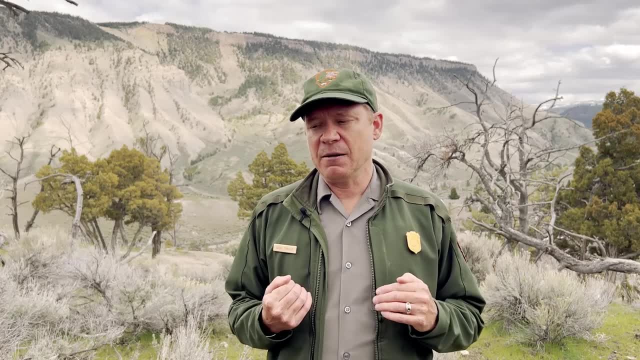 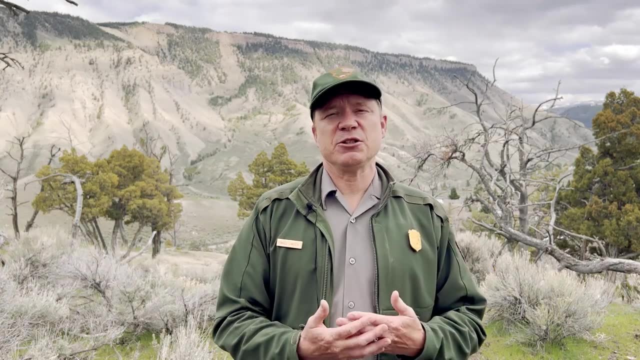 nature's processes, take control and, again, that's our mandate as a park service. now that carnivores have been restored to yellowstone, we have one of the most unique opportunities to understand how a species like the elk faces nature and how it's been managed in a way that they don't want to be. 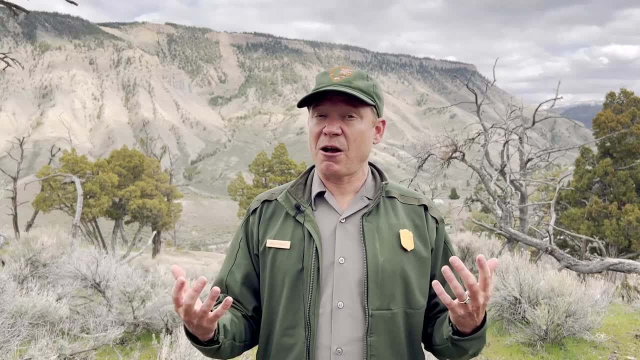 threatened or affected by wildfire and in that way they're able to protect themselves and the wildlife that they don't want to be affected by wildfire. and in that way, they don't want to be affected by wildfire and in the challenges that I've just discussed yet still thrive, which they very much. 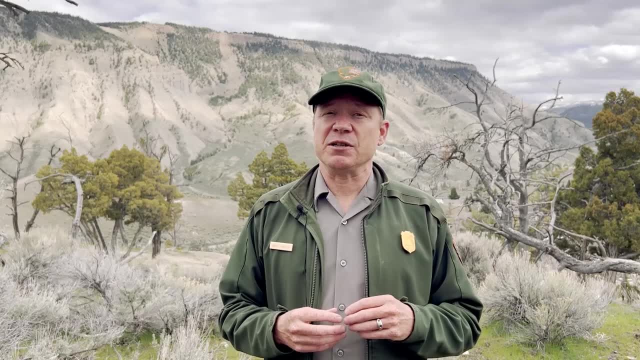 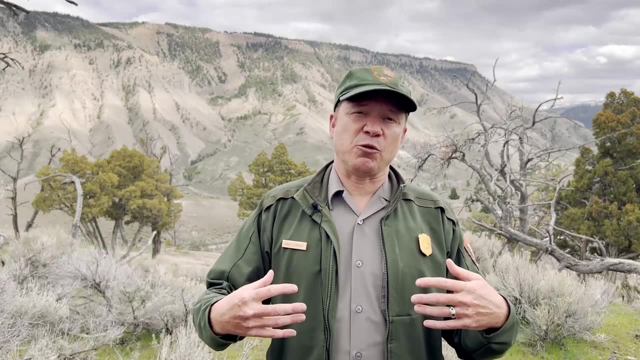 are doing. We have very healthy, robust elk herds in the greater Yellowstone ecosystem- and once more moving beyond our borders of the park, recognizing that elk rely not only on Yellowstone National Park for their safety and security and success long term, but as well as the public and private lands, 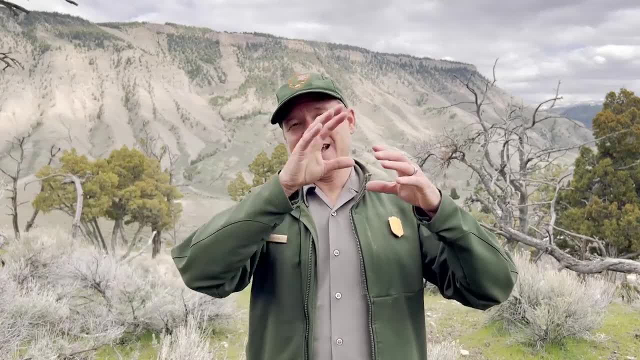 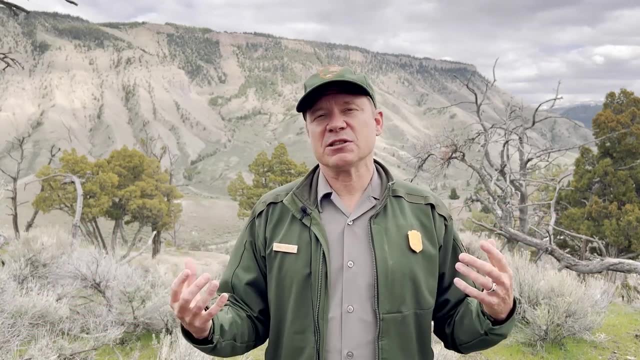 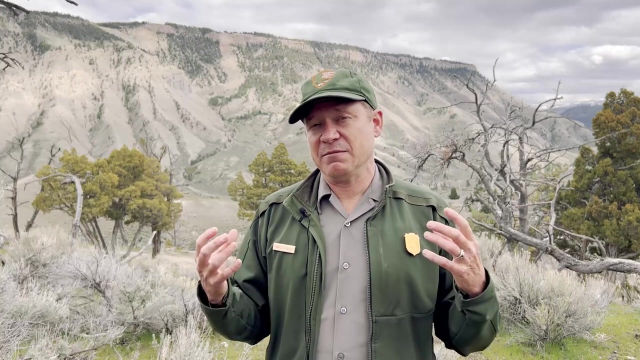 that surround the park, because they move through this gradient of protection to human, more human dominated landscapes. and somewhere in between those gradients is where we are trying to understand that path of the elk and what their long-term success will be, and we have high hopes for that. and again in 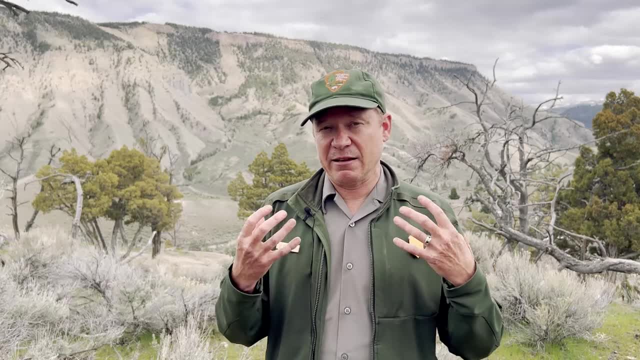 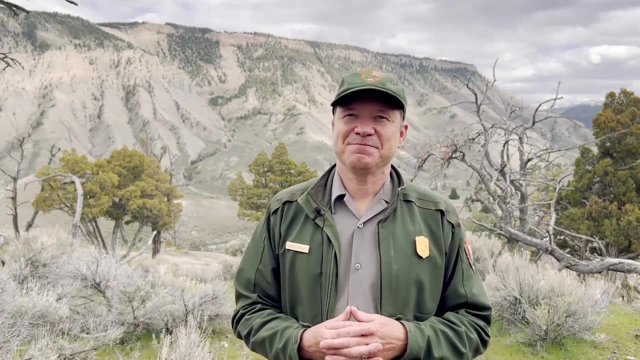 recognizing that, at its core, Yellowstone is going to be that really important preserve for elk in this system. That's a ton of great information Before we sign off. I got a couple questions for you. Yeah, You mentioned, you know all about the life history and the management and everything, but then you 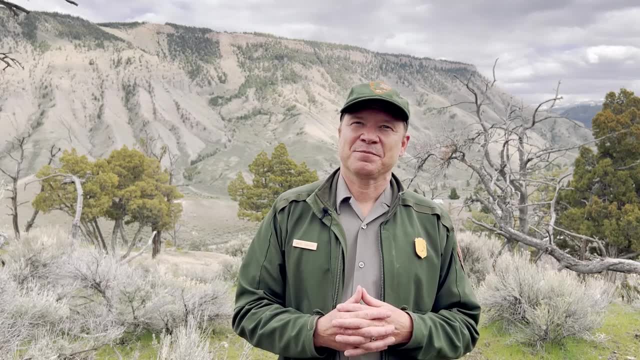 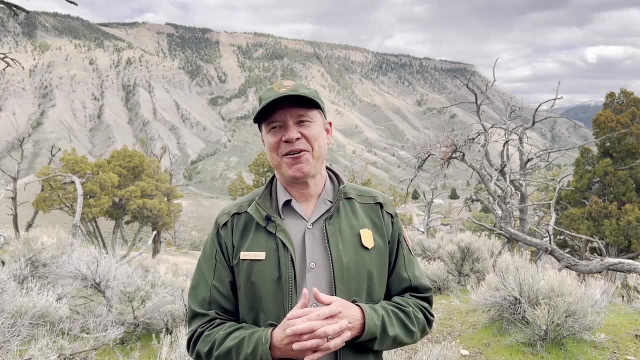 talked about the people who want to come and see elk and earlier in the talk you mentioned a little bit about now we're dropping calves. so as someone who gets to work here in the park and knows where elk hide and things like, if you were to come, what are some tips that you want to give somebody if they're? 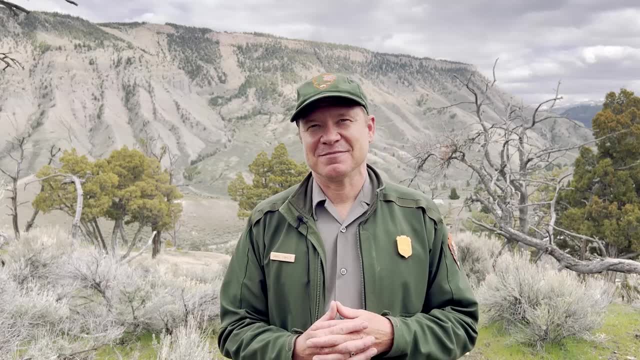 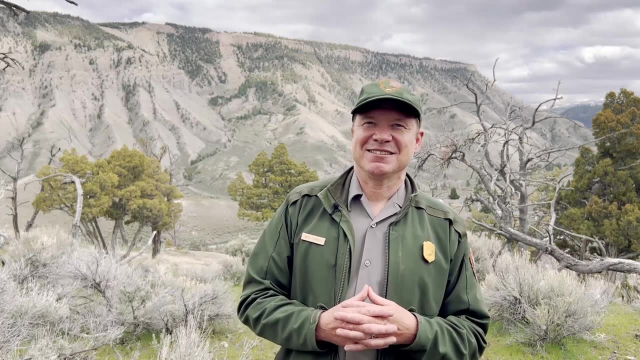 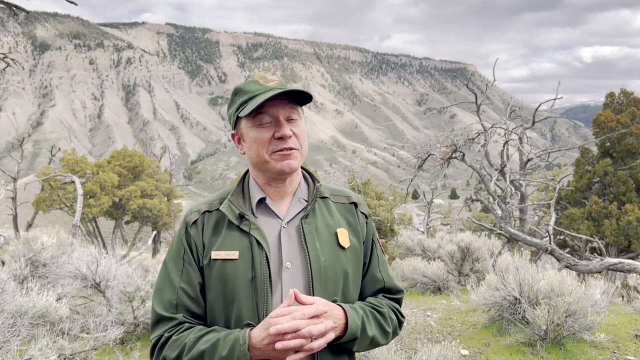 coming to see elk. what? where might they go this time of year? what might they be aware of? you know elk we think of, like you know, bears and wolves- as staying safe distances. but if you could share a little bit about what elk, how to view them safely around here. So you know, I've worked now in Yellowstone for over 25. 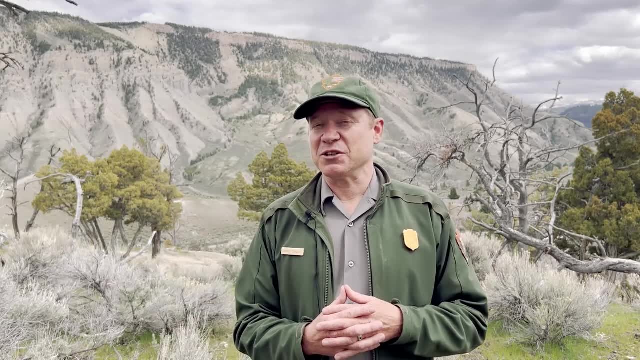 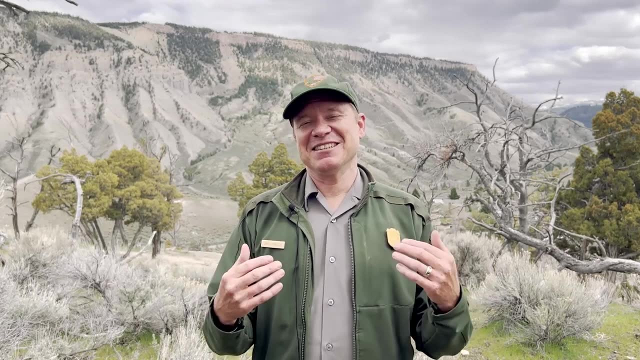 years now, primarily with the predators, wolves and cougars. I've been involved with some bear work, but the elk actually is the animal I think I'm most, particularly this time of the year- cognizant of as a risk out there. so it's really important for the public to be. 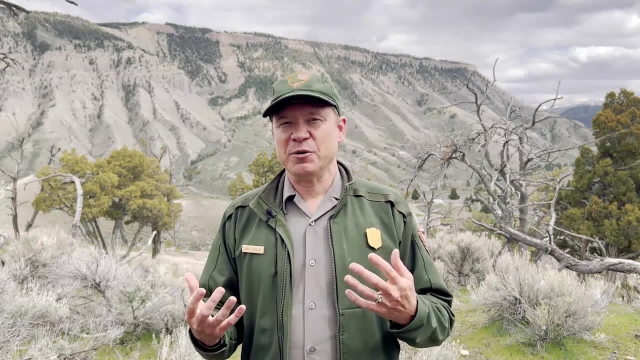 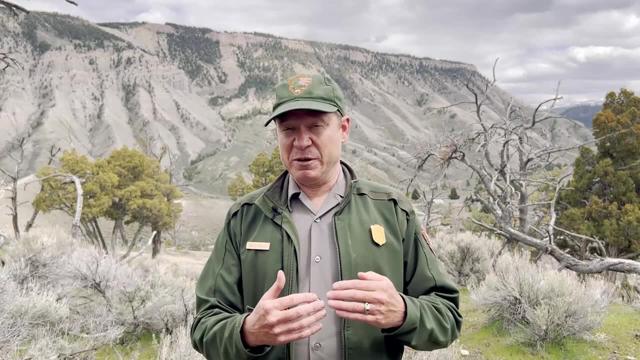 aware of is that, like all wildlife, you want to respect the elk when you see one. the maintaining a proper distance to elk in Yellowstone that would be 25 yards. avoiding, but remembering at certain times of the year you would probably want to be even more careful of getting in and being careful of the animals that you're going to see. 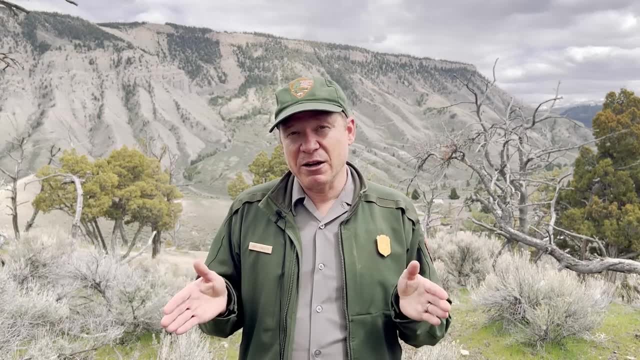 So you want to be careful of the animals that you're going to see. So right now, cow elk are incredibly vigilant and protective over the newborn elk calves and they will charge, they will stomp, they will run at you to protect their calves and to try to discourage you from being around the area. so it's really important for the public to be able to come to a place like Yellowstone and enjoy the beauty of an elk, watch those young elk calves frolic as they get a little bit older but, being very aware of the defensive nature of a mother elk, it's not something you want to mess with. it's the scariest animal in the land. 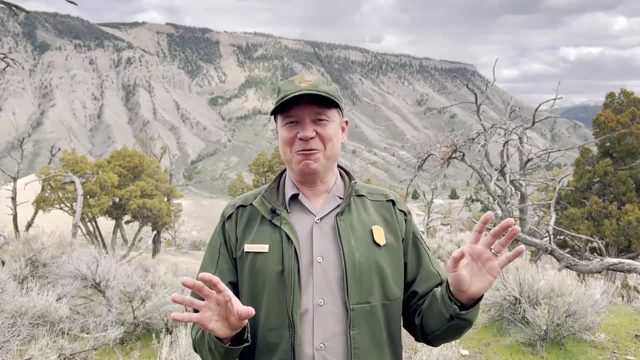 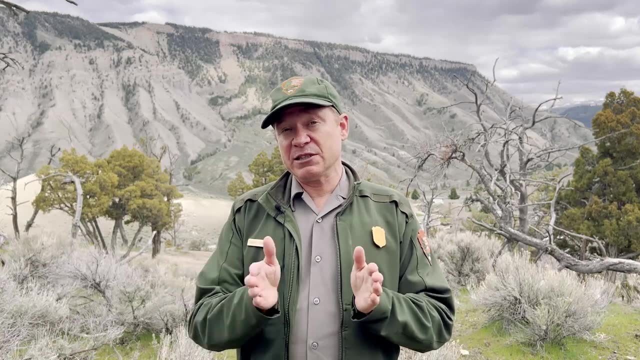 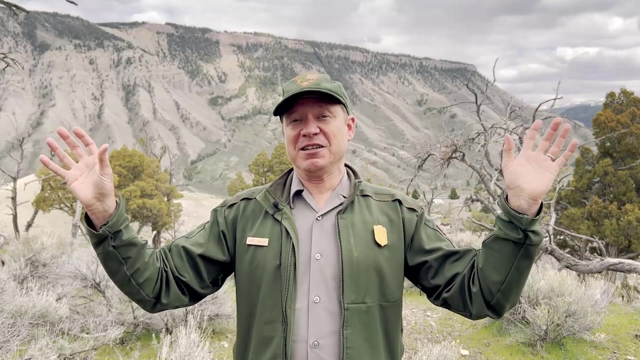 I'd much rather contend with a bear encounter or other animal encounter out there than a lone cow elk on a trail right now. So remembering that equally important is during the fall breeding season, the rut- what we call the rut Mammoth hot springs- is one of the best places in the in the country to come and watch elk. 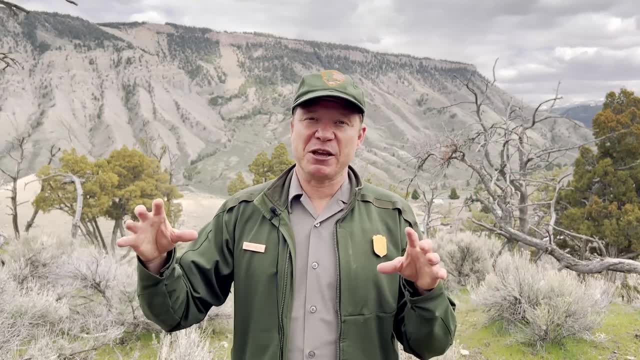 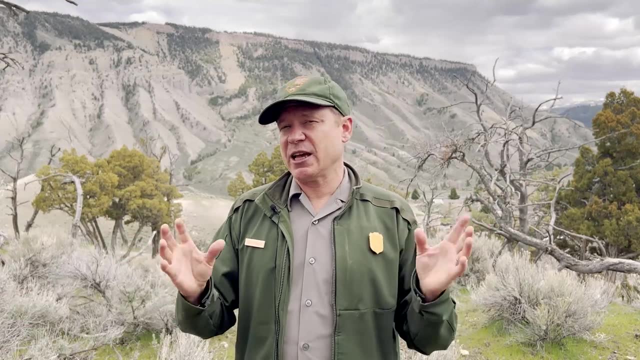 breeding behavior. and those bull elk will come into the mammoth area to try to gather up their harems, or even outside of the developed area. like mammoth, They're bugling, they're roaring, they're changing and charging at you. So remember that. 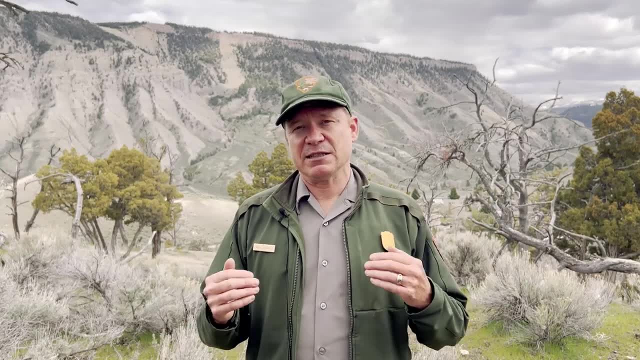 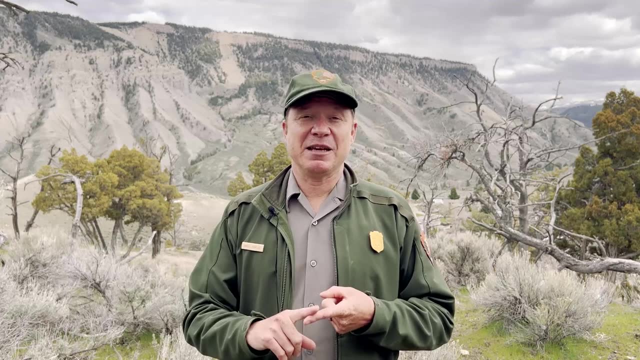 at each other and fighting over those controlling those breeding rights. and a bull. elk can be also a very risky animal. they're super charged with hormones and they will not discriminate between running down a person or charging a vehicle if it's too close to their cows that they're 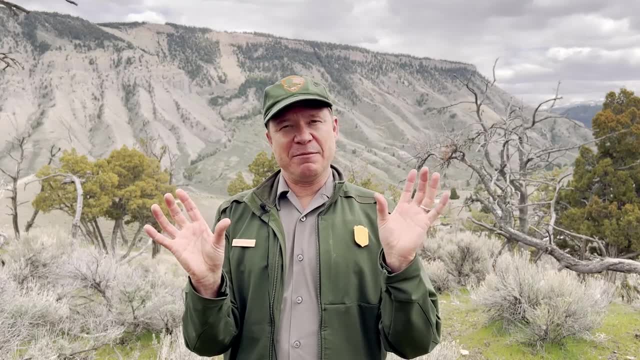 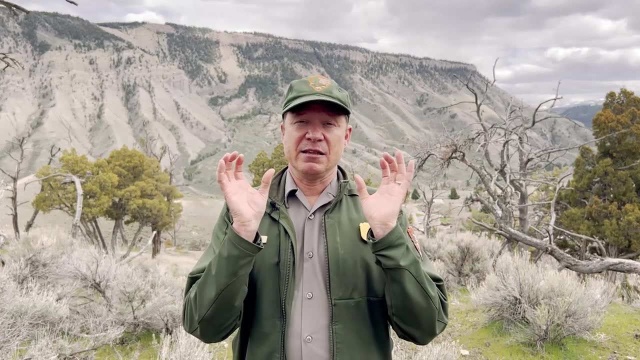 protecting. so those are two key times of the year: the month of may, late may, early june or the month of june in particular, as well as the fall, late september, early october, breeding season. the public should come and enjoy and embrace the beauty of yellowstone elk, but be very respectful of their 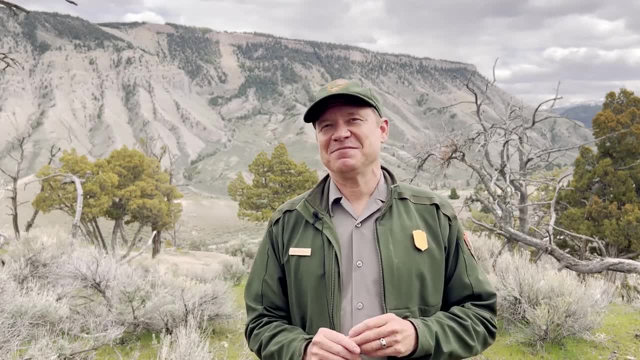 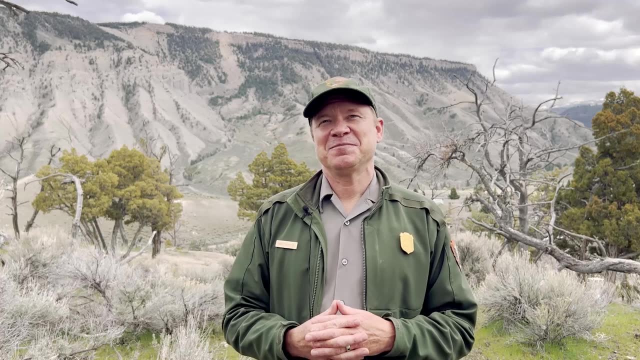 space and of those behaviors those times of the year. yeah, thank you. yeah, and then the last thing we'll see, if you know it's i'll. maybe i'll catch you off guard, but do you have a story about an elk or just like an anecdote or something about why you know why they're such a cool species and 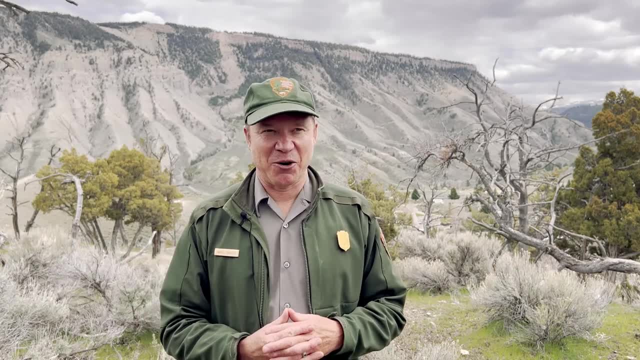 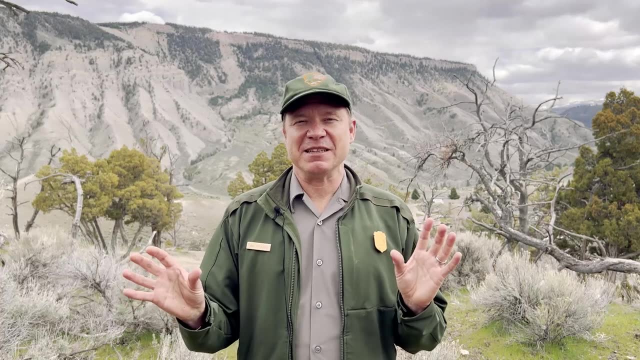 why they're so important to yellowstone, like you personally, yes. so, um, you know, when you study individuals through collaring, you kind of pick up on their patterns. i look at their movement a lot from day to day and where's this elk and what's this elk doing? and you follow them. 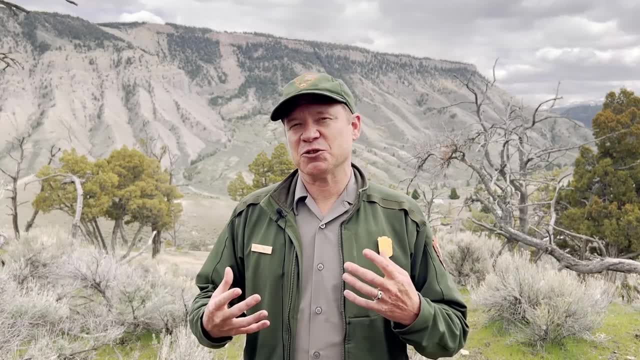 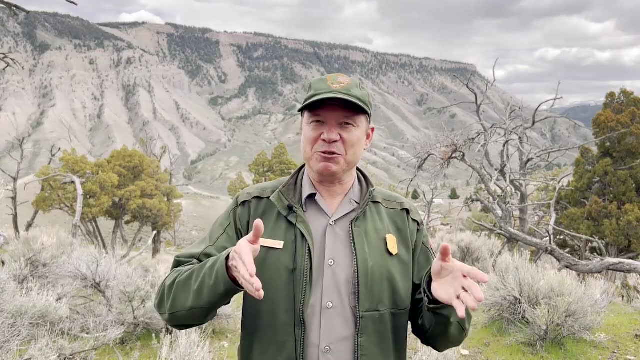 through their lives and you become really interested in their stories. and one story in particular is really fascinating to me: elk 1125. we give them unique numbers and that's part of how we keep track of the data, but elk 1125 was a cow elk that we collared. 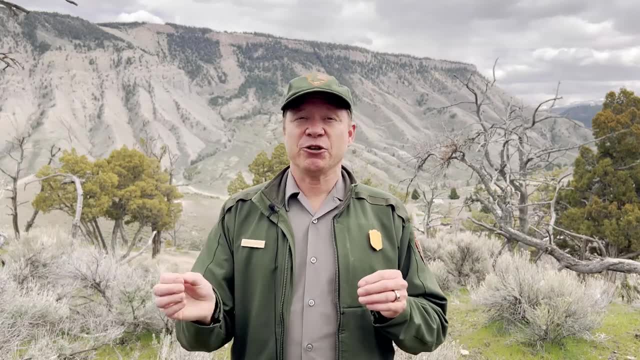 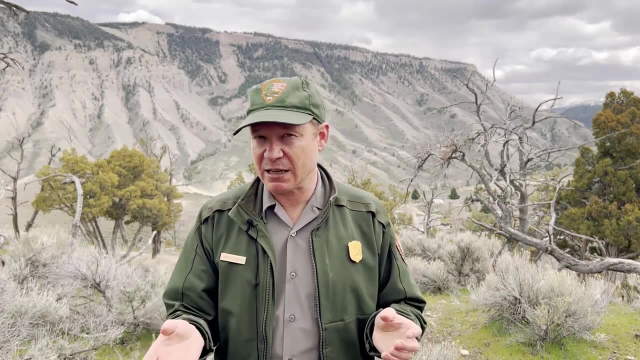 in 2011.. and she was born, we age her. we can pull a tooth from the elk and we can accurately age an animal. we do this with every wolf kill or cougar killed elk. we can pull a tooth from the dead animal. we can submit that to a lab that you can accurately age that animal. 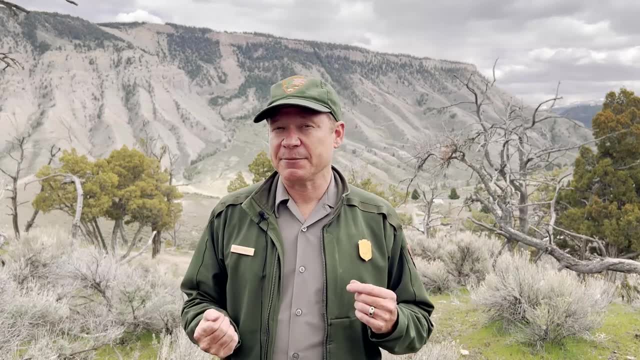 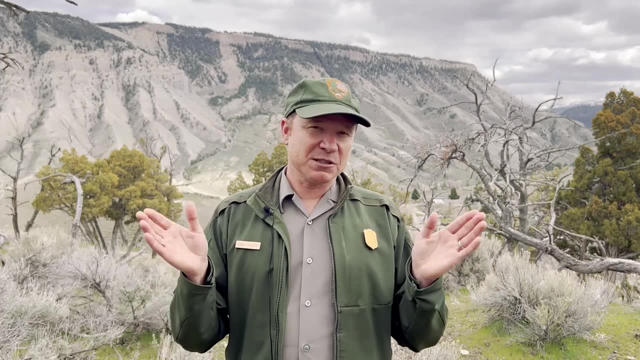 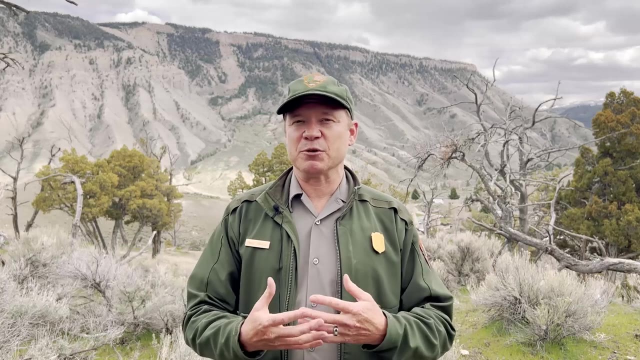 by counting the rings and the teeth through, and so we do that with live captured elk as well, and so elk 1125 was born in the summer of 1994.. this was the year before wolves were reintroduced. this was the year when cougar populations were starting to increase, when grizzly and black bear numbers were high and abundant and this cow elk lived through 25 and a half years of one of the most abundant and concentrated area of carnivores anywhere in the country. and this cow elk was eventually killed by wolves at the ripe age of 25 and a half years old. but here's a cow elk that successfully. 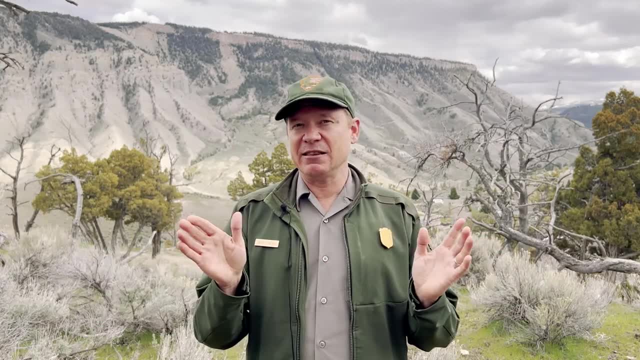 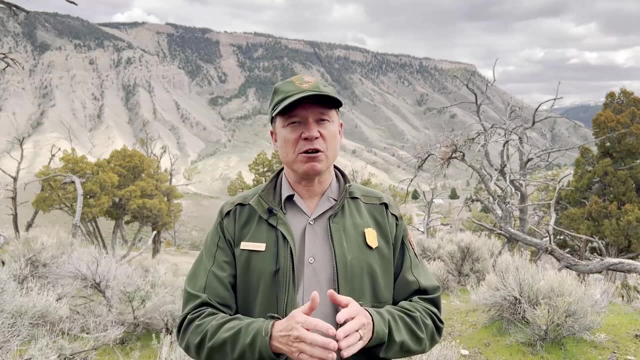 navigated the challenges of yellowstone's landscape, navigated all those years of living amongst carnivores and was successful, was resilient. she probably produced calves every year for the bulk of her life, until she reached her mid-teens, and yet she then went on to live another 10 years. 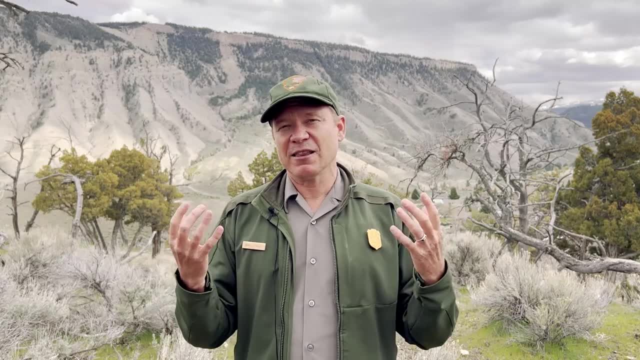 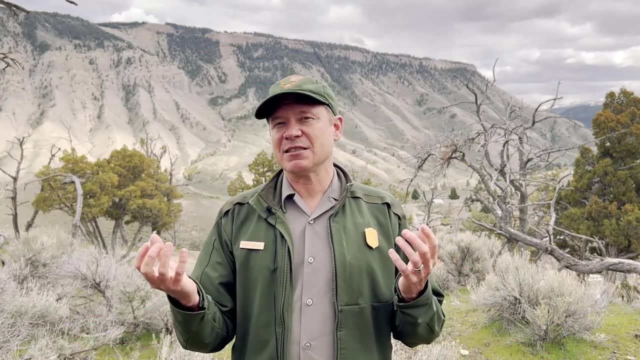 out there. so that just her story- elk 1125- you know who basically was born before wolves came back and died long after they had been established- really represents their resilience, their ability to adapt to a changing environment, and and really represents the spirit and the soul of 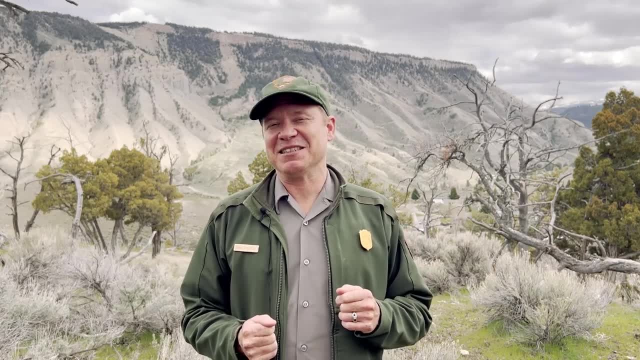 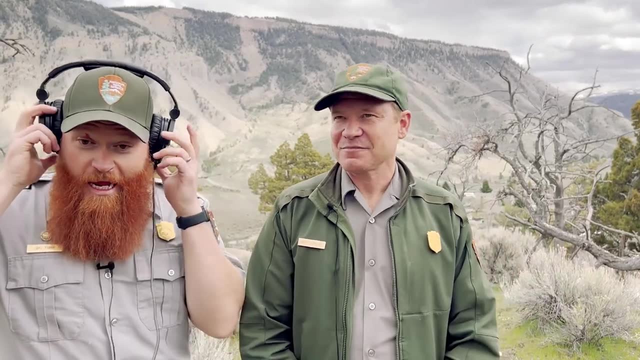 yellowstone's wildlife, so 1125 was a really amazing animal to me. so well, that is awesome. i'm going to jump back over on camera here with you, so i want to take these off. first, i want to thank everyone for joining us, uh for this video. i want to thank dan for 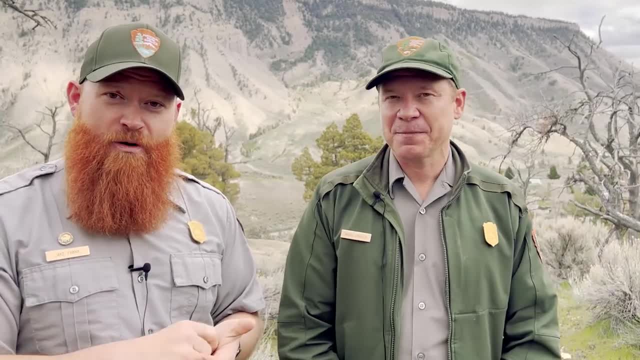 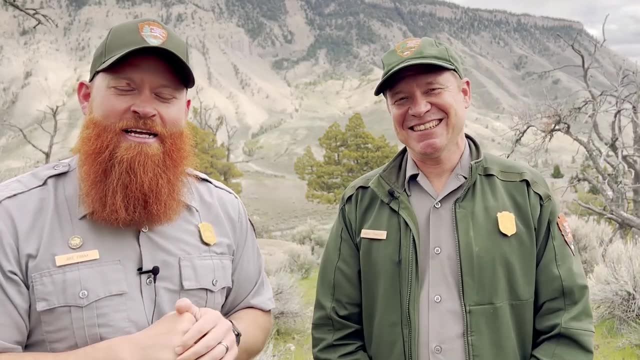 sharing the stories and all of his information. thanks, jake. hopefully you guys had a notebook and a pen and pad he's got like just it's a fire hose of information that come out of there. so it's always fun talking to dan. yeah, um, but thank you again for following along our virtual video. 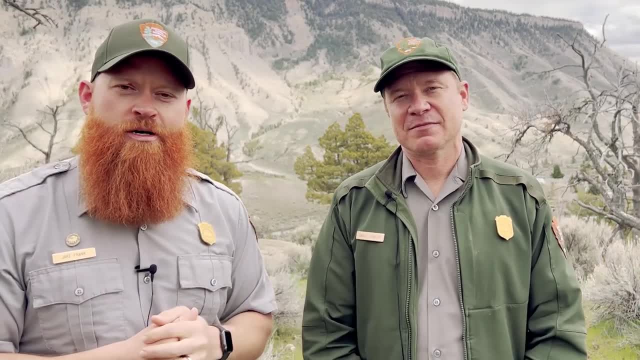 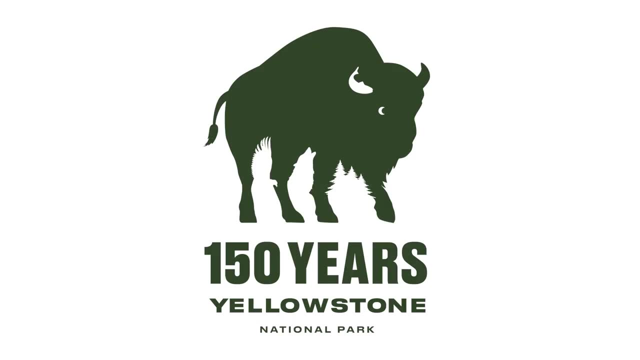 series, our 150th anniversary series that we're doing here. uh, we thank you for your support of yellowstone national park and we'll see you on the next one. thank you, yeah, thanks you.